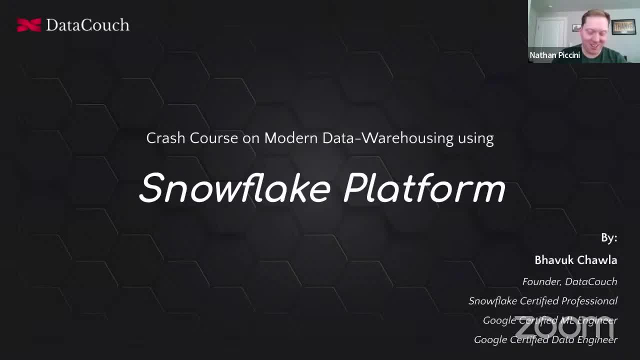 He is an official instructor at the Google Cloud Platform, as well as the founder of Data Cloud, and he's going to be giving us a crash course on modern data warehousing using the Snowflake platform. So, Pavuk, before I hand it over to you, I just want to remind everyone again: if you have questions, please use the Q&A tab, and then we will be giving a certificate of attendance at the end of today's presentation. 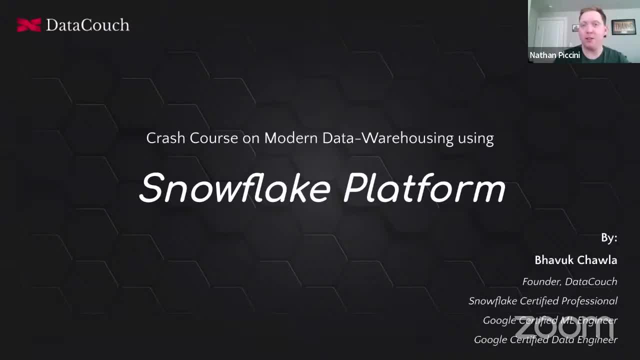 So we'll give you probably around 15 minutes to make sure you get that filled out, make sure you have the link, and then certificates will be sent out before the end of today. Yeah, so, Pavuk, why don't you go ahead and get started and then? yeah, excited to have you. 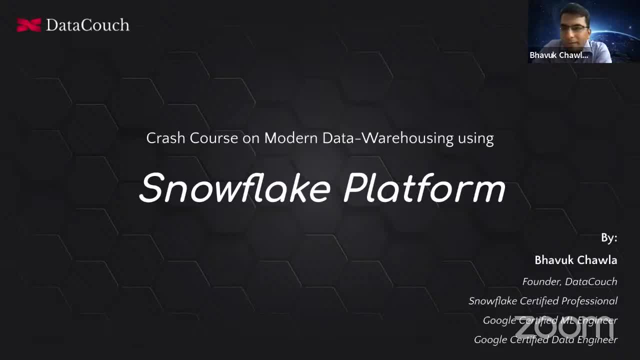 Thank you so much, Nathan. It's my pleasure and honor to have everyone here and I see like people joining from different parts of the globe, So it's very exciting for me today to lead this session and I would try my level best to share this knowledge and ensure that I can make a positive difference in your day-to-day work- day-to-day like learning that you are having every day, so I can take that learning to the next level. 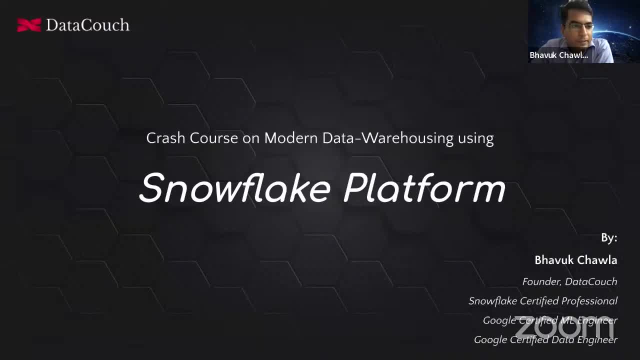 So I am really thankful to you. like you are joining, I know you are very busy, working on multiple things and you have other commitments also. Even then, you have taken out time to attend this webinar on Tuesday, which is a working day. 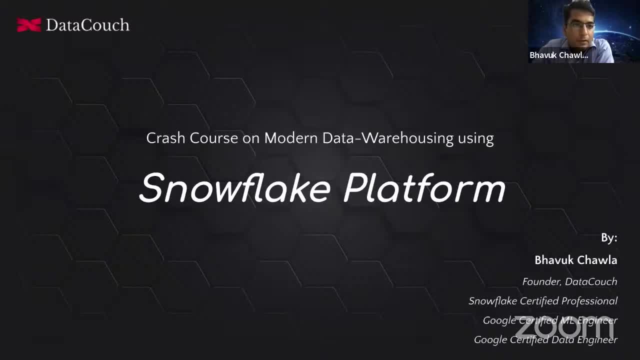 So I appreciate joining like you are joining this session on a working day. So let's get started, and this webinar is on a very interesting technology, which is Snowflake, And it's like next one hour, you will be experiencing a lot of interesting facts and also hands-on around Snowflake. 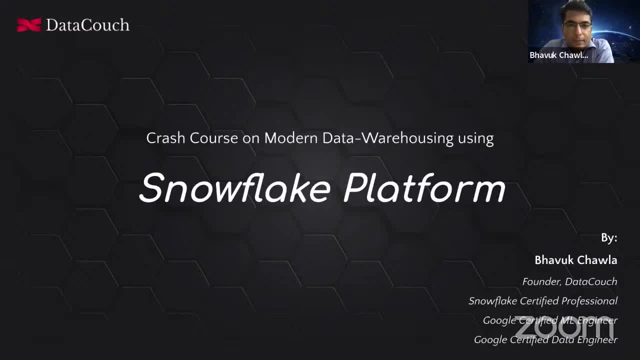 So just stay tuned and ask questions. participate as much as possible to get maximum value out of your participation. So my name is Bhavok Chawla and I am an official instructor for Google Cloud, Snowflake, Confluent and Cloudera. 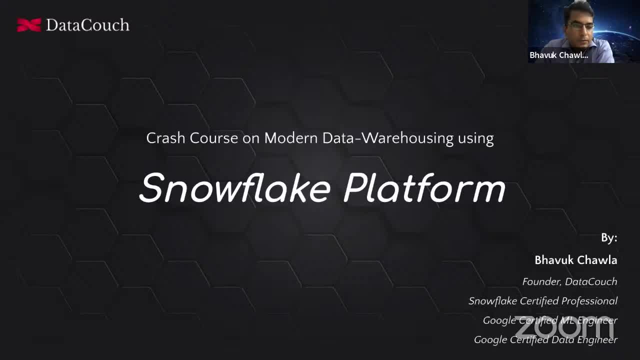 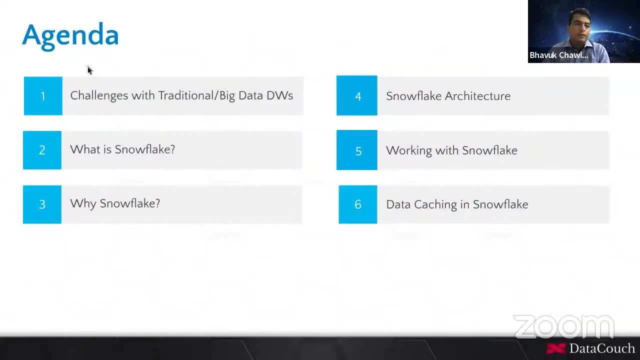 I have a company called Data Couch and we are into this business for last six years now and we have been training professionals worldwide in latest, greatest technologies. So today's session webinar specifically Like we will be discussing various aspects. So one aspect is: what are the challenges with traditional warehouses, data warehouses? 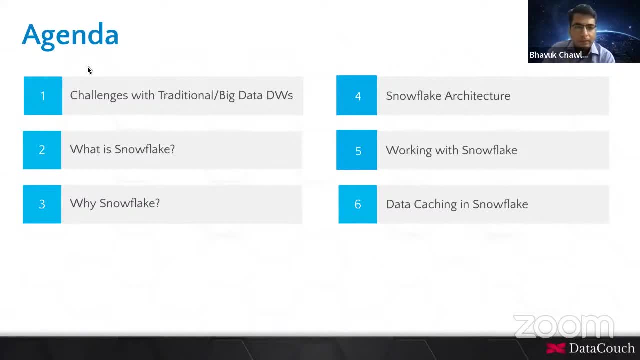 And then we will be looking into what is Snowflake platform and why we use Snowflake platform, And then we will be looking into the architecture of Snowflake and what are the key components within that architecture. I'll be giving you demo on Snowflake platform. 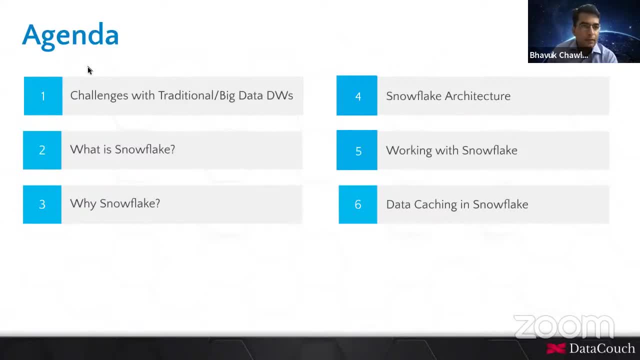 I have a trial account set up so you can also set up your trial account and I can let you know how can. How can you do that? And once you set up a trial account, then how can you navigate through the Snowflake user interface? 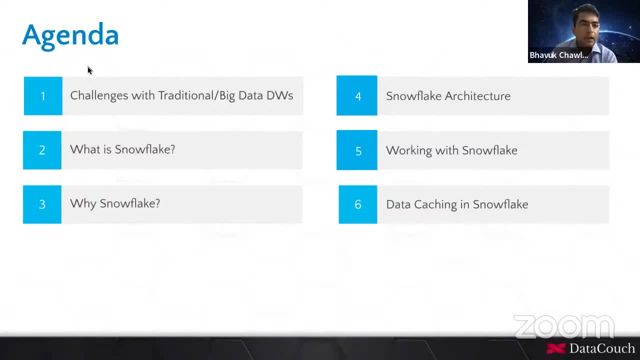 How can you look into the query plan? How can you look into the caching, How can you look into the metadata information schema? So all these things will be covered in next one hour. So that is our agenda. So this is much more detailed introduction about me. 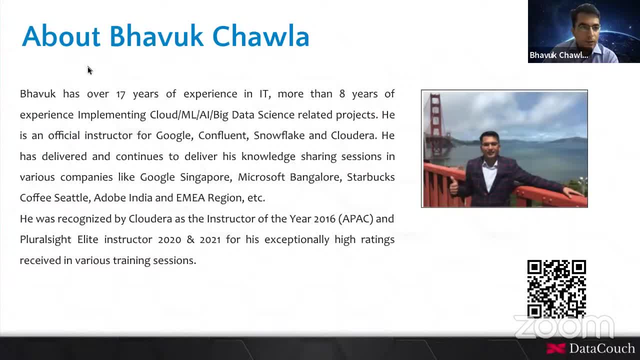 So it will be great if you can connect with me on LinkedIn. So there is a QR code that will be for long-term learning partnership. So I Encourage everyone to connect with me on LinkedIn. in case, like you have any queries, you can reach out to me on LinkedIn also. 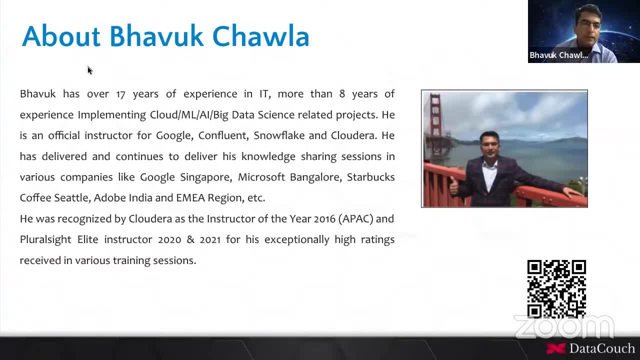 I will be more than happy to answer your questions, even after the webinar. So it's a lifelong partnership, learning partnership. So I have delivered session for many companies, including Google, Singapore, Microsoft, Bangalore, Starbucks Office, Seattle, Adobe, India, EMEA regions. 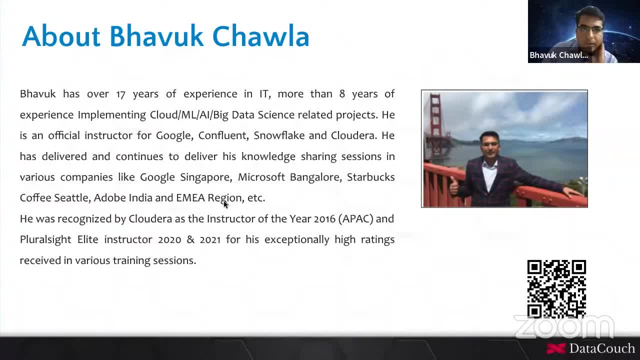 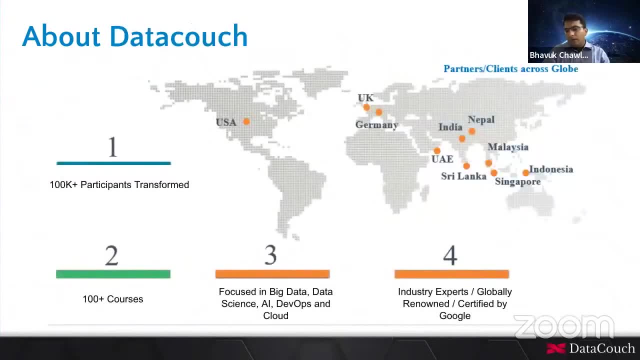 So delivered many sessions across different geographies. Yeah, So different technologies, including data-related technologies, machine learning- So we have transformed more than 1,000, 100K participants across the globe. So this is more into like in-person classes, self-paced courses, as well as the e-learning modules or the virtual instructor-led sessions. 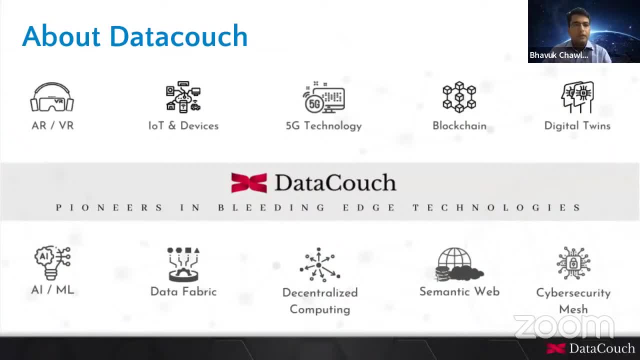 So we are into Web 3.0 technologies and we are ensuring that we are always dealing with cutting-edge technologies and transforming professionals in Fortune 500 companies. So this is our goal. So these are some. So these are some of the sessions that we have conducted across the globe. 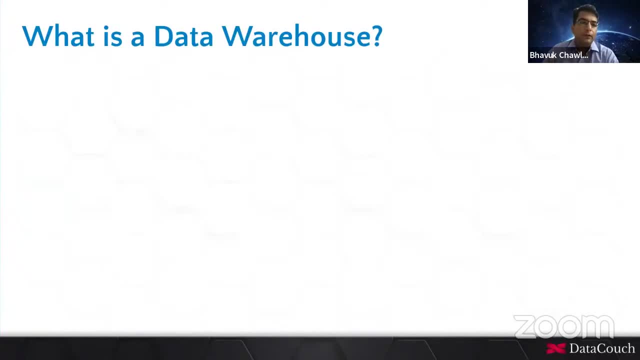 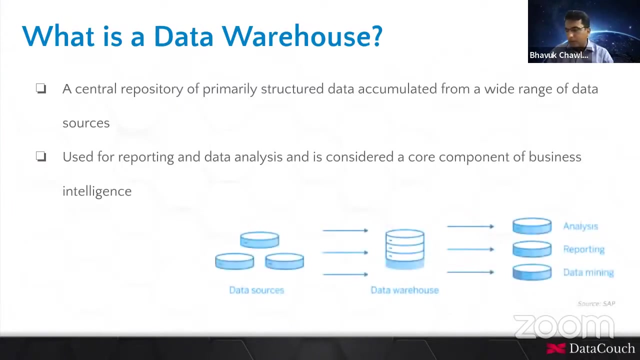 So very first question is: what is a data warehouse? Before we go into the detailed hands-on on Snowflake, first of all, what is a data warehouse? So a data warehouse is basically a central repository, And here you will see that we are able to get data from different sources. 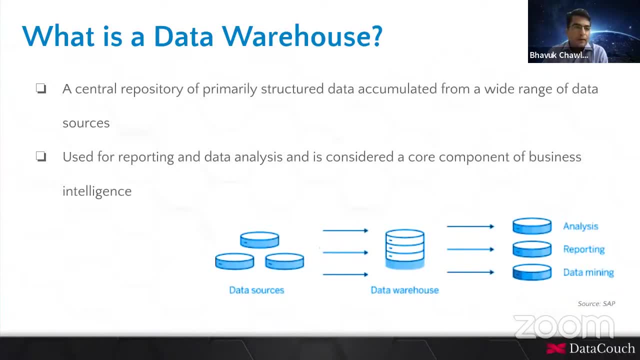 So these data sources can be your operational data sources, transactional data sources like data marts. So you are bringing data from different, different data sources And bringing it into data warehouse, And we are talking about primarily structured data here. 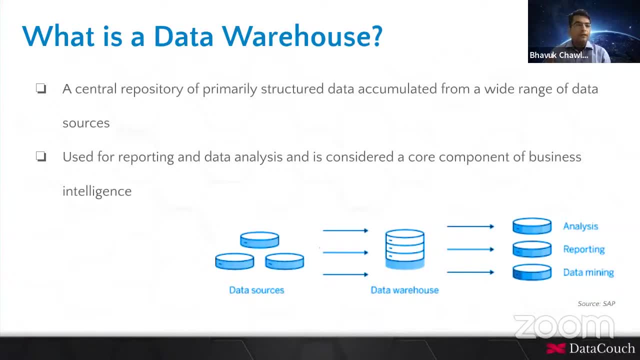 So when we say data is accumulated from different sources, then this data is made useful for your business intelligence reporting, or you want to do some analysis on top of that data, or you can use that data for your machine learning algorithm. So you are making that data available in a structured way at a central place that is our data warehouse. 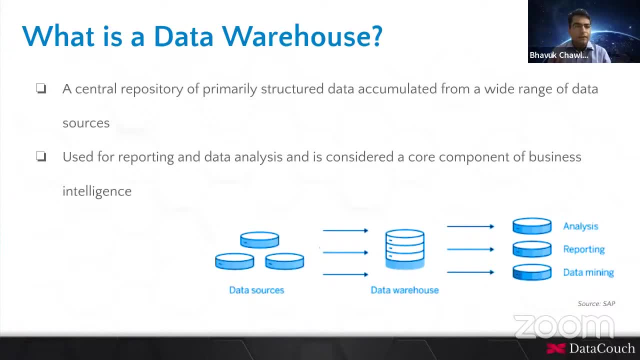 So this is a very quick background about data warehouse. What exactly is data warehouse Before we delve deeper into Snowflake platform? So if you have any queries, questions, you can always bring it on the chat. I will be more than happy to answer those questions. 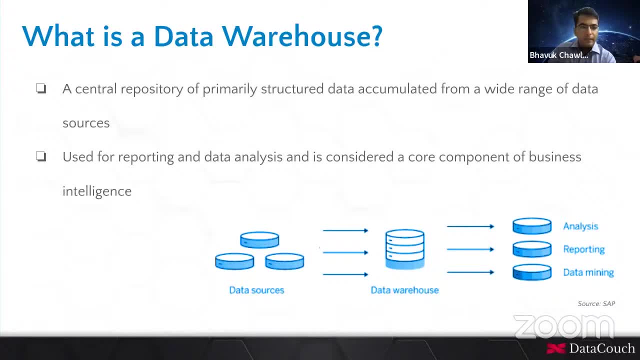 But before we move on, it will be great if you can, if you have any queries, if you have anything in your mind, you can go ahead and ask. So I'll just take pauses in between to ensure that your questions are getting answered also along with the session. 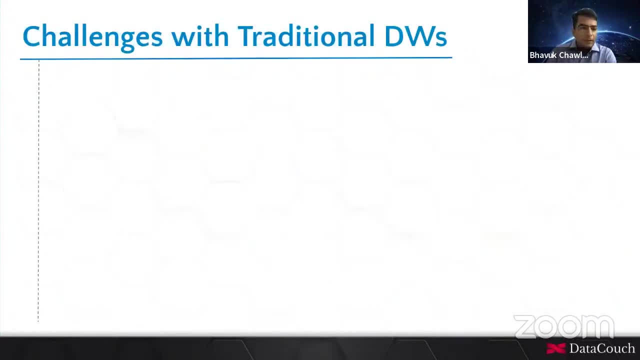 Yeah, So I see there are no questions, So I'll move to the next topic, which is challenges around traditional data warehouses. So I'm not sure if you work with traditional data warehouses. I have a working experience working with different data warehouses, including Hive, specifically. 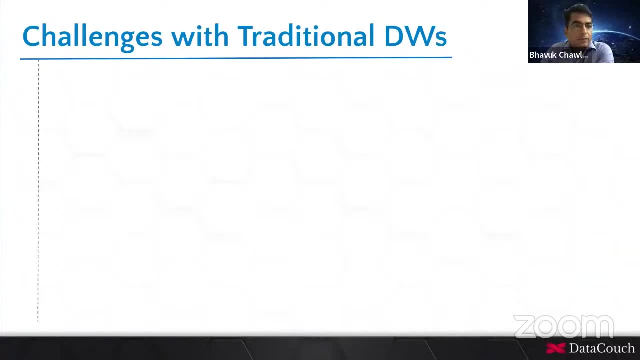 Like I worked a lot with Hive And then there are other data warehouses. I work with BigQuery also, I work with other data warehouses, So those are Like BigQuery is not traditional, but in general I work with Hive and many other traditional Oracle warehouse as well as now cloud-based data warehouses. 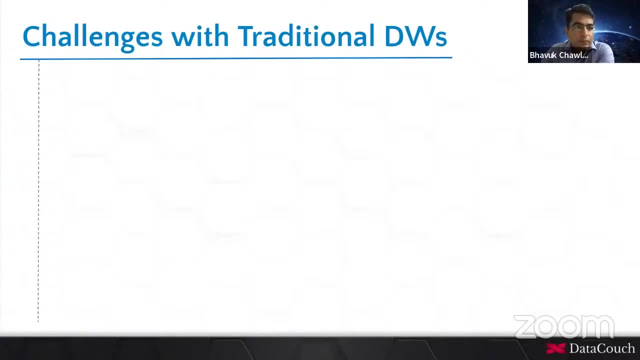 So I'll be sharing some of the differences and experiences working with those. Okay, great, So you know, like database is a general term. As such, like you will find on a very high level, there are two types of databases. 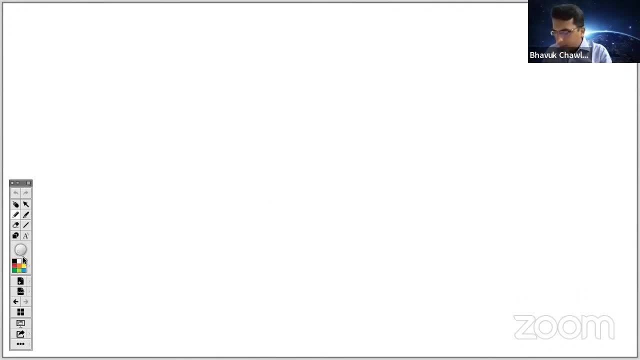 So you can see this is I'm using a whiteboard so that it is clear. So in general, you'll find there are relational, let's say, databases. You must have heard about those And if you see there is one, 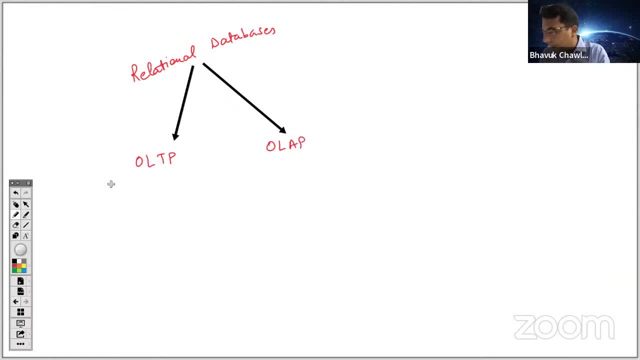 There is one thing called OLTP And another thing is called OLAP, So this is online transactional processing. This is online transactional processing. So this part is like: when transactions are happening on the website, then those transactions are going into this OLTP. 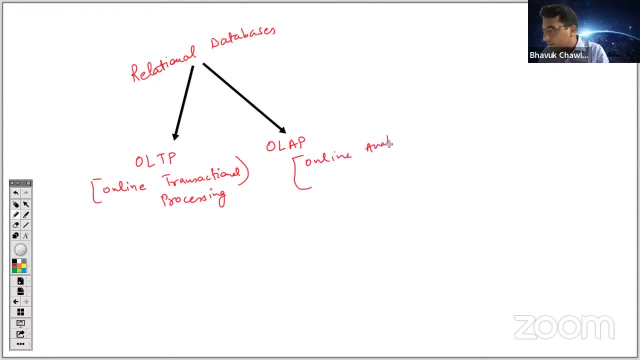 OLAP is online analytical processing, Analytical processing. So this part Like is basically for historical analysis, right, So you are using it for reporting? right, So you can have business intelligence tool connected with the OLAP. 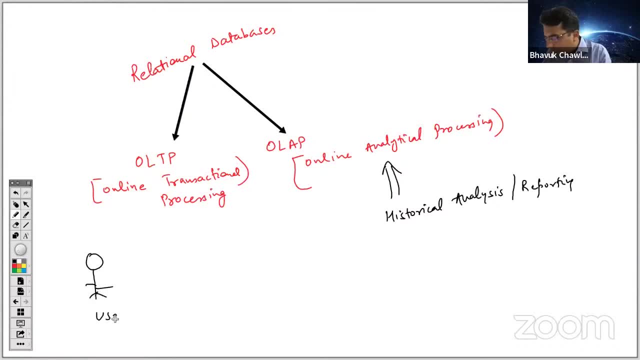 So how the process works. Let's say this is a user And this user is placing an order. Let's say this is a website- Amazon. Let's say there is e-commerce website And on e-commerce website there is order getting placed. 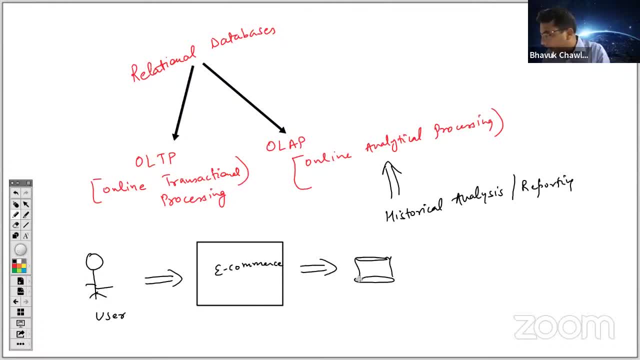 And then Then this goes into OLTP database. This is OLTP database, And then this is like a process which is running And this is moving data into OLAP, And then business intelligence tool is connected to the OLAP. 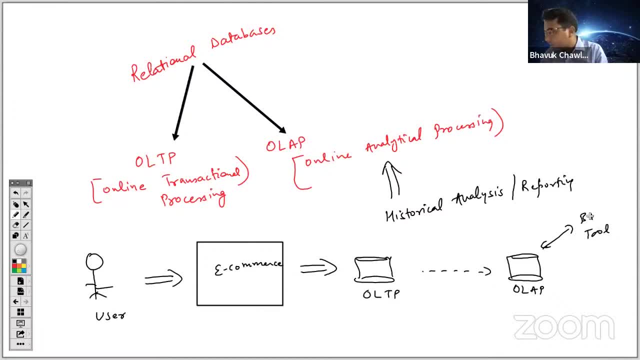 And we can fire ad hoc queries through business intelligence tools. So this can be Like here: we will get the dashboards, So you can have dashboards And on that dashboards you can see like various insights. 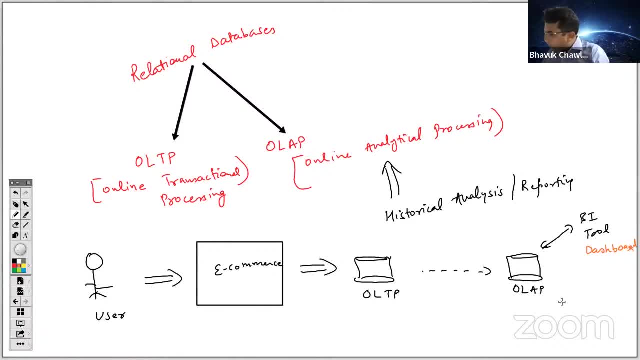 Like you can take. You can take decisions Like these are for business users. So business intelligence is business users. So this is how the overall holistic picture is Like. I hope you got it, Sam, that there is a relationship between OLTP and OLAP. 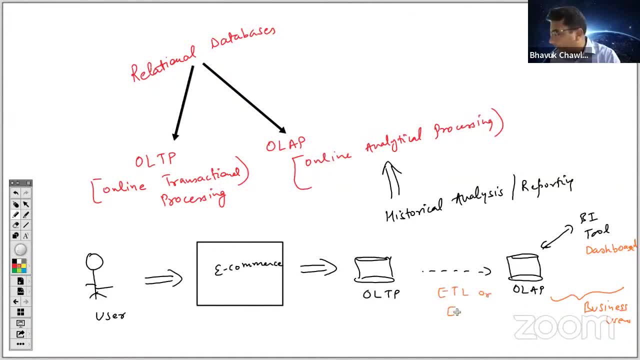 And there is a process. Maybe you are doing ETL or you are doing ELT, So extract, transform and load. You are moving data from OLTP to OLAP so that you can fire queries. Yeah, So I will explain this more. 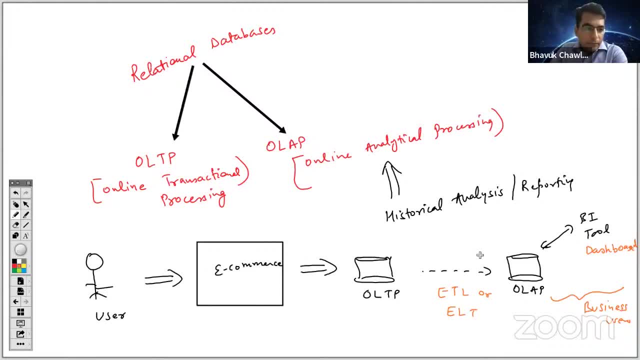 But this is a quick Answer to your question. like databases, There are two types of relational databases. Specifically, I talked about OLTP and OLAP, So we are talking about data warehouses, which is here, So we are talking about data warehouse. 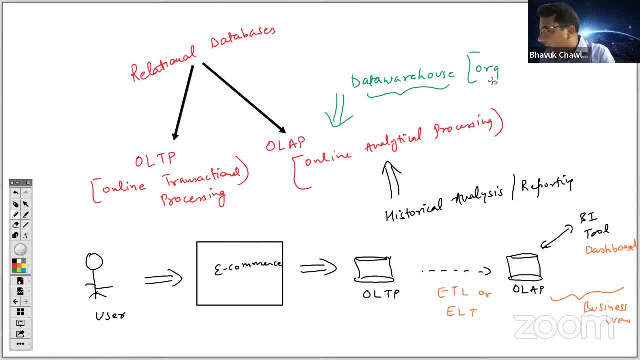 And data warehouse is basically organizing your data in a manner so that reporting is easy. Yeah, So we are organizing data in a manner so that we can fire queries and we can get the results. So we are talking about this portion right now. 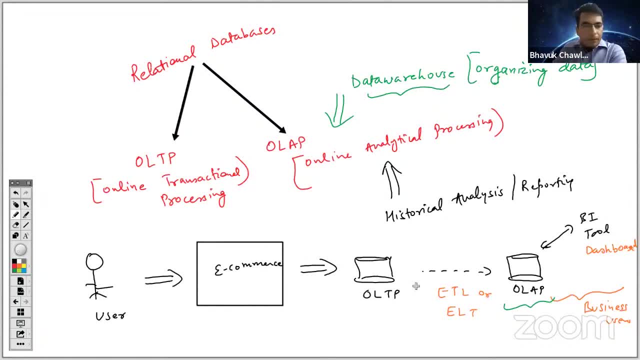 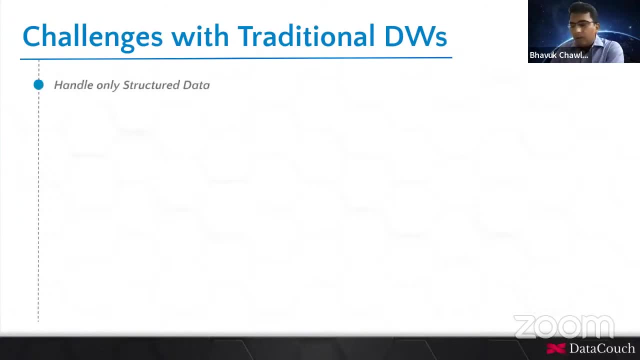 So data warehouse OLAPs That we are having, Okay. So now coming back to this, So there are many challenges with traditional data warehouses. So one thing is they handle only structured data. Second thing is performance of data. like performance for large data set is usually low or slow. 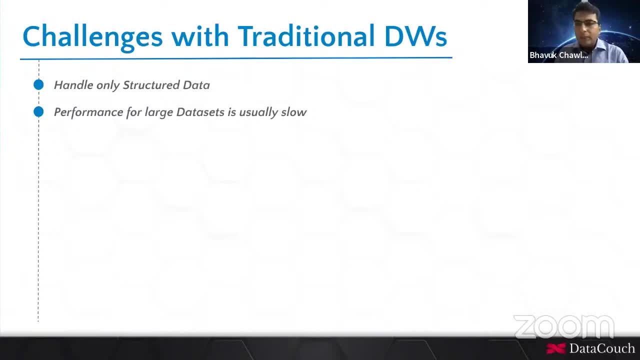 It's very slow, Like it takes maybe three hours to run a query, But if you are using Snowflake then you can fire that query and you can achieve the results maybe in less than three minutes. So these are some of the case studies you will find. 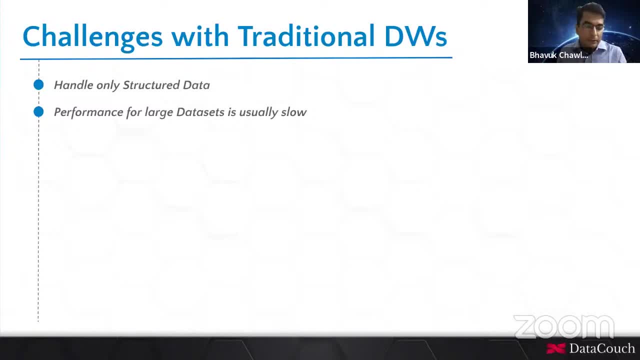 And even my personal experience working in different projects, I have experienced Snowflake is much more like better in terms of giving the performance of the query is very fast and the latency is very low. So the storage perspective in traditional data warehouses storage is not infinite. 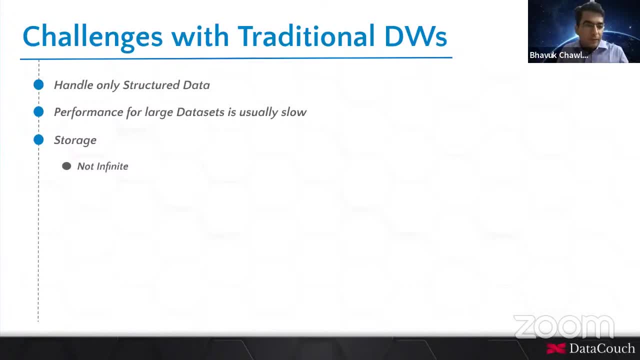 But we are talking about Snowflake, in which, you will see, we are making use of cloud-based data warehouse where we have almost infinite storage available to us. It's not scalable, It's not elastic. So, traditional data warehouses, you will find they are having a lot of limitations. 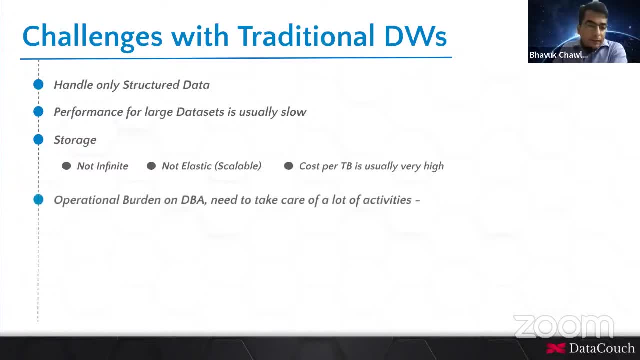 The cost per terabyte is usually very high. Operational button is very like. it's very much on the DBA database administrators You will find, like database administrators they have sleepless nights fixing issues in the data warehouses, traditional data warehouses. 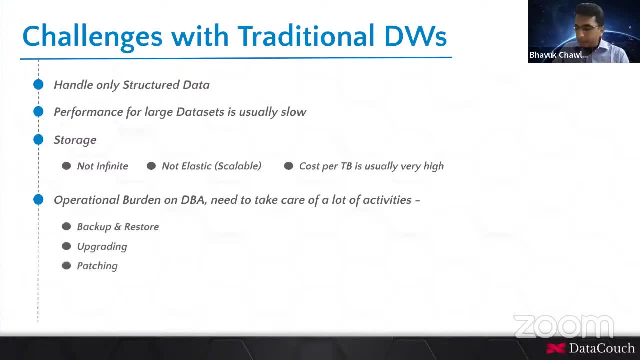 So there are a lot of things that they need to take care, like backup and restore, upgrading, patching, capacity planning, multi-tenancy, indexing. So there are So many things that database administrators they have to see or they have to take care in a traditional data warehouse. 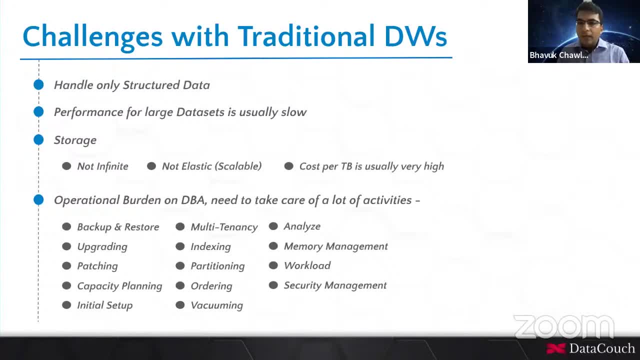 But when we talk about Snowflake, we are basically ensuring that we are not going in that direction. We are making use of data warehouse as a service, So it's like data warehouse as a service. So it's like cloud-based data warehouse, modern data warehouse, which is overcoming all the problems that we were having in the traditional data warehouses. 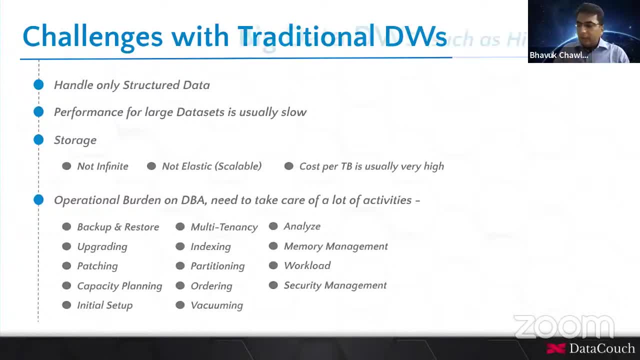 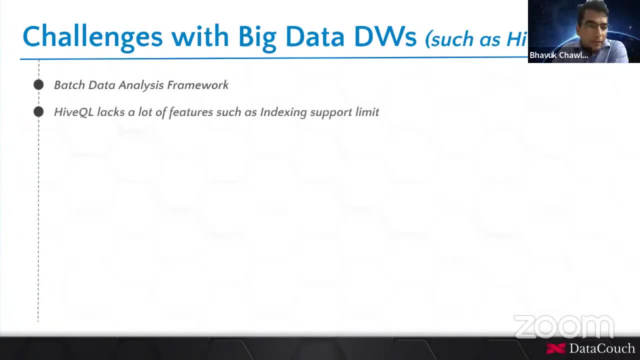 So, after traditional data warehouses, there were other types of data warehouses which were called big data warehouses. so these big data warehouses, for example, hive. so this particular warehouse was created in facebook and it was in 2008 when it was created, and it was created on top of hadoop. 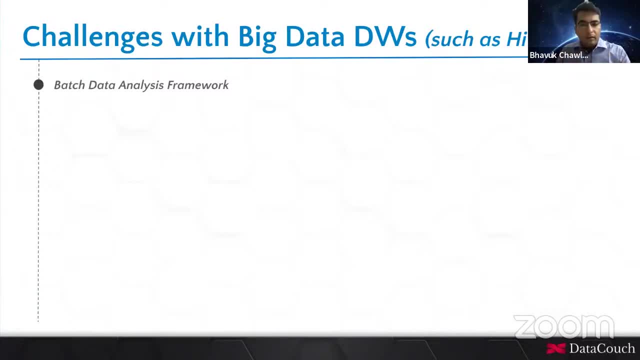 environment, so hdfs, and you can even run queries on hbase when you are using hive. so this is primarily batch. yeah, it's not for streaming data ingestion or streaming analysis, so you cannot do that through this data warehouse, like hive data warehouse, and it is built on top of hadoop, so 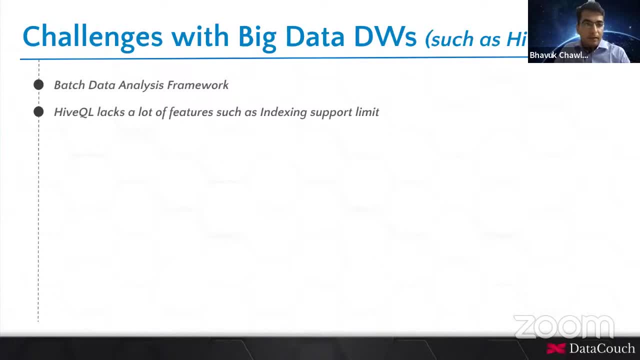 there are certain fundamental assumptions and there are limitations of hadoop and hive actually inheriting those limitations because in hdfs you cannot update data. so hive also struggles a lot when it comes to updates, even though it provides your syntax to update data. but there is a lot of. 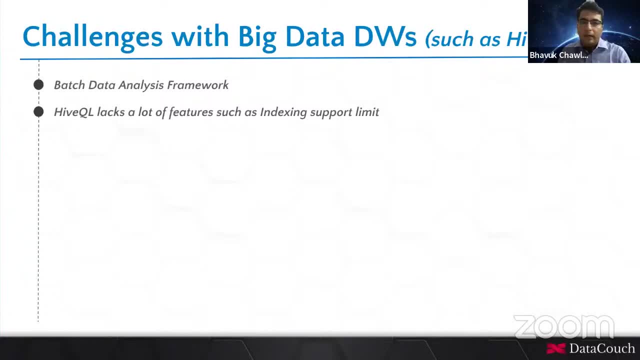 going, a lot of things going on under the hood. that means compaction going on and a lot of like delta and then full, full, like we loaded the data and then we there is a delta record, and then delta, delta directly being maintained, and then how the data is being merged. so it's very complicated process under the hood. 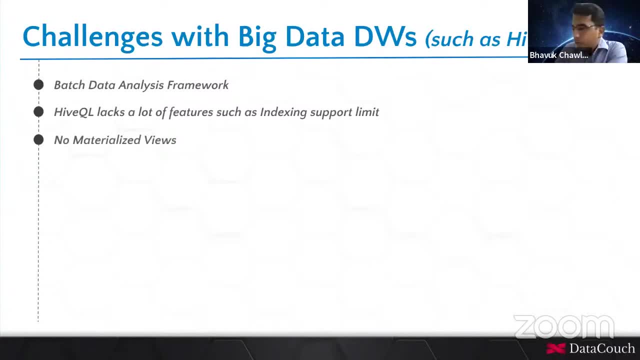 so hive ql, hive query language is lacking. support for a lot of features, including like indexing support, is very limited. materialized views are not there. stored procedure support is not there, and then updating data is really painful. in hive, rdbms is also like we are having rdbms behind the 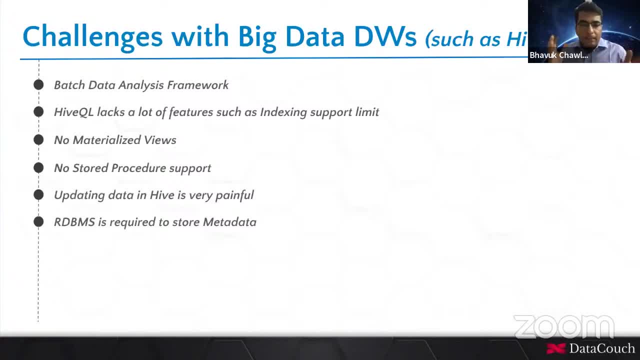 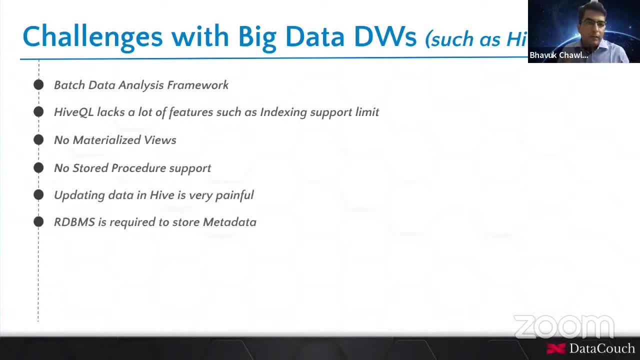 is ensuring that we are having metadata in hive. so keeping data and metadata in sync is in hive is really problematic. it's not easy, it's very painful. so you will experience like issues. you will get exceptions that the metadata is not in sync with data, so you have to repair table in hoop. so a lot. 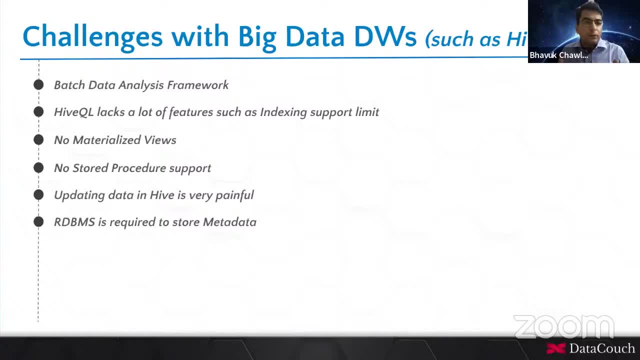 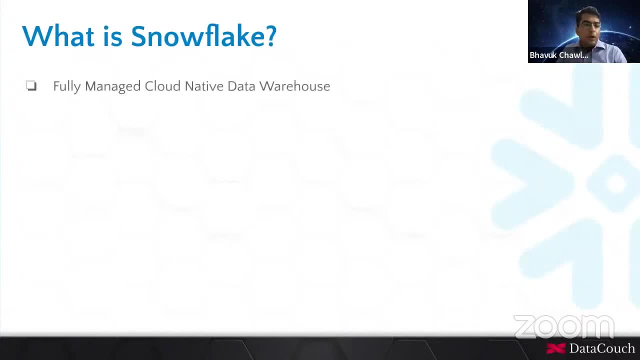 of challenges are there traditional data warehouses and including big data warehouses, because big data warehouses also, they are having some fundamental assumptions. now, what is snowflake? snowflake is an Snowflake is fully managed cloud native data warehouse. Yeah, so fully managed. that means we are talking about data warehousing a service. 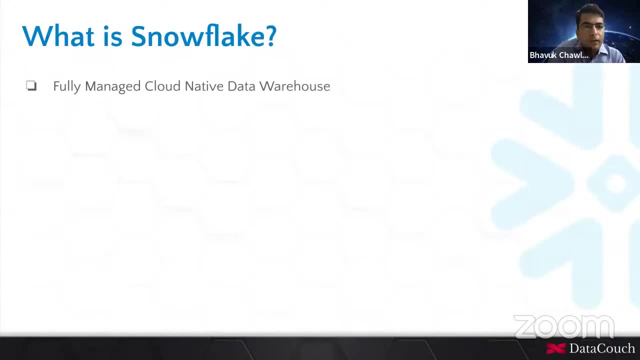 So one option is you buy a car. Second option is you rent a car. Third option is you take an Uber. So when you buy a car, you are investing so much You have upfront cost of buying hardware. So when you are buying- let's say when we are buying a car, it's like you are owning. 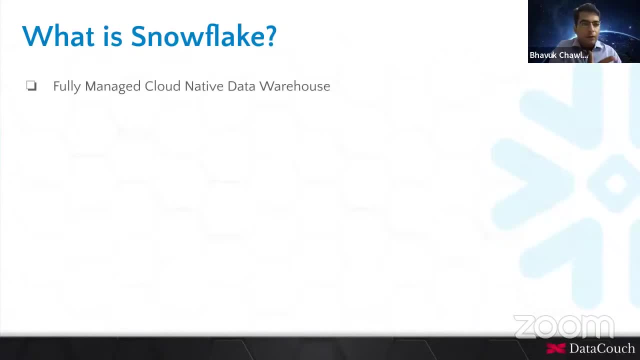 your own data center. When you are owning your own data center, your own data warehouse, you are like spending a lot of money to buy that hardware, to buy the car, And you have to get a lot of approvals. Yeah, so then only you can buy. 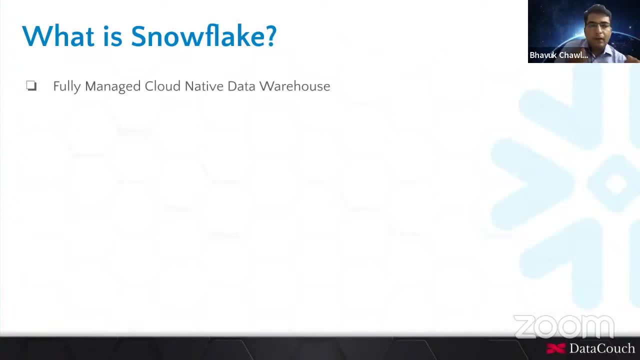 And then you are investing a lot on the licensing and everything, And then after that there is a cost involved per terabyte and licensing models can change based on the data warehouse that you are choosing. So what I want to communicate here is: we are not into buying a car because we don't want. 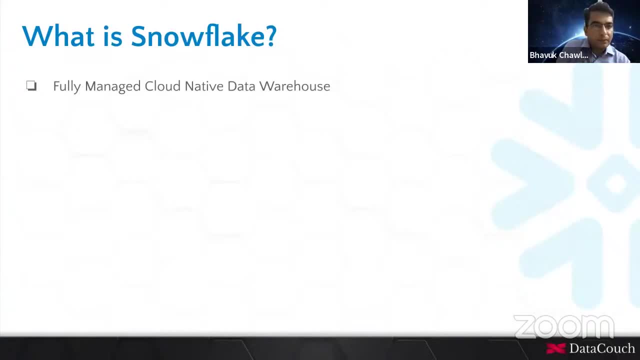 to pay upfront. We are not asking you to buy million dollar machines, So we are saying that maybe go for rental Based model or go for Uber. That means you pay for the trips that you are making right, Rather than paying for the entire like the car. 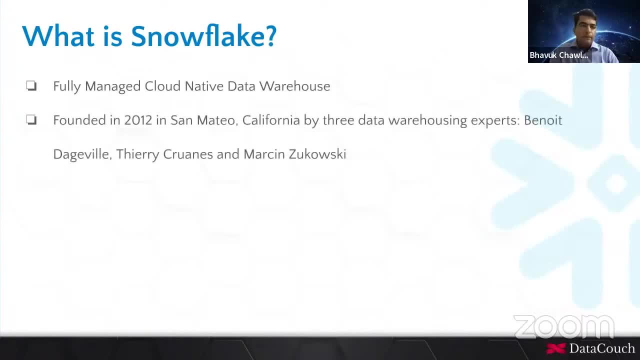 So that's the idea here. So we are on cloud and it is something which is very much elastic, So it is highly scalable. I will talk about the benefits of using Snowflake in more detail, but I'm just sharing with you that it is fully managed and cloud native data warehouse. 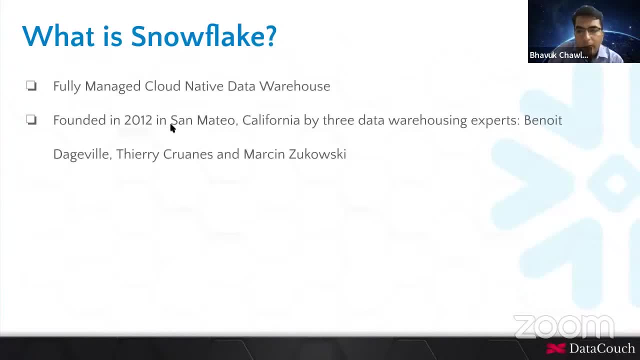 So it started in 2012 in San Mateo, California, by three data warehousing experts. So these are the three people who started Snowflake. And please understand, Snowflake is not something related to Snowflake schema. Yeah, it is. It is something like two founders out of these three founders. they loved skiing or winter. 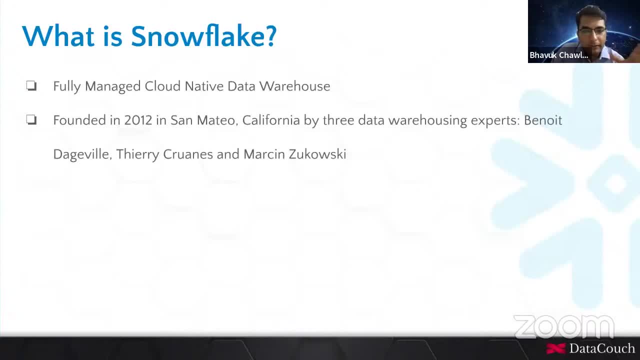 sports, So that's how the name Snowflake- So it's coming from there. It's not like any data model or Snowflake schema. specifically because a lot of people are confused, like because there is a term Snowflake schema in data modeling but we are not. 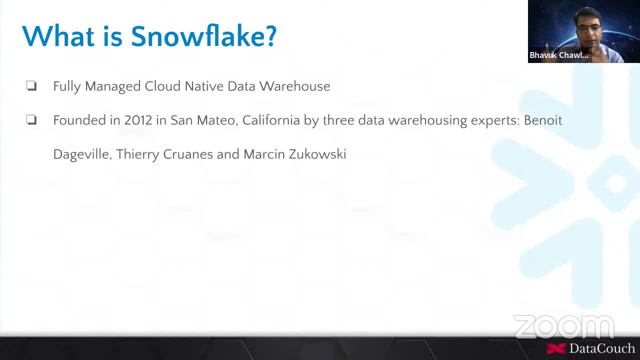 talking about that. We are talking about Snowflake. Like it's a. like they were, they were fond of skiing and winter, So that's why the name is Snowflake and it started in 2012.. And after that, in 2014,, initial customers started to onboard into Snowflake 2015,. it 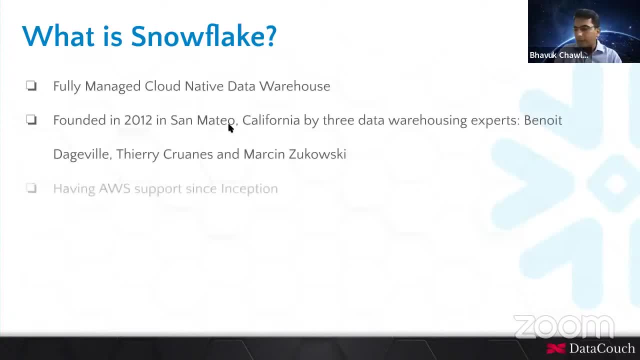 became generally available on AWS platform And later on it started to support Azure cloud as well as GCP, So it can run on three main cloud providers. So it's cloud agnostic. You can run it on AWS, You can run it on Azure. 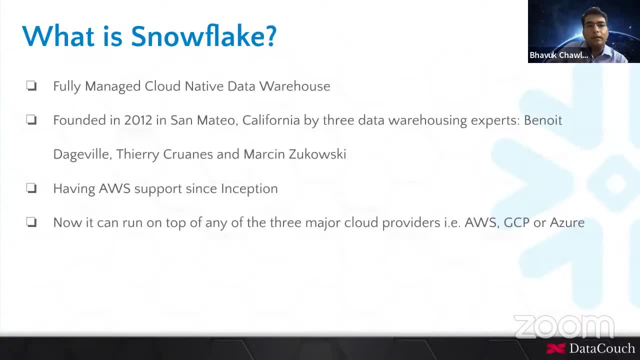 You can run it. You can run it on GCP, So you can run Snowflake on all three cloud provider- different, different cloud provider. You can choose which one you want to go for. So a lot of times many companies they set up Snowflake like maybe you are having AWS as. 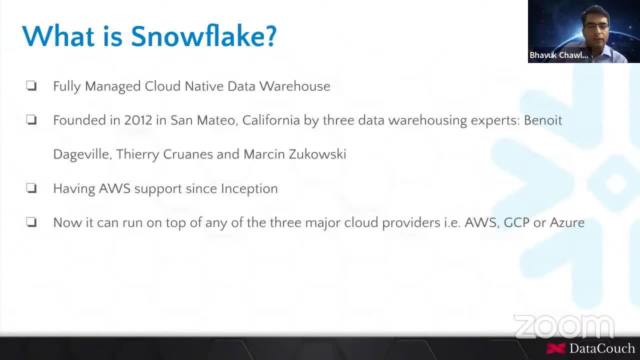 your primary cloud provider and then you have DR strategy and then you have Snowflake also running in some other region, in maybe GCP or Azure, So you may set up Snowflake like that, but in general Snowflake supports three main cloud providers that we have public cloud providers. 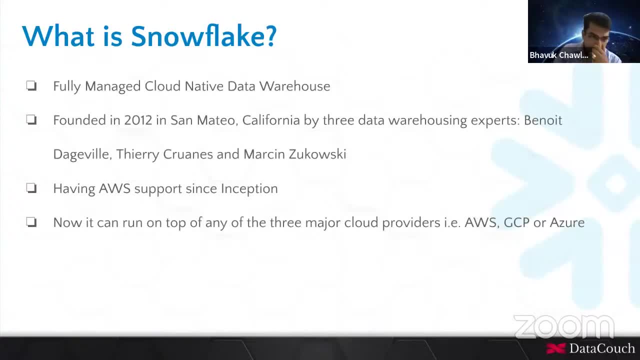 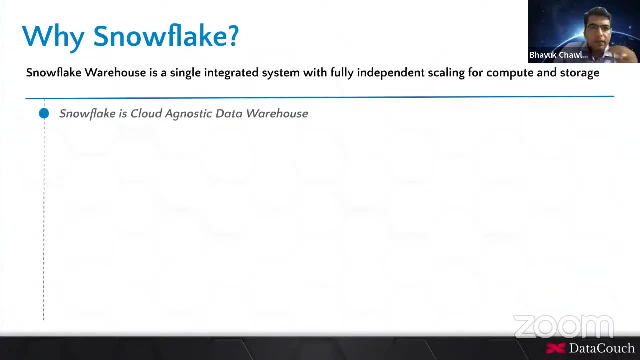 So this is AWS, GCP and Azure. So why Snowflake? So very first question is why we are even talking about Snowflake. Very first thing is like it is cloud agnostic. So if you go for any specific data warehouse provided by a cloud provider, then you will. 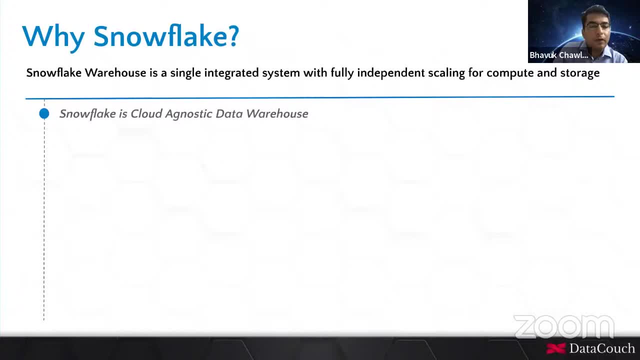 be specific to that particular cloud provider only, But we are talking about cloud agnostic solution here. Second thing is it supports modern features that cloud basically offers because it is cloud native, So we have auto scaling functionality. Yes, That means if number of concurrent users are increasing, then you can scale up. 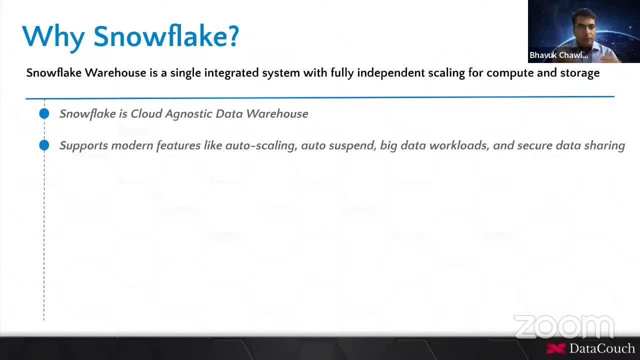 And if load is going down then you can scale down. You can choose, You can even schedule that. on weekends I want less load so you can reduce the cost, But on big days you want more load so you can change the capability of the machines. 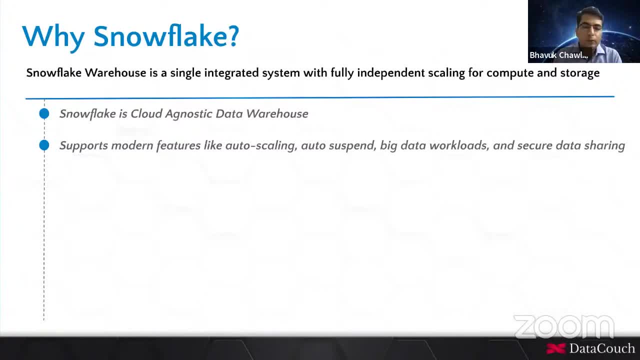 that you're running So you can schedule these things. You can have tasks in Snowflake through which you can implement such kind of optimization- cost optimization. So we have auto scaling, We have auto suspend big data workloads, we can run and secure data sharing, which is 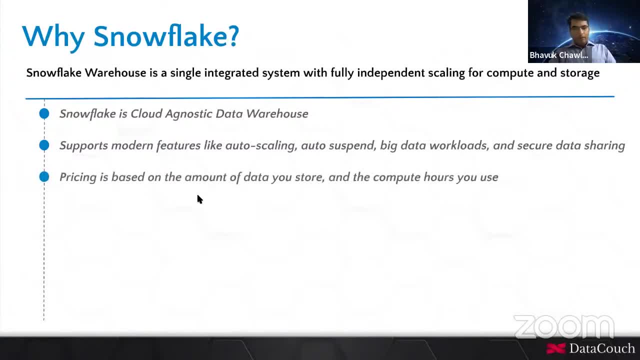 very powerful feature of Snowflake. So we have a pricing model in which we can pay for the amount of data that we store and also how much compute we are using. When we fire the query, when we run the queries, then only we pay for the query runtime, right. 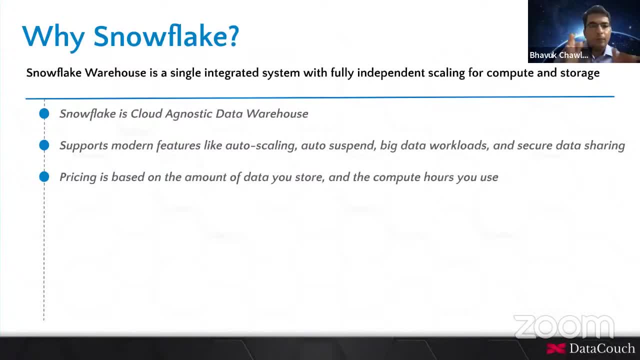 So we are not paying for running the machines, but we are just paying So we can optimize, We can set up the functionality in a manner so that we just Let's say, when you are at the right light, you can turn off the car because you are not. 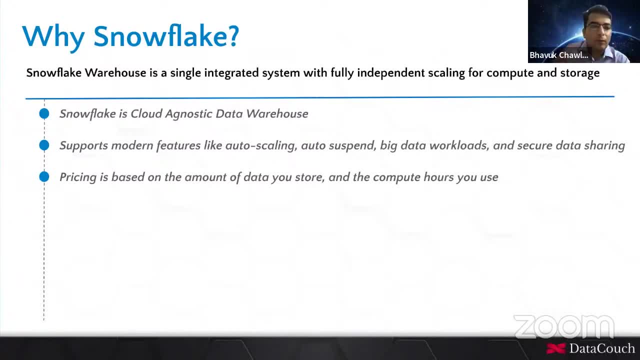 right now driving right, So you're just waiting. So same thing: when no queries are running on your warehouse, you can turn off the warehouse so that you are not spending money. Yeah, So same thing is applicable. So you have auto suspend functionality in Snowflake, through which you can optimize the 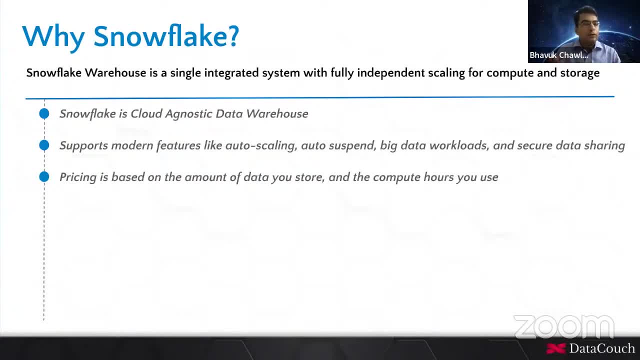 cost And as soon as you fire a query on Snowflake, then it will auto resume. You can set that functionality also During the demo. I will show you how this can happen, So you don't have to. You don't have to worry about managing it, scaling it right. 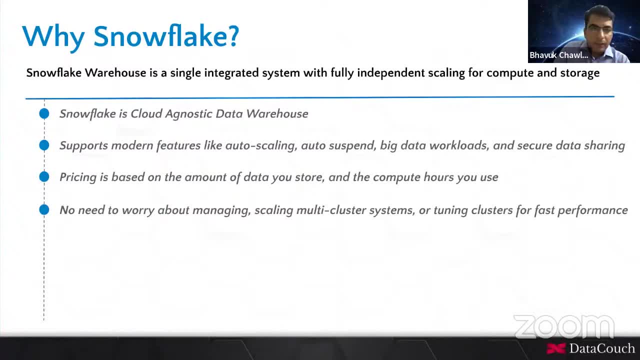 So as an administrator, as a database administrator, it's really painful to manage data warehouses, but Snowflake is removing all these pain areas and you don't have to worry about a lot of things as an administrator. So it's reducing a lot of overhead- the operational burden that we are having as a database administrator. 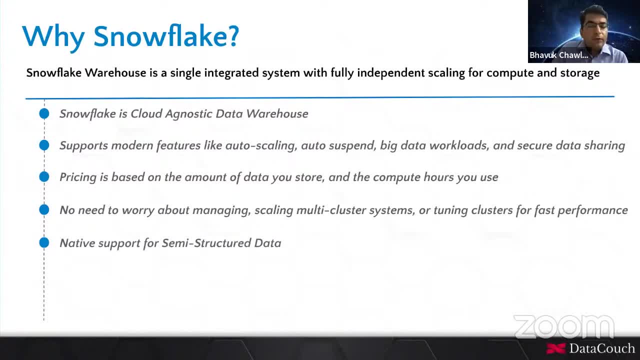 So it is having native support for semi-structured data. This is another beautiful feature about Snowflake. You will find there is a patented. There is a white paper from Snowflake. If you search on internet, you will find Snowflake white paper on semi-structured data. 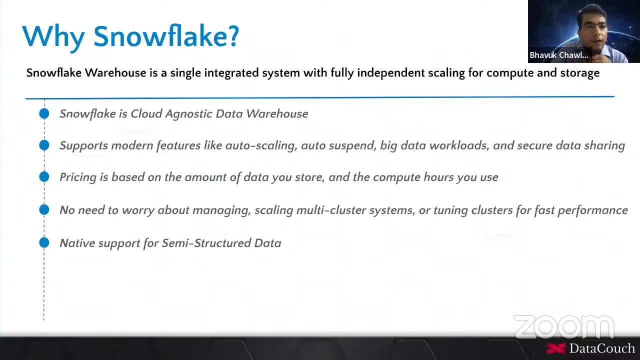 You will find how this has been implemented In other data warehouses. you will find semi-structured data is like a black box and data warehouses they cannot parse that semi-structured data field. It's like maybe glob, blob or string. So it's not very useful in other data warehouses. 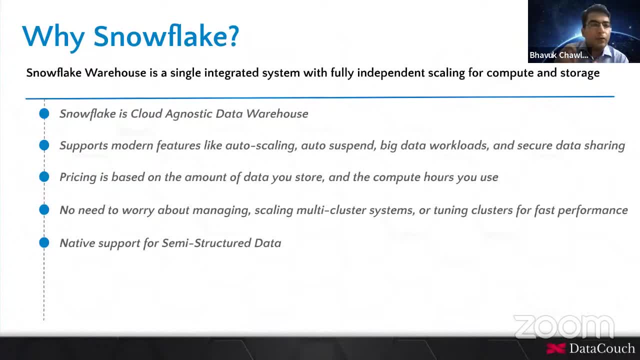 But in Snowflake the semi-structured data can be parsed by the query optimizer and it can build very optimized plan based on the data warehouses. So it's based on the structure of your semi-structured data, The level of nesting that we are having in the semi-structured data. 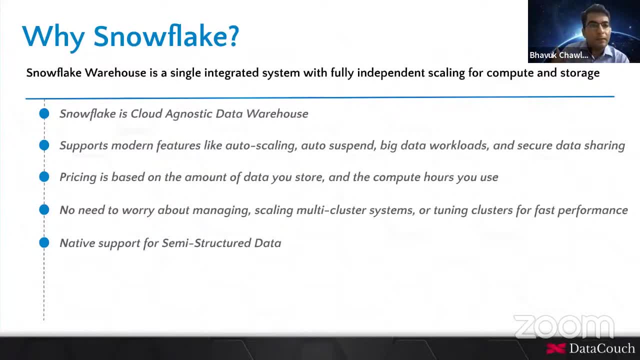 So that's another beautiful feature of Snowflake: that it supports semi-structured data natively. It's first class citizen in Snowflake. It's not something which is like a black box for query optimizer, and storage is the way it is stored. It is also very much optimized. 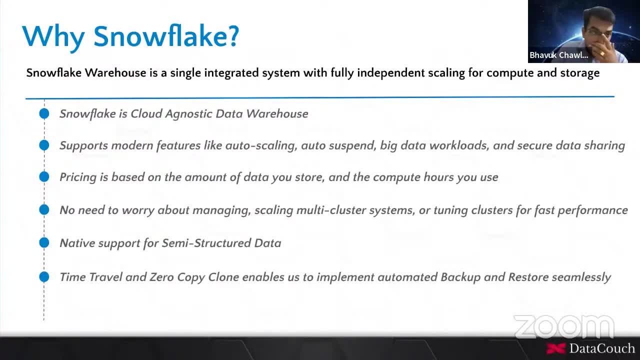 So Snowflake supports time travel. That means you can go back in time You want to. Let's say, by mistake, you drop the table, You want to restore, You want to go back. So there is a limitation on, like, how much time you can go back, depending on the edition. 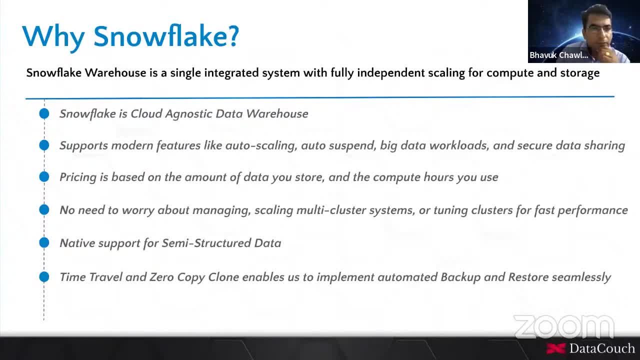 of Snowflake that you have chosen. So let's say, you have an enterprise edition that we will be using in the demo. So then you can go back, like last 90 days. Within last 90 days you can go back in time. and that too for permanent objects, not for 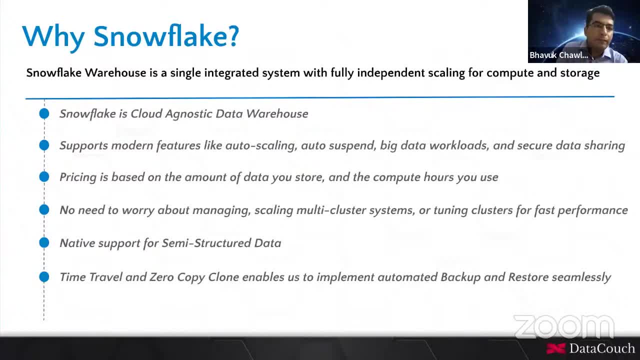 temporary objects or transient objects, but for permanent objects you can go back in time for last 90 days. So time travel feature is also there. And then we have zero copy, zero copy clone, So you can create different environments. So let's say you have a prod environment. 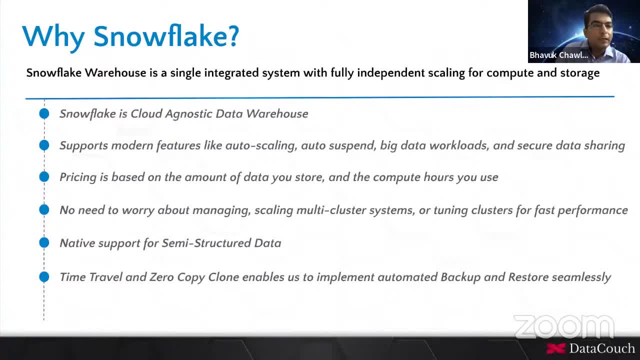 You want to create staging environment, You want to create QA environment, You can do it in fraction of seconds because it is something which is called zero copy clone. You are not copying data from one environment to another, but it is more like metadata based. 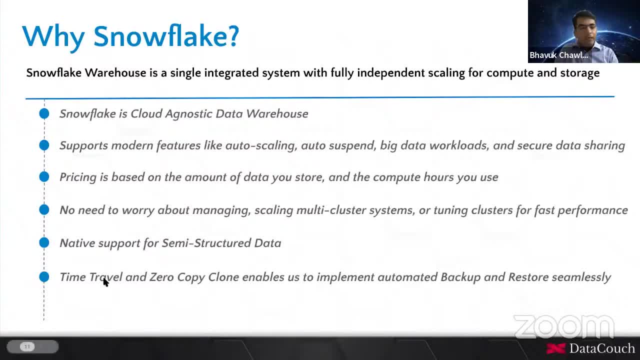 operation through which you can create a copy, And then the combination of time travel and zero copy clone can help you in achieving backup and restore functionality in Snowflake. So Snowflake has many features. If you give me one hour, then I can talk more about that. 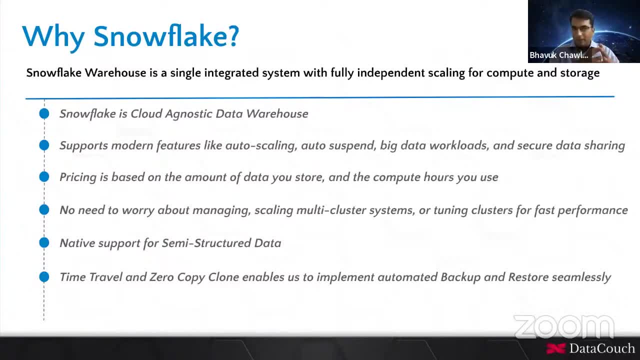 But the purpose of this webinar is to go through the web, Like the web, So you can see the overall crash course on Snowflake. So we want to see some demo of Snowflake and how to get started with Snowflake. So I will be going to towards like query plans and some of the other interesting areas. 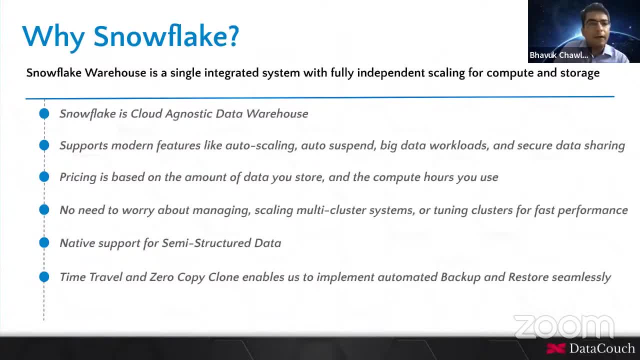 So just stay tuned, But if you have any questions still now, please feel free to ask. I hope you got it, Like why Snowflake is so useful and how it is helping us in achieving scalability and elasticity. and it is- it is cloud native. 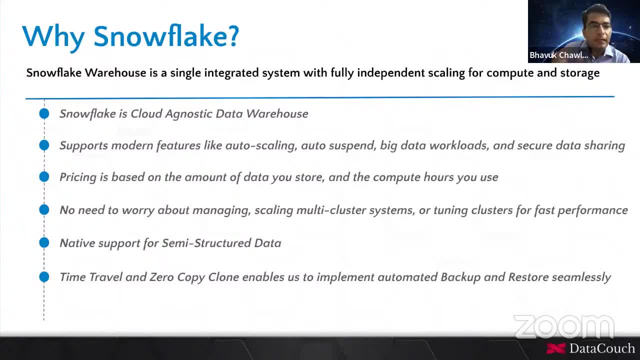 So these are all benefits of Snowflake. It's all decoupled architecture And compute. they are decoupled, So storage can scale independently and compute can scale independently, So it's very secure. So I will talk about security in more detail when we are comparing various editions of Snowflake. 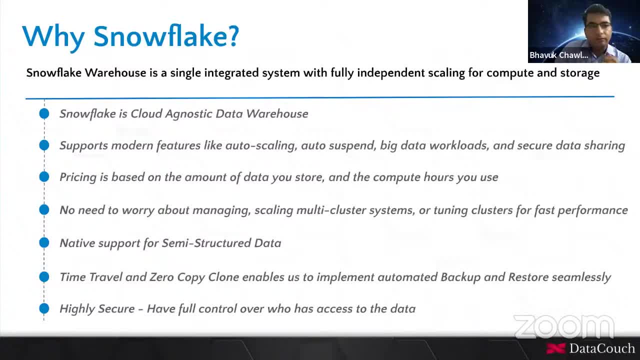 So we have standard edition, We have enterprise edition, We have a business critical edition and then virtual private Snowflake. So we'll see there are, like, different features offered by Snowflake in different editions of Snowflake. I'll show you how it works, but it is highly secure. 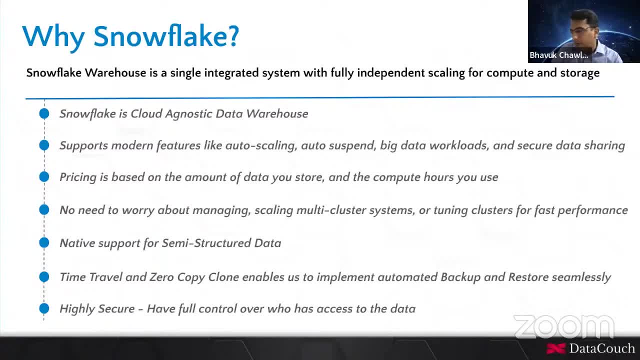 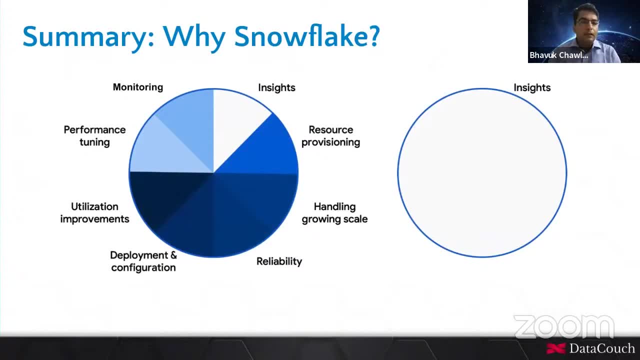 And We'll find the various compliances. that already follows right, So we'll look into that. So in summary, in short, what we discussed till now in like a lot of other data warehouses, you will find you are spending a lot of time in like resource provisioning, you are handling the growing scales. 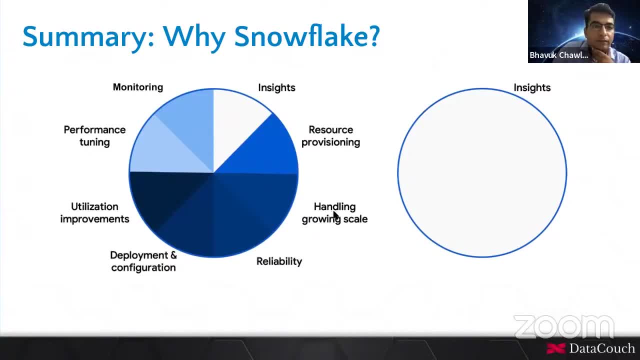 So you are worried that hard disk will be full, like a lot of data is being ingested. You are worried that on festival there will be a lot of data arriving and data velocity will be very high. So If you are working as a database administrator of traditional data warehouses, you will find these issues can be overcome through Snowflake, because in Snowflake you can focus on. you can focus on the insights. you are focusing on actually getting value out of like, out of the data, rather than thinking about 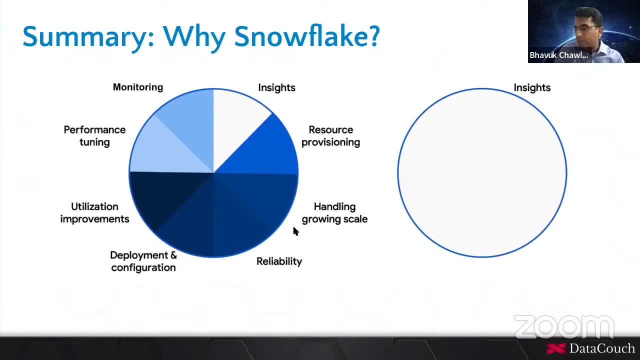 rather than thinking about growing scale, like if hard disk will be full or my machines will be less, how I will be handling the data velocity And how you are taking care of performance tuning. So you are. you are thinking a lot If you are working with traditional data warehouses, but when you are working with Snowflake, you focus on your business use case and get the value out of your data rather than thinking about all these operational things. 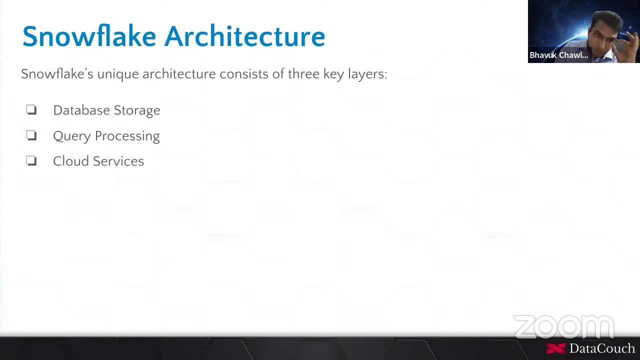 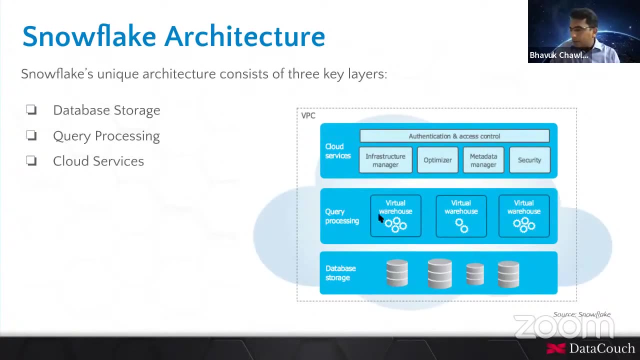 So now, uh, Snowflake architecture. So in Snowflake architecture, this is three layered architecture and this layer is called database layer, This layer is querying layer And this layer is called cloud services layer. So in this Snowflake architecture, you will see, in database layer, we are storing our data. 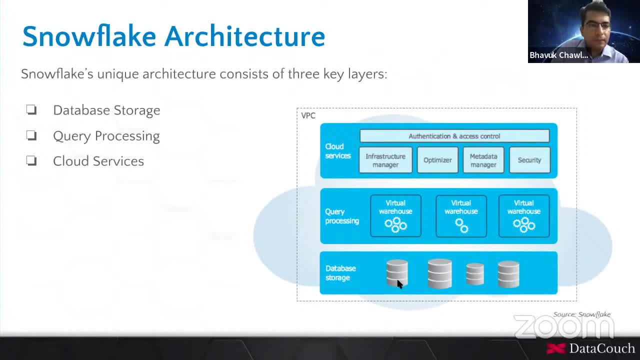 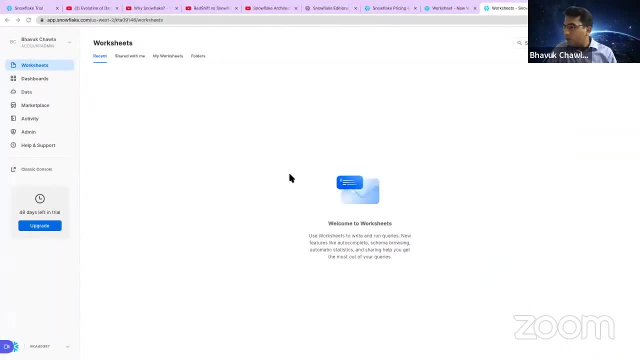 So this storage layer can be on AWS, It can be on GCP, It can be on Azure. Yeah, So this is one picture that I want to show you. along with that, I also want to show you architecture. I have few videos on Snowflake. 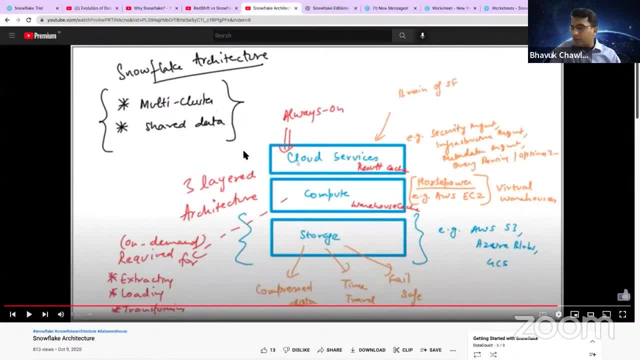 You can watch these videos whenever you get a chance. it's there on our YouTube channel and I can share the details about the YouTube channel. So what I want to share here is, like Snowflake architecture. There are like, if I make it bigger, there are three layers. 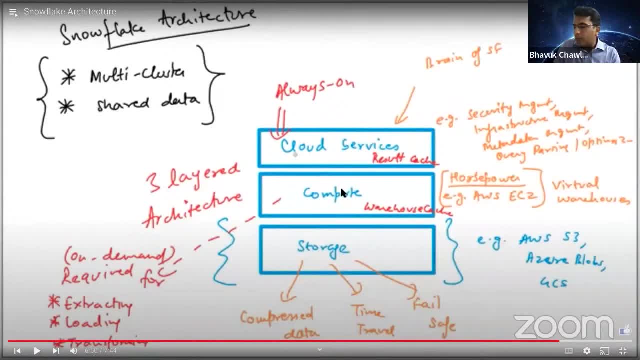 So one layer is storage layer, Another one is compute layer and third layer is cloud services layer. So storage layer is actually storing your data and it's like infinite storage. You can store any amount of data. in traditional data warehouses. We struggle a lot with the amount of storage that we are having because it is a cloud based data warehouse. 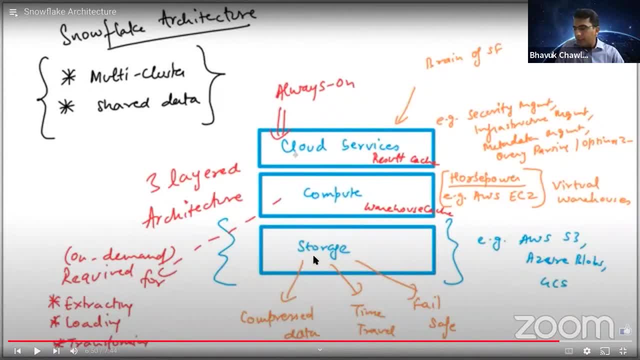 So storage is not limited. So you can- Yeah, So you can- have data here and then you have data for time travel also. So all data is compressed and it's in columnar format so that the querying is easier for historical data and time travel can be performed. 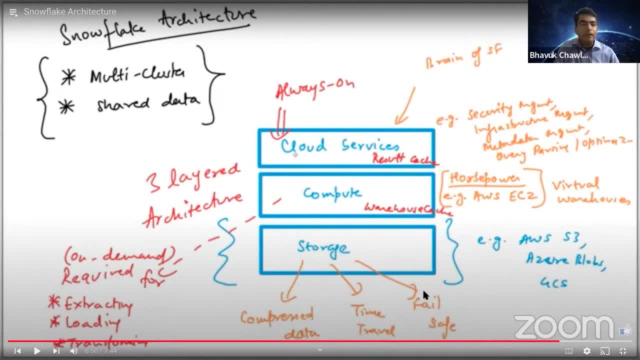 You can go back in time- So it's also part of the storage layer- and fail safe. You can recover data once time travel period is over. then you can request Snowflake support to recover your data. It's like retrieving data from your recycle bin. 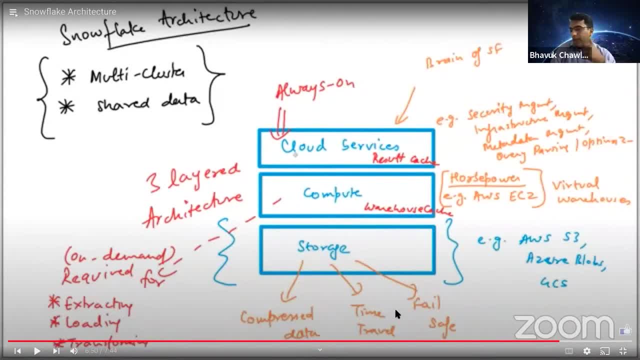 So it's fail. safe period, which is seven days after time travel period. So that's the storage layer, which can be S3 blobs or Google cloud storage. Now we have a compute layer. compute layer is on demand, So that means this is horsepower. 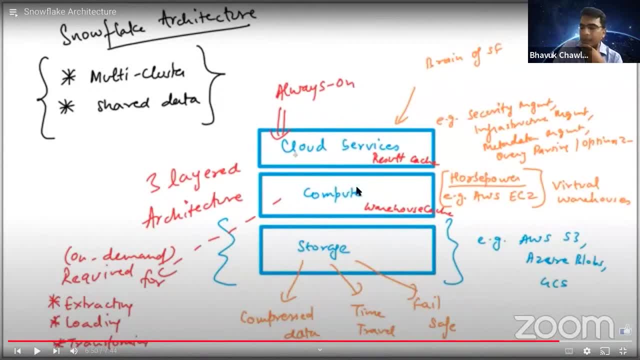 This is the place where you will be fired, Like when you fire a query, then the queries are executed through compute, So it's like EC2 machines running under the hood If you are talking about, let's say, Snowflake is running on AWS. 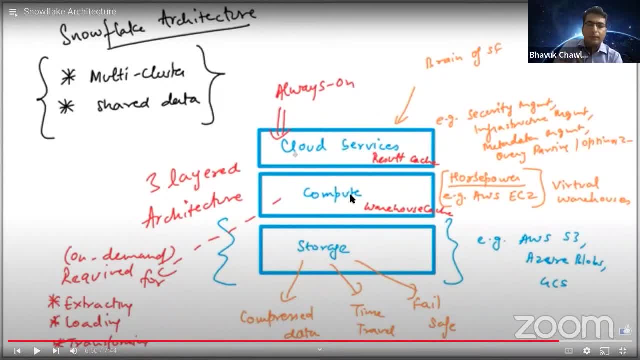 Let's take that example because in demo also I'll be showing- Snowflake is running on AWS. So compute layer is like machines are running and they are running your queries. They are running from the storage and let's say you are ingesting data, you are loading data into Snowflake. then also compute layer is actually executing those load statement, the copy statements that you are having. 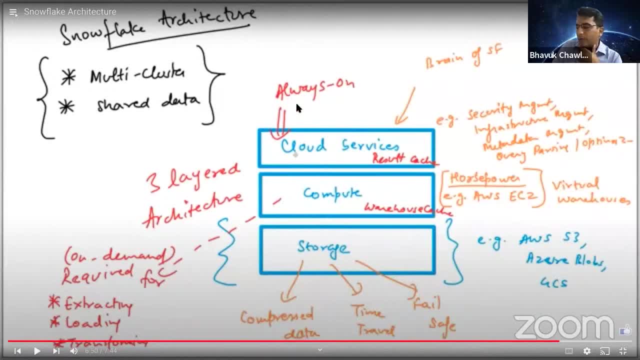 And then we are having cloud services layer, which is always on, which is 24 by seven running, And this cloud services layer is responsible for security, infrastructure management, metadata management, query parsing, optimization and many other reasons we need cloud services there. 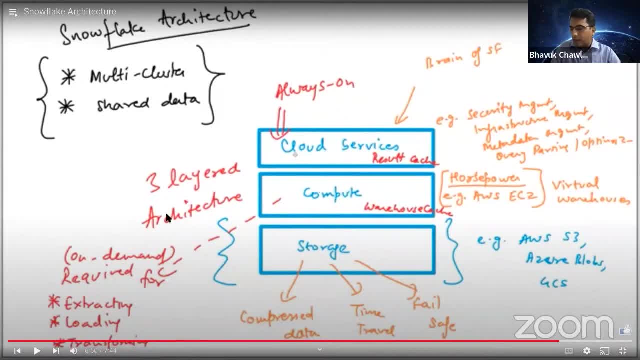 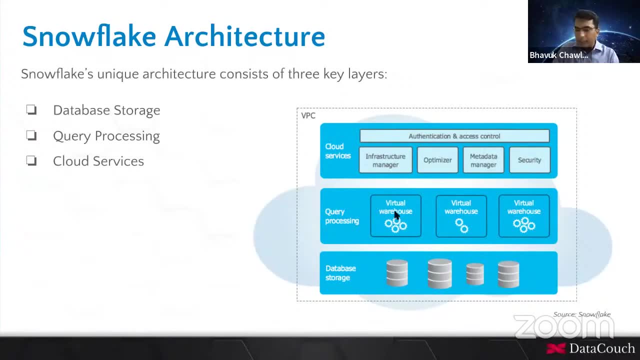 So this is a three layered architecture, Data is all shared and this is multi-cluster architecture, So I hope you got it Like there are three layers in Snowflake architecture. and this is for storing your data, This is for running your queries and this is for your metadata, your caching, your security, your optimization of queries. 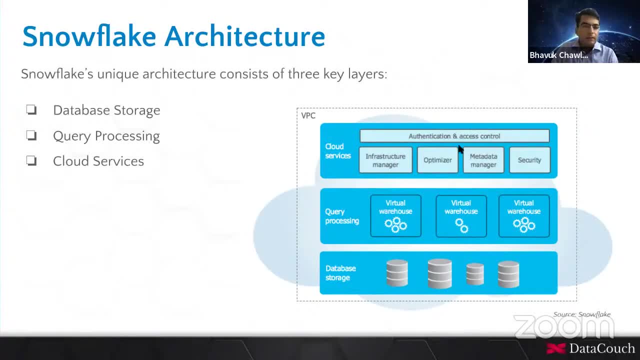 Yeah, So all these things cross cutting concerns are taken care by cloud services layer. I take a pause. If you have any questions, please ask. I will wait For a few seconds And probably it looks like we have a couple of questions in the Q and a tab. 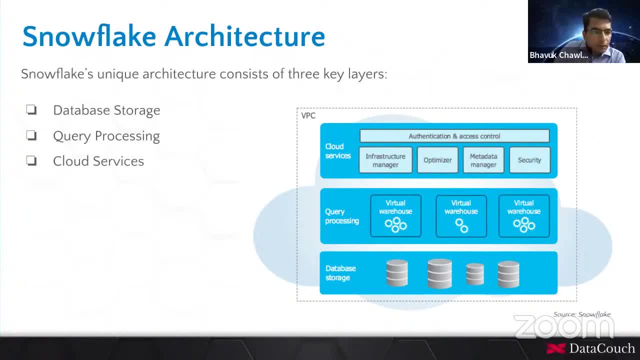 If you can open that up, give me a second. Uh, okay, So okay, Okay. What is the difference? Okay, This is taken care. difference between database and data warehouse. I'm just getting started with Snowflake. after the, how do you go in depth into Snowflake? 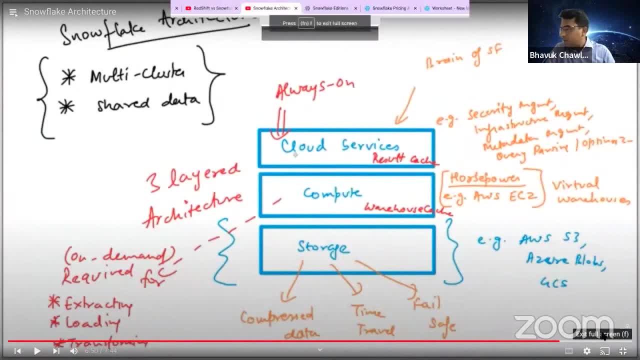 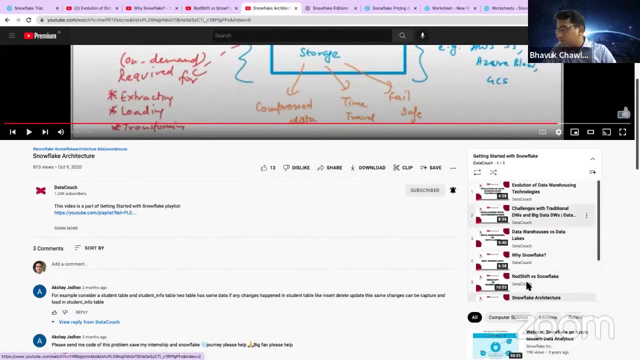 So I would suggest there are few videos that I've created. You can watch these videos and I have some recordings also on the YouTube channel So you can watch those recordings. So if you go here and you say there is a playlist for Snowflake, you can start with that. 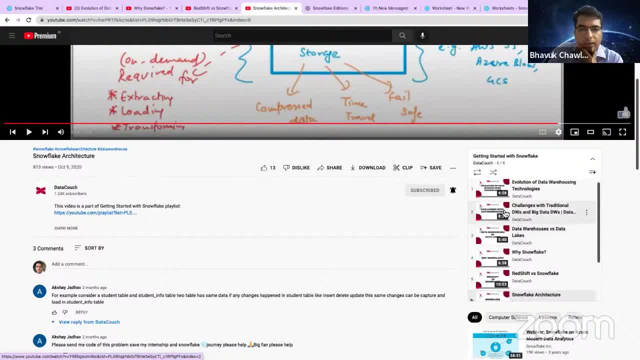 Uh, this can be a good starting point from my perspective. This, this, this should help you like how to work with Snowflake. Uh, okay, So now next one is. next question is: what skills do you believe are required before even considering Snowflake- uh, Snowflake- data warehouse management. 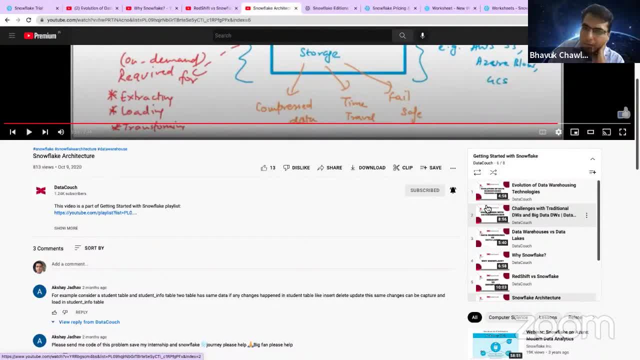 So, Ali, uh, that's a good question. So you should be familiar with, uh, the data warehousing concepts as such. Uh, you should be clear about the data modeling approaches, right? And you should know, um, some basics of SQL and RDBMS before you move into Snowflake. 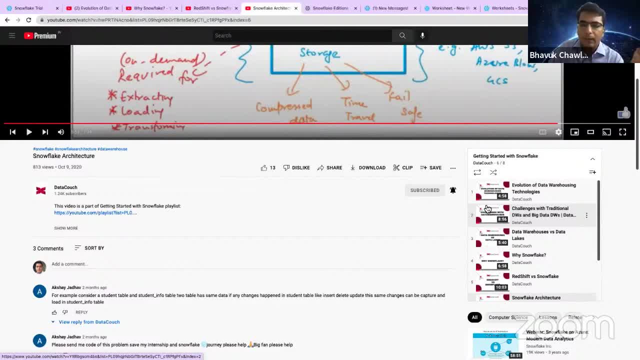 So if you are comfortable with basics of SQL RDBMS, you are clear why we need data warehouses, What is the difference between data warehouse and data lake And what is the difference between data warehouse and transactional data databases- then you should be good to go. 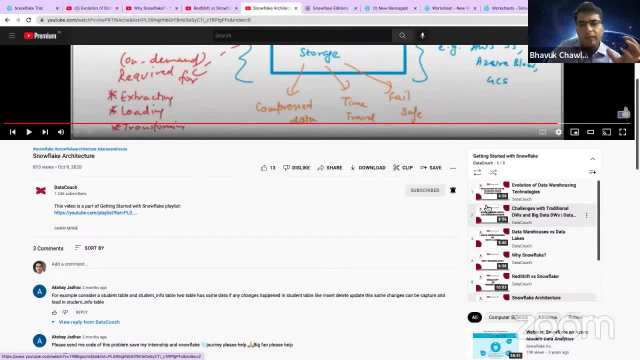 And you can easily learn Snowflake. The learning curve is low. Best thing is like: if you know SQL, then you can learn Snowflake very easily. But if you want to understand the internals, then you should basically start learning how the columnar structure is. 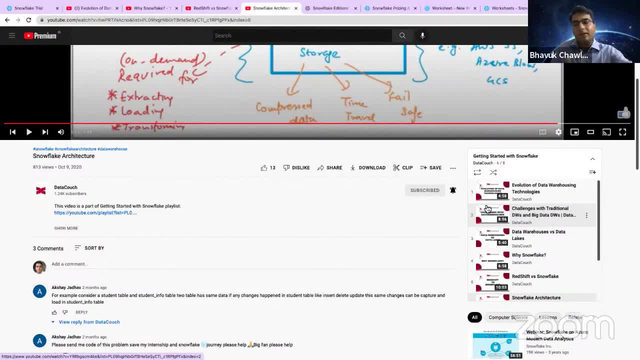 You should start learning about the open source technologies that we are having, For example, um the parquet format. in like uh open source world, you will find a lot of similarities of parquet with the FDN format that Snowflake is using. 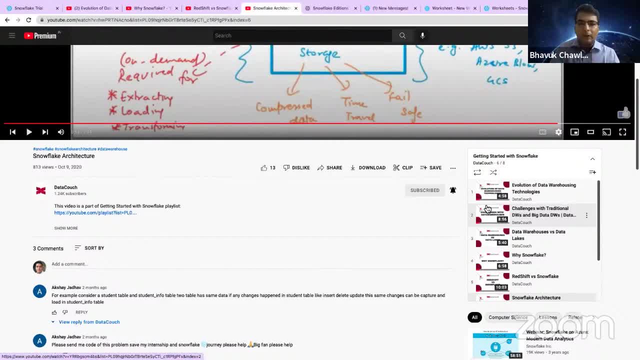 So, Ali, this should answer your question like: uh, relate with the open source technology, because a lot of things in Snowflake are hidden. But if you know Spark, how Spark optimization work, how the query optimizer in Spark works, then you will be able to relate with Snowflake. 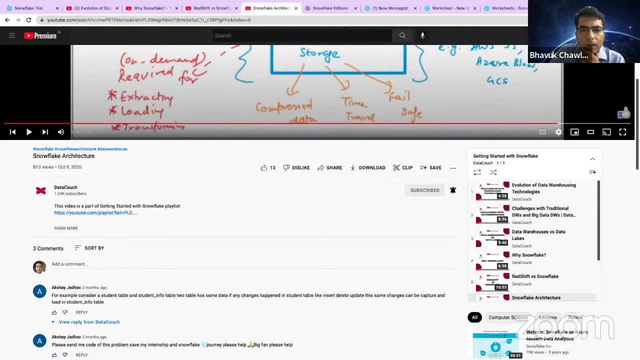 So that is a quick answer. Um, now another question is: uh, there are like, let me, so, let me sort it. Okay. So I see the questions are changing. So how would you, uh, how would the functionality of Snowflake differ in different cloud services? 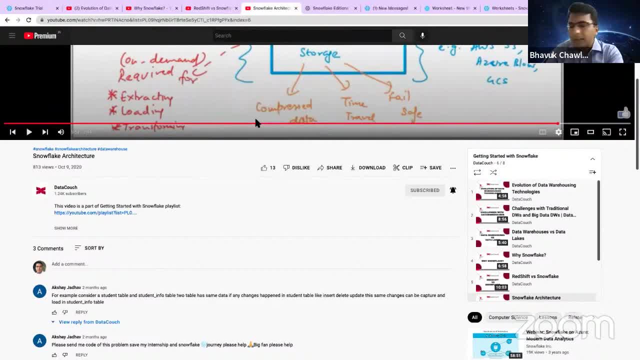 So yeah, so you will be going to the regions where you will see the limitations and where, in which regions, Snowflake is available. Uh, I would suggest go to that Page where you will find, uh, region specific information and cloud space cloud provider specific information of Snowflake. 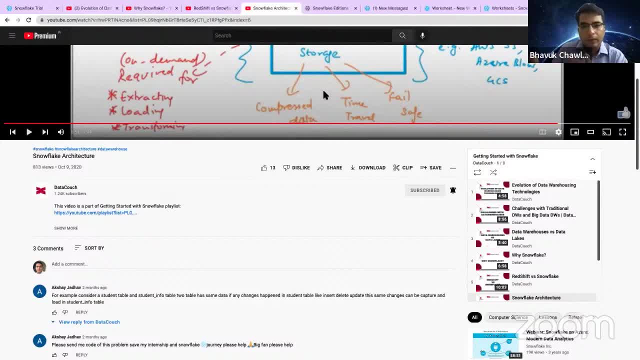 There is a page on the Snowflake document documentation itself where you will find all the caveats and things to take care of. Uh, so this is well documented on the Snowflake website. What are the benefits of Snowflake when compared to Redshift? 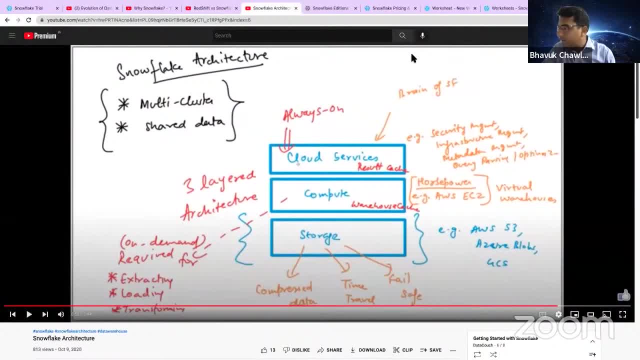 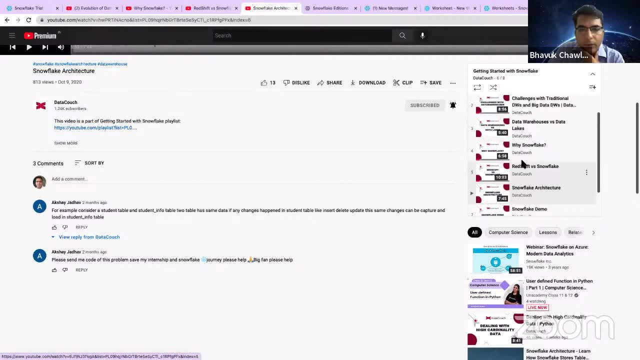 Okay, great, So you will find I have a video on Snowflake versus Redshift. When you are going through this, you will find there is a video, uh, and it is 10 minutes video. I would highly recommend please watch this video. 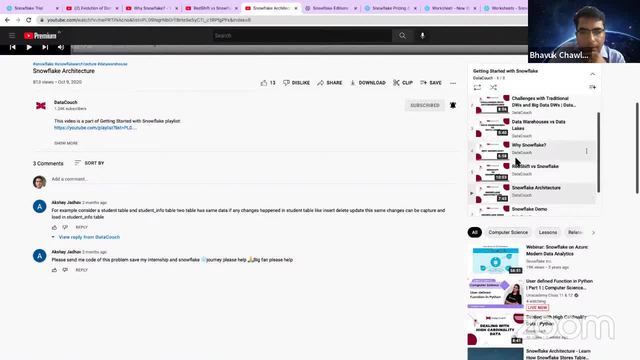 You will get an idea of how Snowflake is different from Redshift. Yeah, Which querying language is used? We use Snowflake, So it's no SQL query language which is used and it is very much similar to the ANSI SQL that we are having. 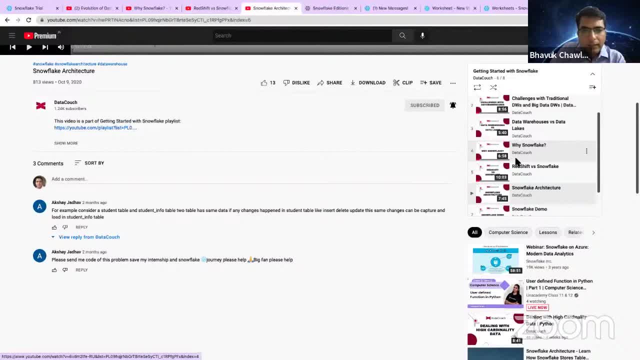 Would I need uh? Rohit, I hope you got it. You got the answer. And Ali, I hope you got the answer. How Snowflake is different from Redshift. Uh, would I need AWS Azure working knowledge to start learning Snowflake? 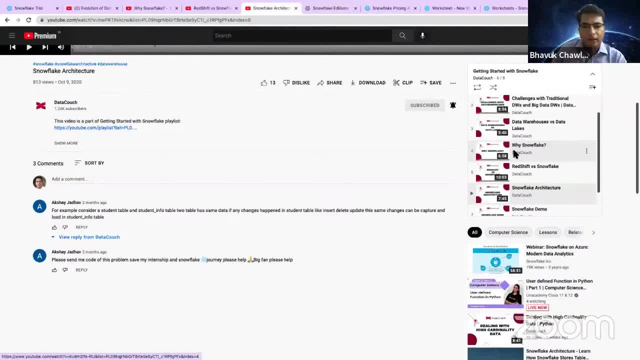 No, it's not mandatory, but yes. when you are integrating Snowflake with uh like streaming pipelines, building such streaming pipelines, or you are creating external stages, then uh, this knowledge will help you. when you are integrating security of AWS with Snowflake, then this knowledge will be required. 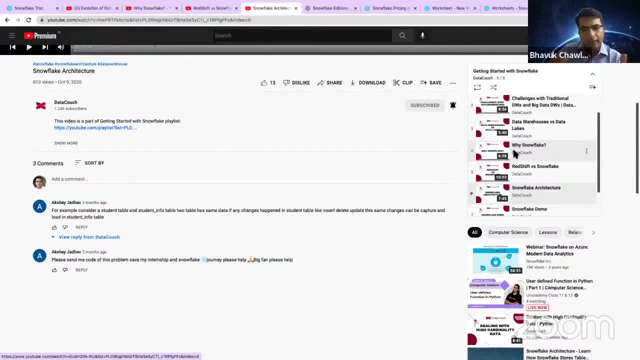 But when you start learning Snowflake you can get started very easily. but later on you can add that knowledge and you can build streaming pipelines or or external stages on your cloud provider and integrate with Snowflake, depending on your cloud strategy that you're having. 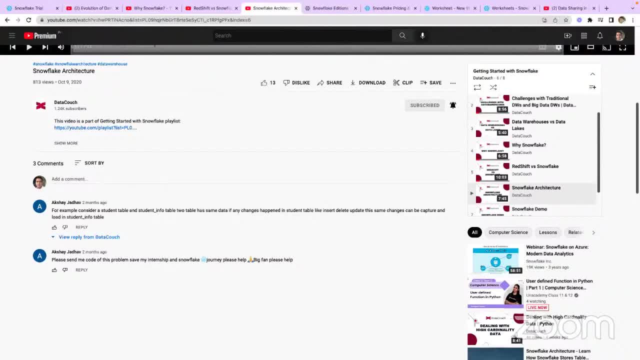 So, um, uh, yeah, so I will talk about the freemium option for Snowflake Freon, So we will look into that. Snowflake support OLTP modeling as well, Or so. Snowflake is a data warehouse and it is for OLAP, for for OLAP based use cases. 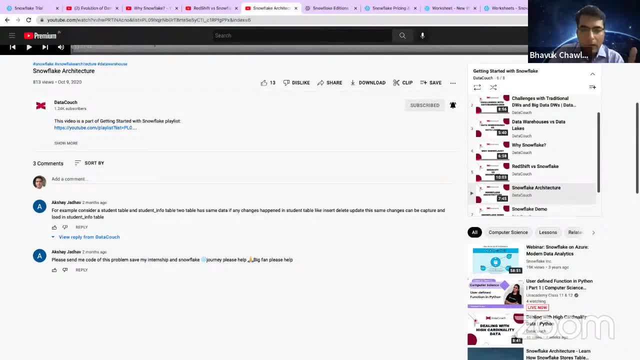 And the storage in Snowflake is columnar and it is good for OLAP based queries, not for OLTP based queries. OLTP based queries will be slow. when you are just working with single record, it will be slow. Snowflake is not for that purpose. 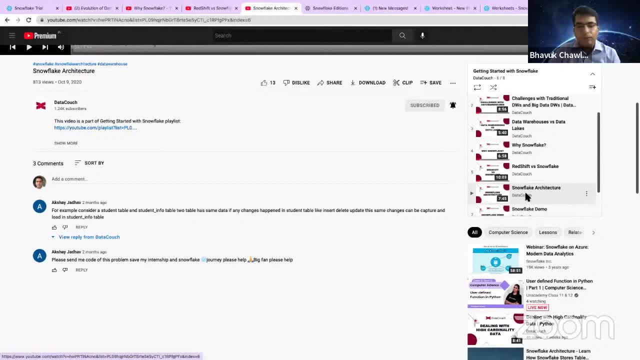 Uh, what is the benefit of Snowflake compared with Redshift? So there is a video. please watch that video- Redshift versus Snowflake, And here you will find it. So this is the playlist where you can watch. I can share that. 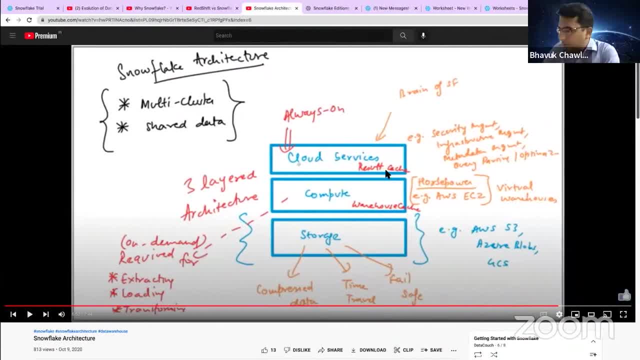 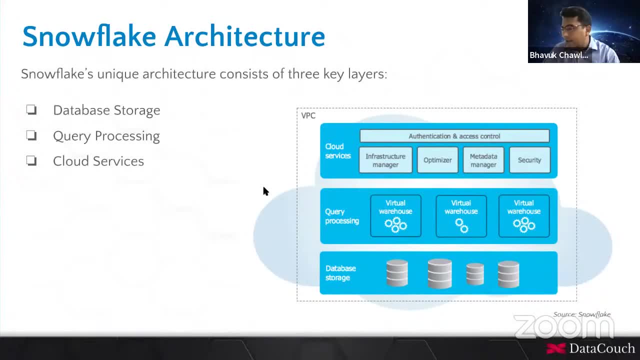 Okay, So now, coming back to this, uh, I think we will continue. So, um, we have three layered architecture, So we are talking about Snowflake, which is a platform, and it helps like to ingest data from various data sources. 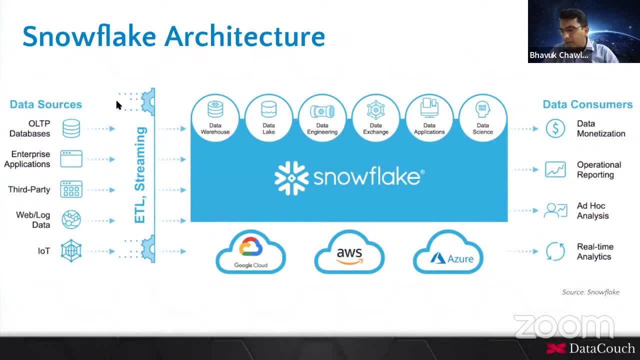 We are bringing data from different data sources and then we are working with that data on Snowflake platform. So this platform can be used for interesting things. like you know, used for multiple purposes. the platform is helping data warehouse engineers um data data warehouse. 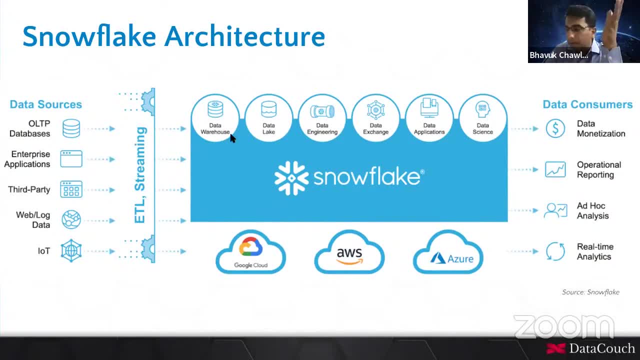 uh, like people who are working with data warehouse, housing, for example, data analysts. it will be good for them. it is good for people who are working with data lakes. it is good for people who are having data engineering background. it's good for people who are sharing data- uh with among. 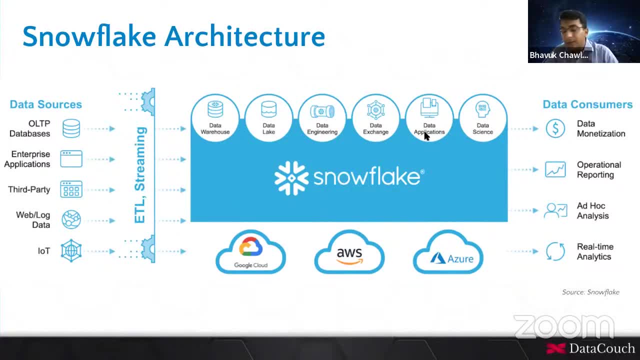 different departments. it is good for people who are building applications- data intensive applications on snowflake, and it's even good for data scientists when you want to do quick feature engineering. so let me take a few more questions. i'm i will just see. why would someone opt a cloud? 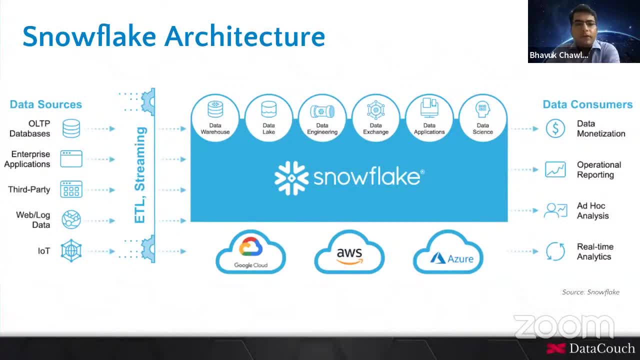 provider themselves come with similar options. okay. so, janty, it is more about like, your cloud strategy in the company. second thing is, like you need to see the cost model that you are having. third thing is: you need to see, uh, the vendor lock-in that you are having. um, you need to see, like uh. 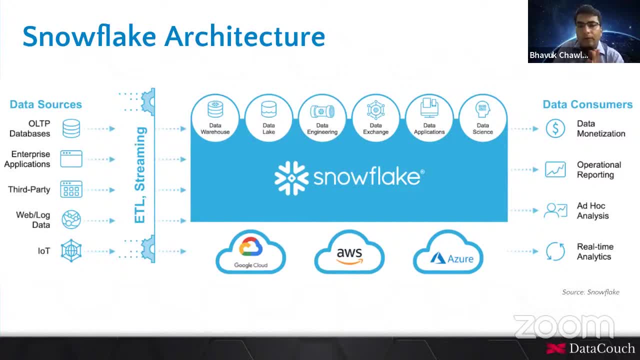 integration with your native cloud provider, which is your primary cloud provider, and what kind of support that particular data warehousing technology is giving. so you have to see multiple factors before choosing a particular uh technology as such, and so, depending on that semi-structured data support, if your cloud provider, how much semi-structured data you are processing. 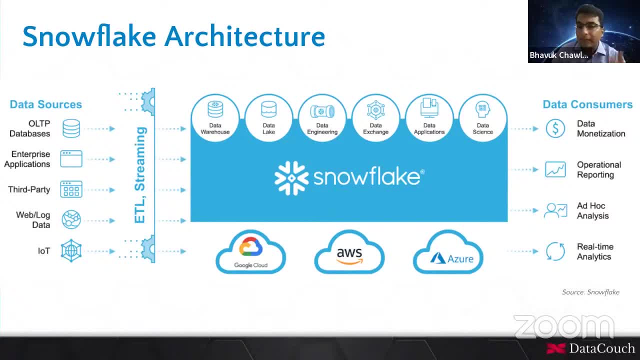 and integration with your partner tools that you are having etl tools like, for example, you have tools related to transformation. you have preferred tools. you have already got support for that tool for next one year, less next three years. then how we are integrating with snowflake- so a lot. 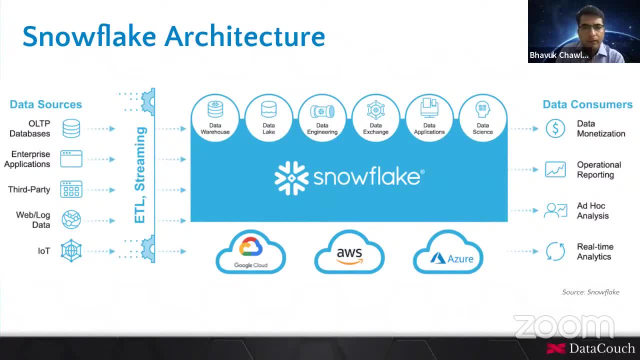 of factors will come into picture when you are opting for a particular data warehousing service. yeah, so to learn how snowflake works, would it be? would i have to integrate with cloud service to begin learning snowflake hands-on? so you can get started? i'm i'm showing you the demo how. 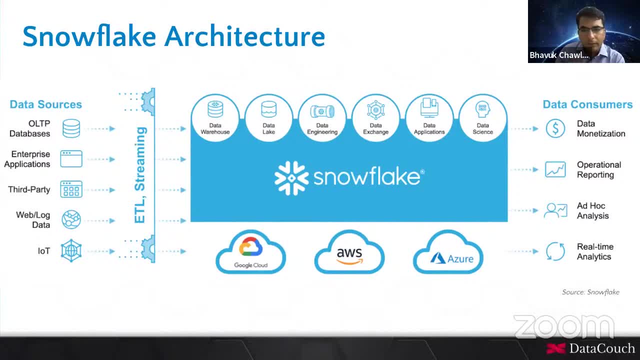 you can get started with snowflake. uh, just give me two, three minutes. i will come back to this. how should i start with snowflake if i know aws? yeah, so i'm going to start with aws, so i'm going to, I'm going to show you that, don't worry more. like a business decision. yeah, business decision as well. 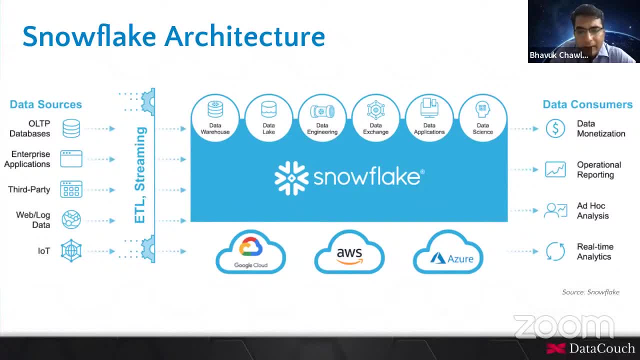 as technical, technical things also, like the overall strategy that you are having related to the cloud data and what is your like costing, yeah so return on investment and how much upfront investment you want to do, and what are the partner tools that you are having ease of integration. 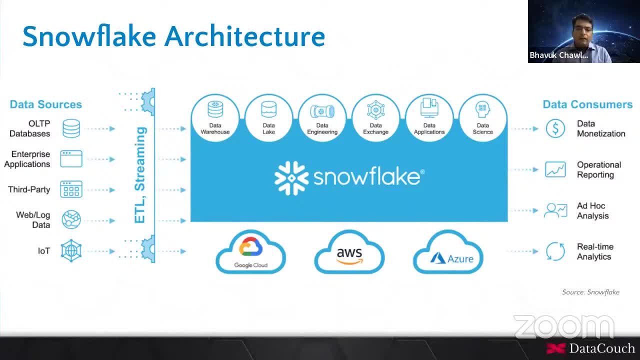 skill set that you are having right. so what is the learning curve that you are having right? so all security compliances. you know different snowflake additions. they are having different offerings, so which snowflake addition are you planning to use? and then, based on that, you are comparing some other product and then you are looking into pros and cons. yeah, what? 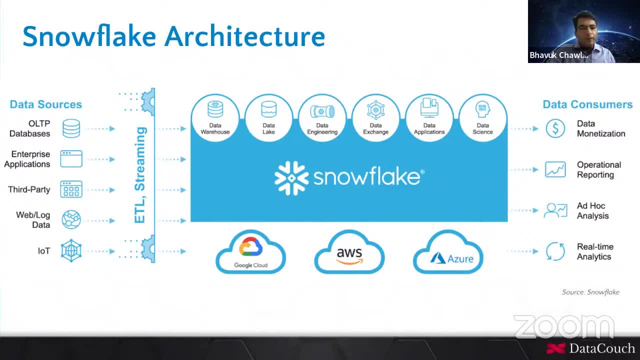 requirements are needed to install learn snowflake. is there free bundles? yes, now I'm moving into that. so there are so many questions: how do we work with snowflake? so let's go into that. so I hope you got it. like, snowflake architecture is one single platform which can run on AWS, Google Cloud. 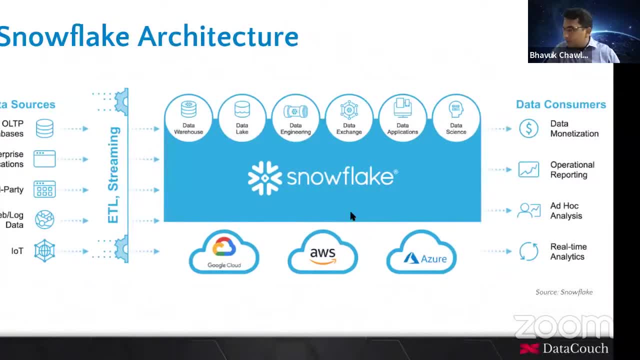 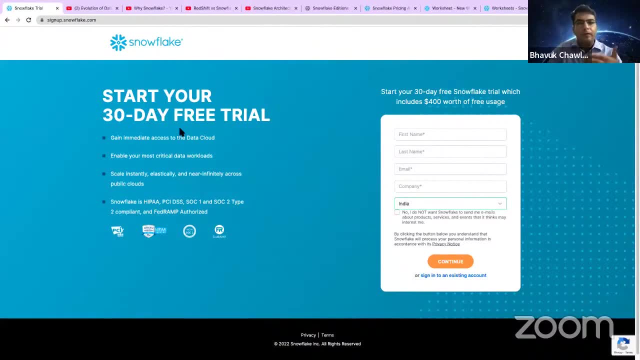 Azure. Yeah, so let's start. okay, so let's start with snowflake. there are so many questions, so this is a very first page, like in case you want to learn snowflake, so you can start with a trial edition. so you'll get free trial and you get $400 credit. so I just created one account working with snowflake. 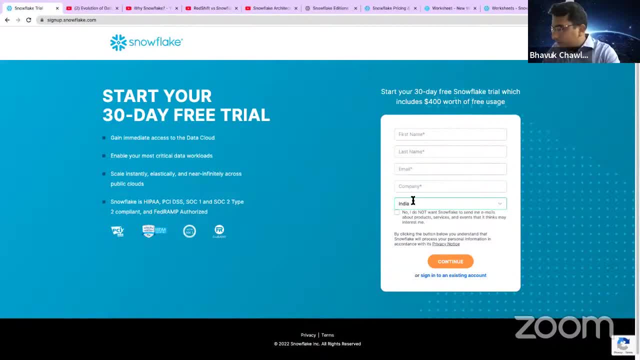 so you can easily create one account by just registering yourself, and there is no credit card required. that's the beauty of this platform. in other cloud providers you will find you have to sign up and then only you can work with that, but here, in snowflake, you don't have to provide your 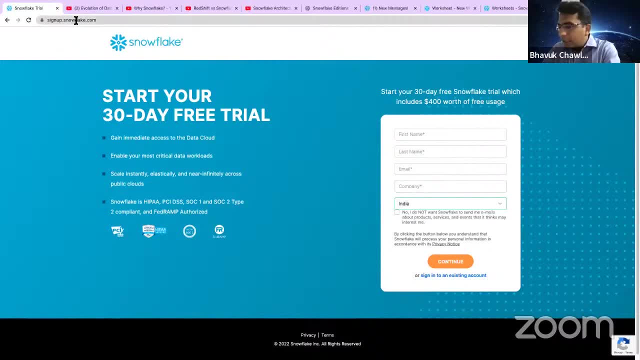 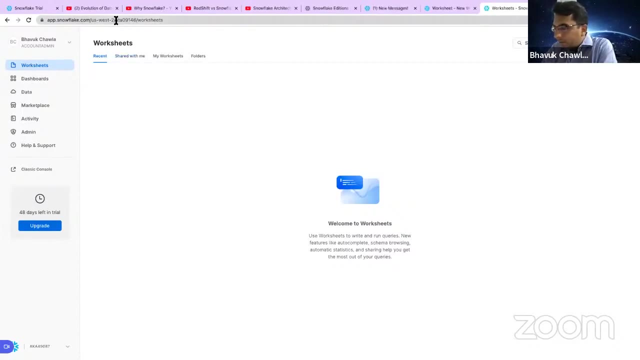 credit card information. yeah, so, so this is our signupsnowflakecom. yeah, so very easy link you can. I can post it on the chat also. so signupsnowflakecom, and after that you are done with the signup, you will be inside this kind of interface. so this is our snowflake interface, and 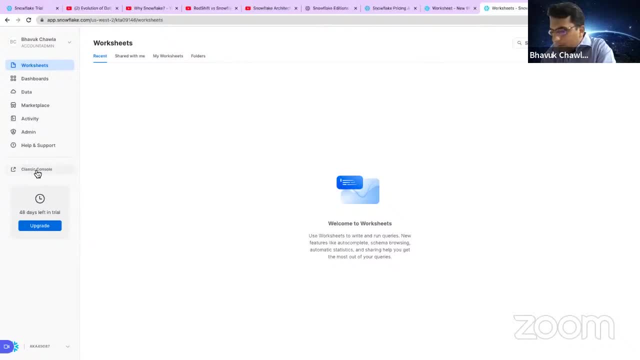 we have two, two consoles like. one is called classic console, another one is called: this is the latest console that we are using and this is the latest console that we are using and this is the latest console that we are having. you can, this is a browser-based console, so I am just 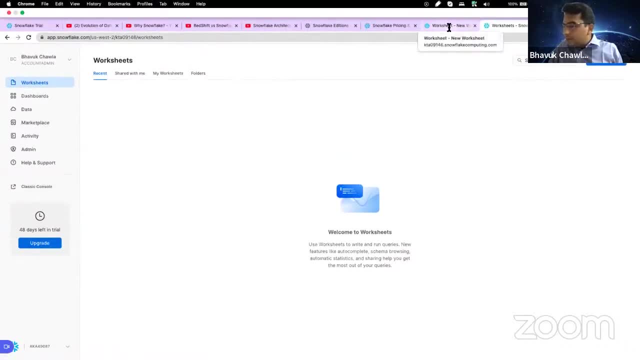 switching back to the classic console and we'll show you some interesting things from the classic console, and then I'll come back to the latest console that we are having so that you can see what additional things had been added in the snow site or the latest latest playground that we are. 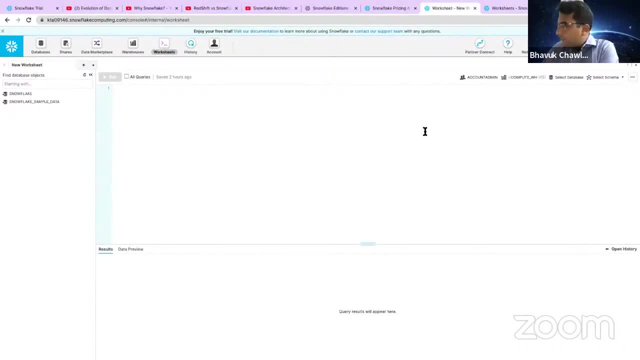 having. so this is our classic console and in classic console you will see we have on the top right is the highest role. if you ignore the org admin, the account admin is the highest role. so this is AWS account that we created, this snowflake account, AWS account. when I choose, 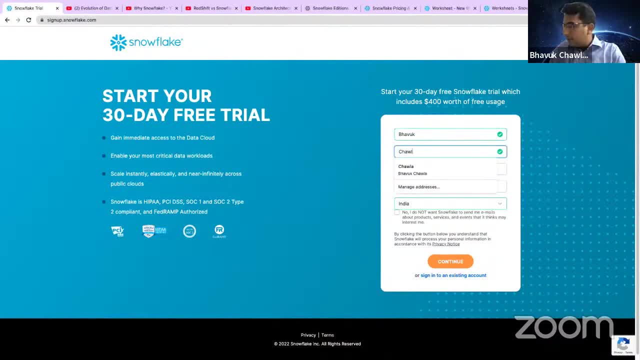 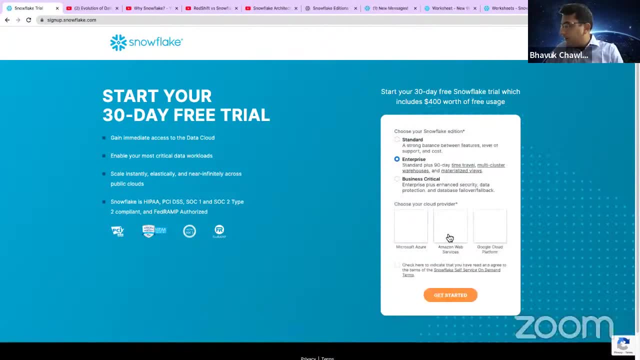 this option. so when I choose this option, I specified my details. so, let's say, I specified my details, I specified my email address, I specified my company name, yeah, and after that I just said continue. after that it is asking me to choose edition of snowflake, so I choose enterprise. 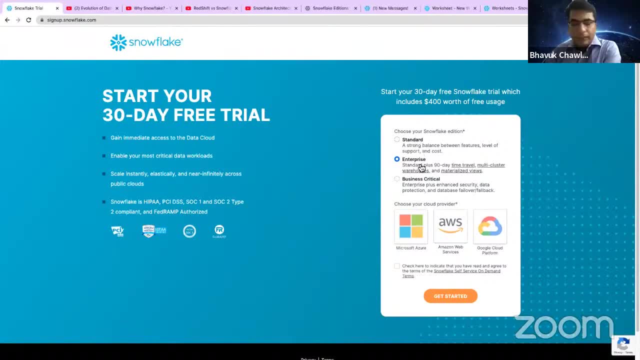 edition because standard edition has a lot of different options. so I choose enterprise edition of limitations, like compared to enterprise edition and it's all free. so i thought like why not we go for enterprise edition? so here i'm choosing enterprise edition and i will get multi-cluster warehouses and 90 day of time travel. so i'm choosing enterprise edition. 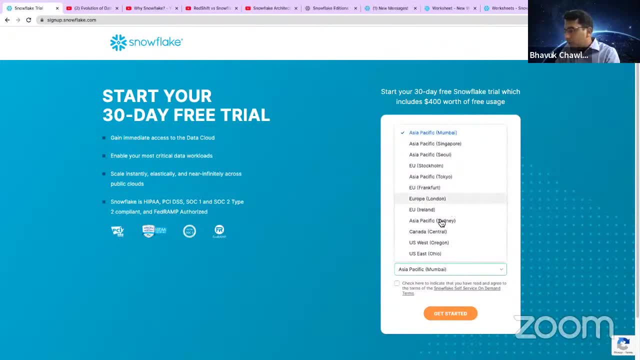 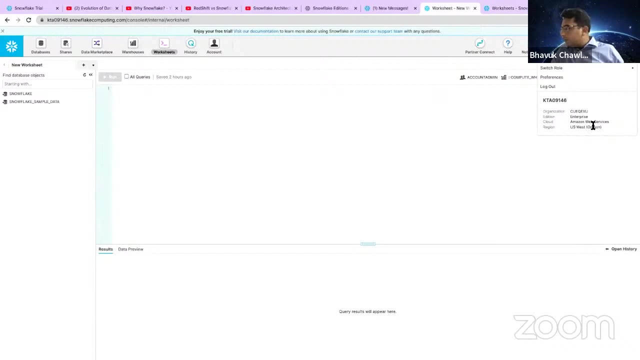 and then i am choosing aws, and then i am also choosing, uh, us west region, so aws and us precision, and after that i i just clicked on get started. so after that i am able to get an account which looks like this: so you can see it is aws and it is us west region and this is my. 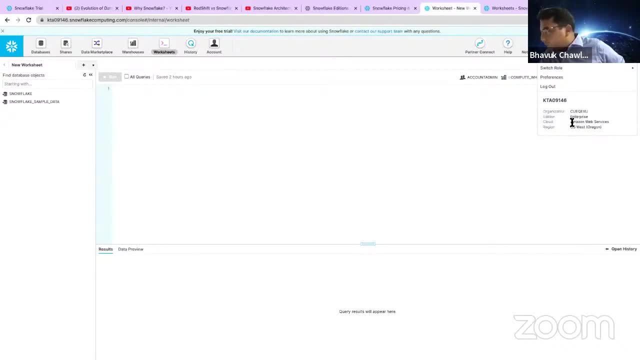 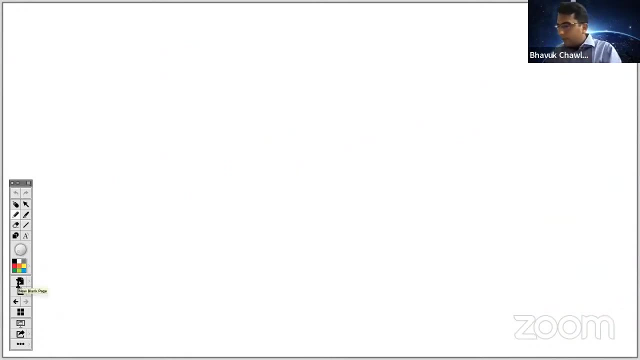 organization and then within that this is enterprise edition that it is showing. so this is one account. so in snowflake, if you go to the whiteboard, you will find there is a hierarchy. so so if you ignore organization, which is on top of the account, i'm ignoring that. 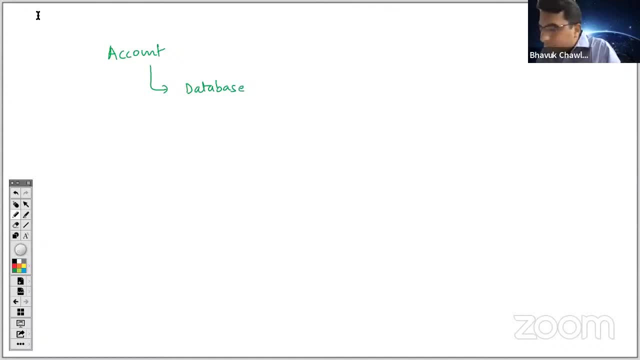 we have this hierarchy in snowflake, so we have: this is object hierarchy that we are talking about. so this is object hierarchy, or securable object hierarchy. so we have databases and there are other things also, we have schemas and there are other things also, and then we have tables, views and other things, right, so you will see that. 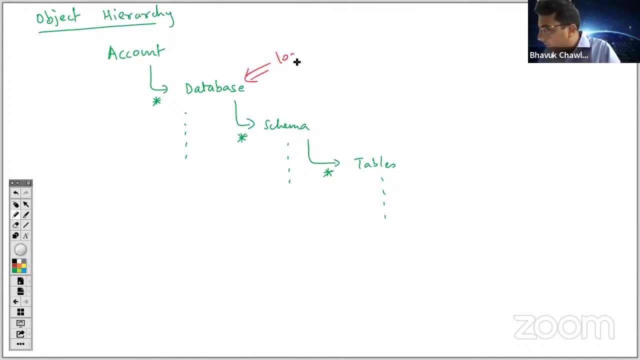 this. like you, this database is logically grouping various schemas. this is grouping various schemas and this is also logical grouping and logical grouping and it is very helpful in multiple things like, for example, you want to implement security, you can have public schema, you can have information schema, so there can be different, different types. 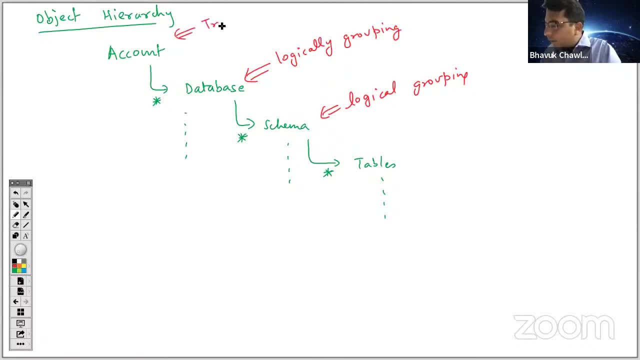 of schema. so there is one account that we are having right now we are using trial account in snowflake and that is in us west region, yeah, and then we have tables and views and everything. so this is a hierarchy. so you'll see, like we created one account and then within that we can. 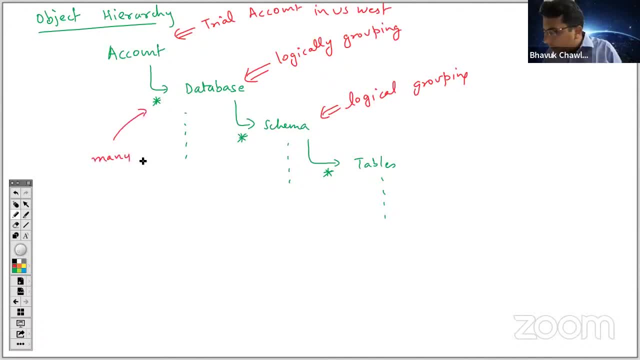 create databases. so. So star means many, Yeah, so you can have in one account many databases. In one database you can have many schemas, And in one schema you can have many tables, right? So there are other objects also, But I'm just sharing with you. this is a structure that you will experience when you're working. 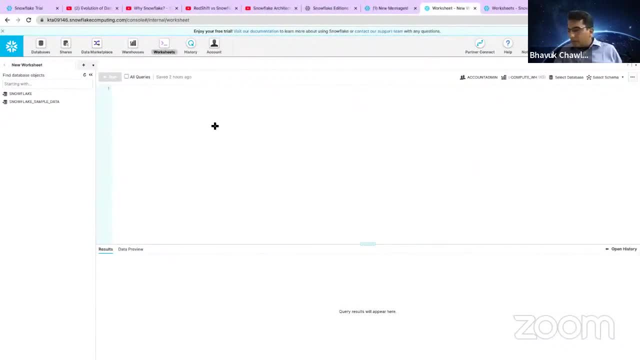 with Snowflake. So, coming back here, when you open this console, the classic console, and there you will see we have databases. So these databases, you can always create database through user interface. So whatever you can do through command line can be like whatever you can do through user. 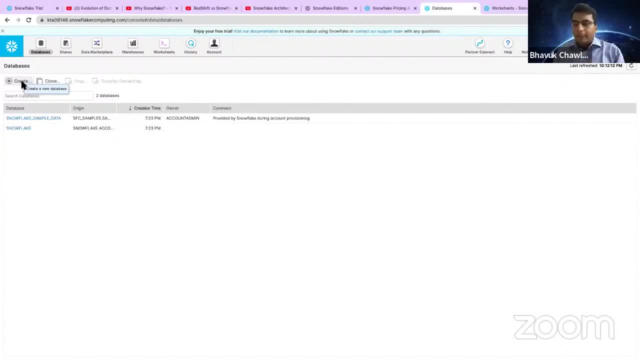 interface can be done through command line. So you can do it through command line, But it is not other way around. It may be possible that you will find the user interface is not having all the options which are available in command line, So command line is much more powerful compared to the user interface, right? 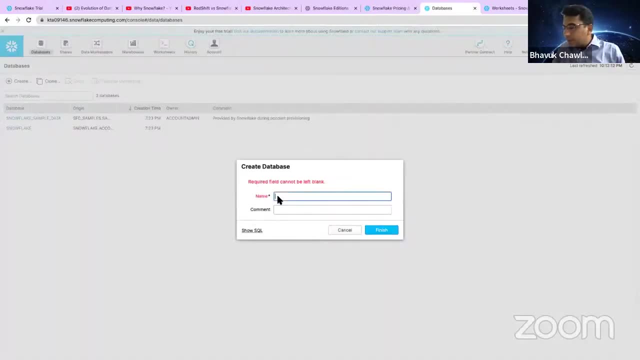 So when you say I want to create a database, you can even see the script. So let's say I'm creating a database demo, right, And I just give Any comment, and then you can see the SQL also. create database demo? and then you can. 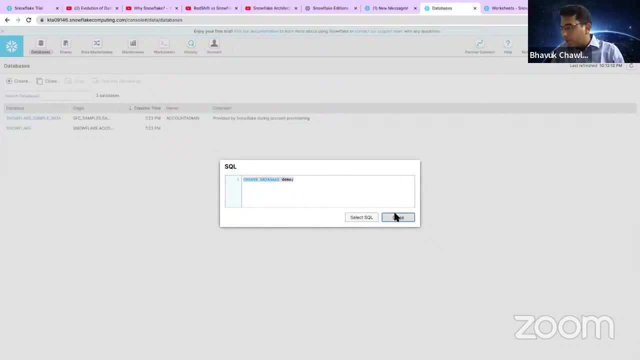 say that I am actually executing, So select SQL or whatever you want to do. So you are. you are creating a database. So you just created one database and you will see the owner is account admin. This is not a good way to create a database, because we should not be creating databases. 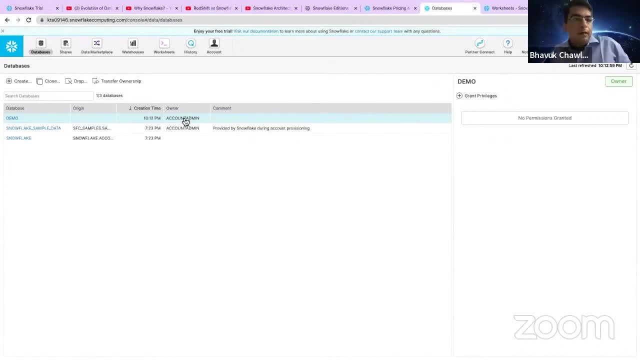 through account admin. It should be done through custom roles, ideally, but since it is a very quick demo, so that's why I'm just showing you that we are in a particular role And we can see, uh, the owner the through. through this owner, we are creating a database. 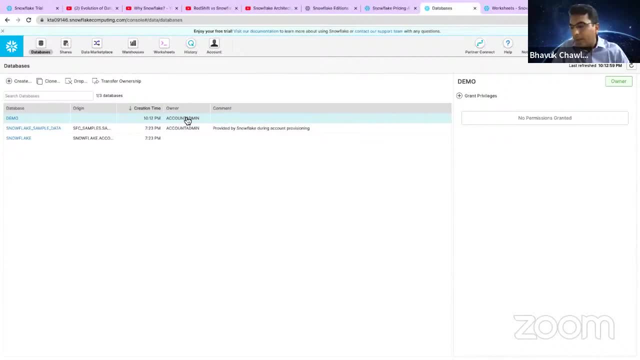 So the object owner is that particular role. right Account admin is the owner for that particular role. But if you switch your role to some other role then you can see the owner will change when you create that object. So by default, when you create any object in Snowflake the owner is the role that is. 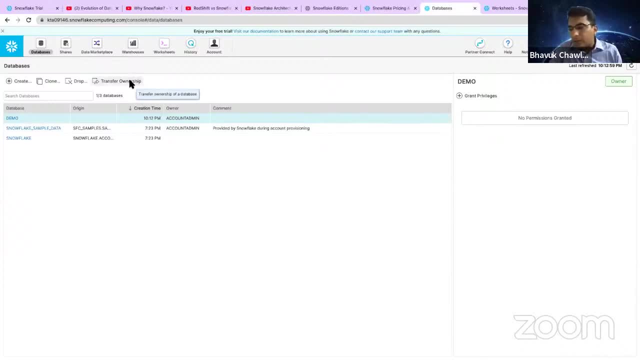 creating that object by default. So you can transfer this ownership to some other role also. but uh, will not go there. We can have a separate session on Snowflake security. We can talk about the custom roles and everything. So in practice, in production, you will be creating your custom roles. 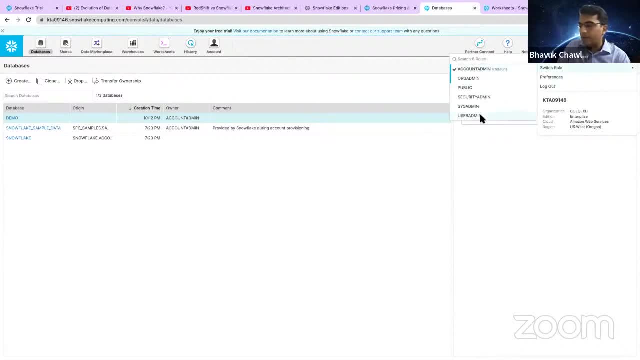 You will not be working with default roles available. So these are the default roles available in Snowflake, but you will be creating your own custom roles, For example, in terms of joining your company. you will be creating roles for interns. Let's say you have some training going on. 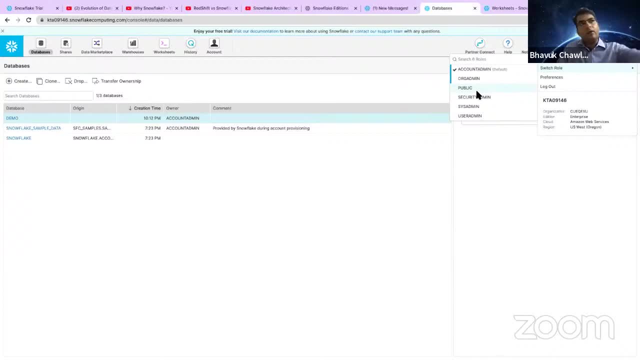 So maybe you will create a role for training? Yeah, So you can. you, let's say, you are having a like um an auditor role, or you can create multiple roles here, um custom roles, And you can. 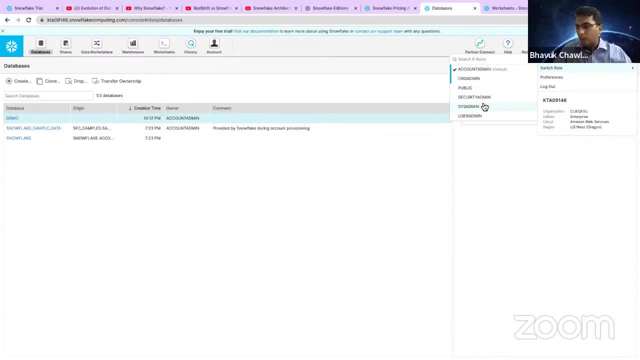 Assign privileges- we have fine grained privileges to those roles. So now this is like way one, way to create database. There are um, like other things also, but you know we are talking about account admin. This is the highest role. 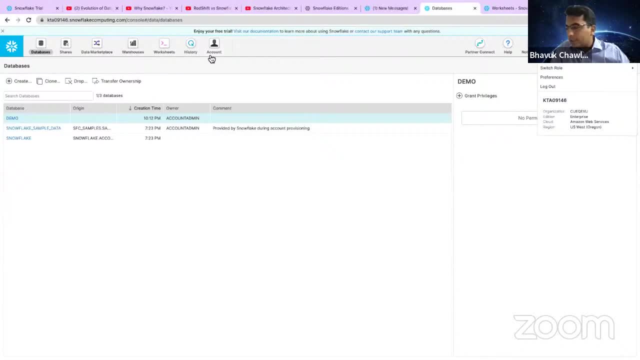 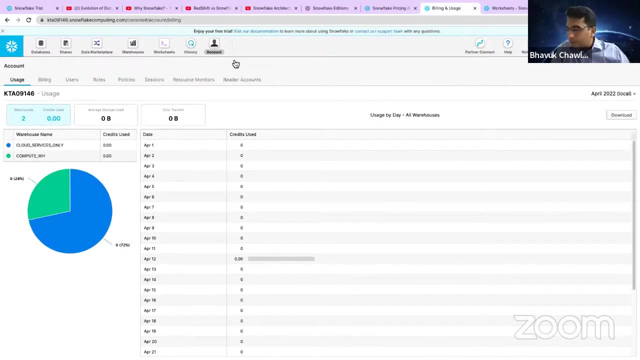 So when you are using account admin role in Snowflake, you will see there is an account tab available. So this account tab is available only when you are account admin. So when you are account admin, then account tab is available And within that you can see the usage. 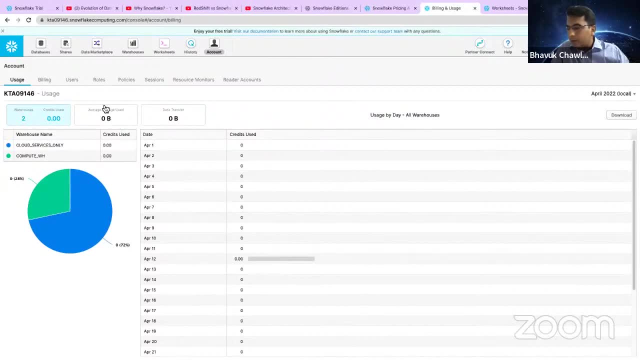 You can see how much usage we are having on each day, how much data we are storing- average stored storage, how much data transfer we are making. Let's say you are having a setup where we are having a prod and DR setup and you're 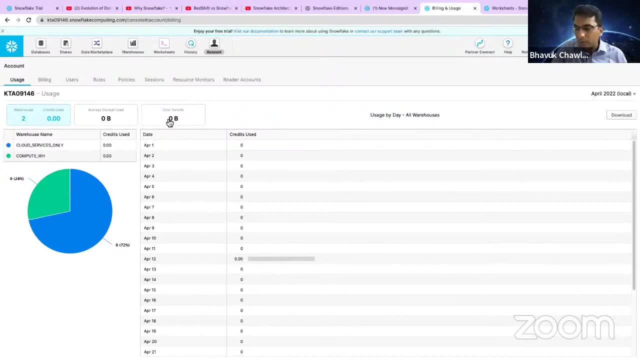 transferring data from one region to another region. So there will be data transfer charges also. So you can see like how much credits, how many credits we have spent, like how many credits we have used. So you can see this information also on the Snowflake and then you can see the billing. 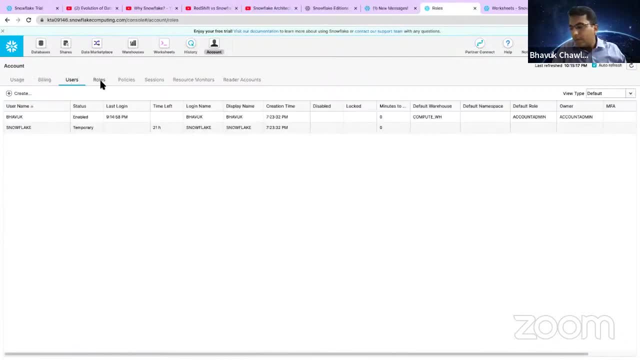 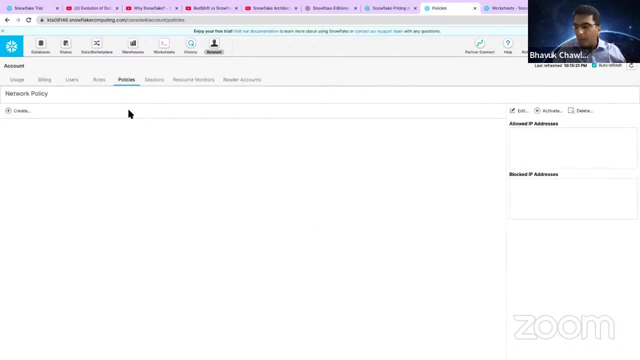 Uh, you can see the users, You can see the roles that we are having, You can see the policies. You can blacklist some IP addresses, You can um define network policies, You can define user policy. So all these things can be done. 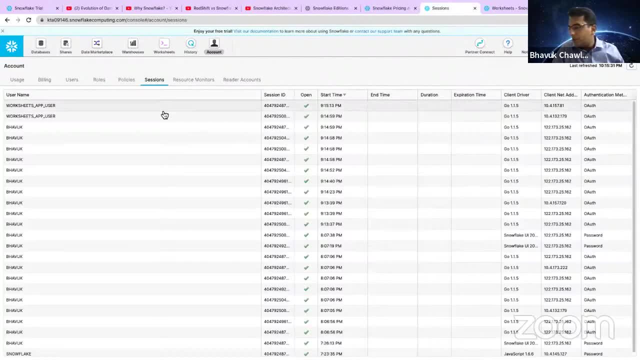 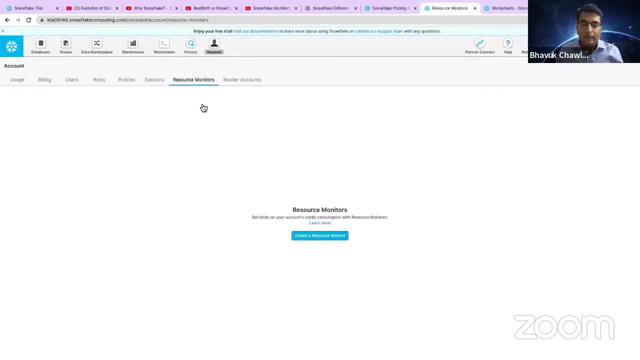 Um, and then we have sessions, which all sessions are going on. Yeah, So you can see that. and then resource monitors, So you can set up quotas, You can set up alerts. Let's say you don't want data science team to use the warehouse. so many credits. 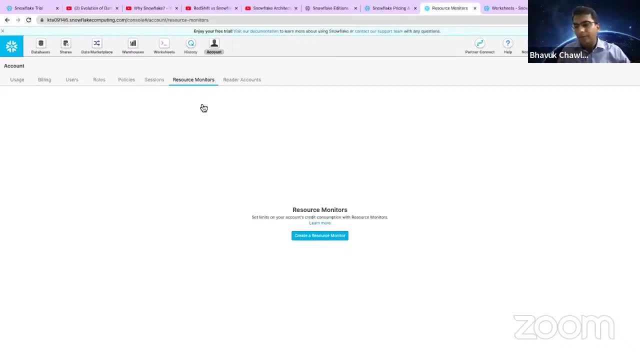 So you you can set up alerts at the warehouse level, You can set up alerts at the account level So Resource monitors can be set up. and then we have reader account. through the reader account, You can share data with those people who are not even Snowflake customers. 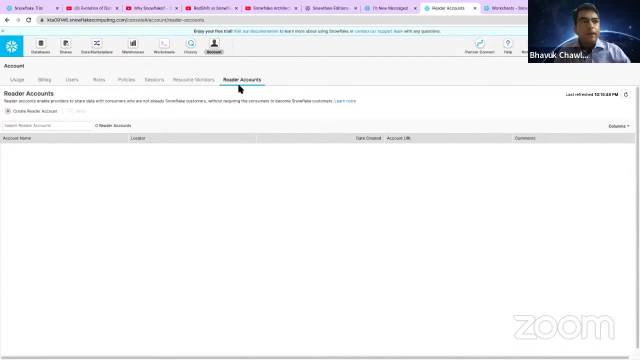 So you can have a, like a reader account through which, like, let's say, my um, let's say, I'm working with another company which is not a Snowflake customer, So you want to share data with that company. It's possible to do that. 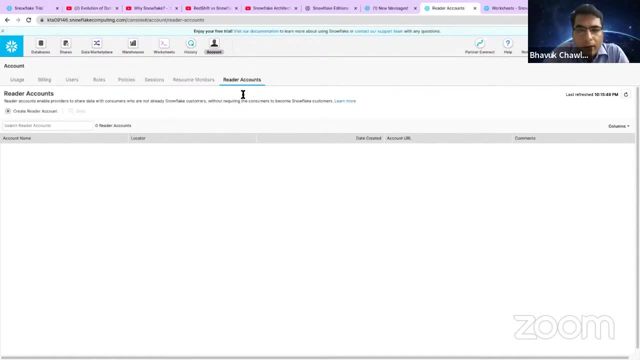 Yeah, So there is a question now. uh, can you please send out the Snowflake playground ring? So I hope you got it like the Snowflake. You can set up a trial Account and you can easily work with that. There is another question. 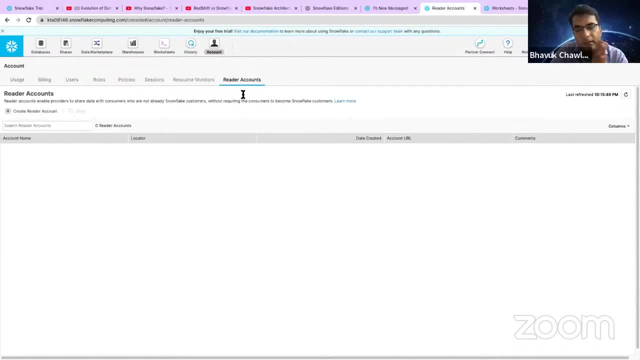 Are there tools to make an easy migration ingestion from data? Yes, So there are tools through which you can migrate to Snowflake and you will find there are white papers available. Um the Snowflake website itself community, you will find a lot of discussions on migrations. 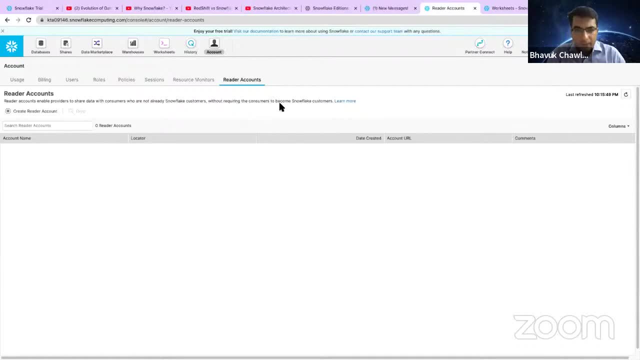 So these are available, And even there are tools available which will. the third party tools are available which enable you to migrate data from Teradata and Netiza. So this is very common. Um, just one thing, Uh, someone else. 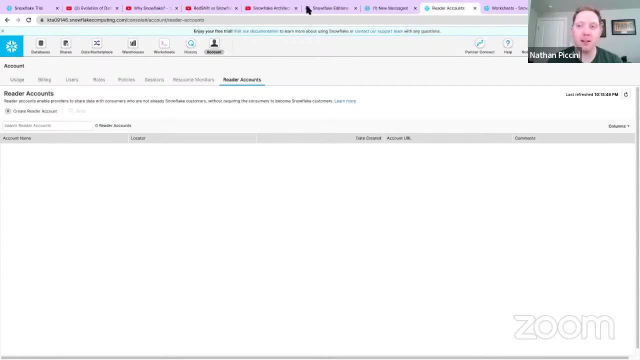 Is asking: uh, while registering, which cloud provider should they select? Is there Okay? Okay, So I choose AWS. Um, it's like it's fine, You can choose anyone. um, because right now we are focusing on core capability of uh Snowflake. 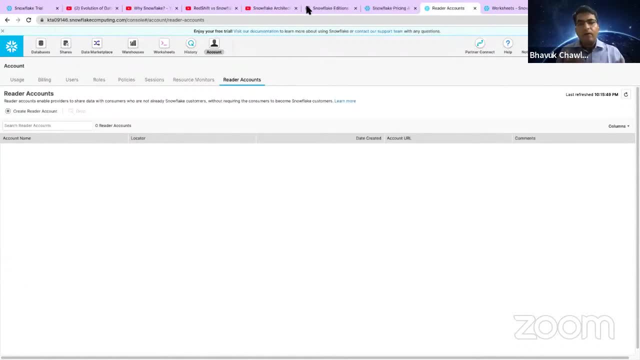 We are not integrating Snowflake with the external stage, or we are not integrating with some streaming pipeline in the cloud provider. So, uh, in case, like uh, you just want to get started, you can choose any. it hardly matters because it's, like uh, agnostic as such. 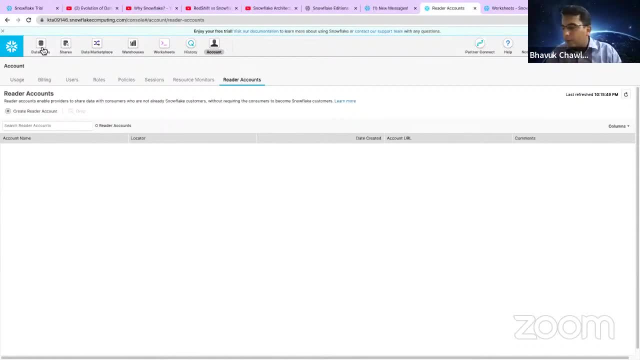 But specific places you will find, like when you are, when you are going to the stage, let's say, uh, then you will see the cloud provider related options will come. So let's say I'm within that. So if you are going to stage, then if you are creating a stage. I know I did not explain what is the stage. 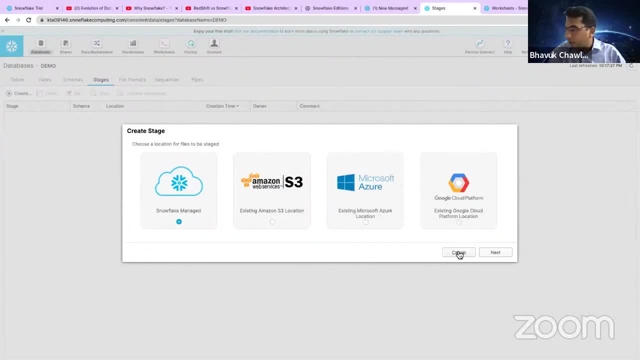 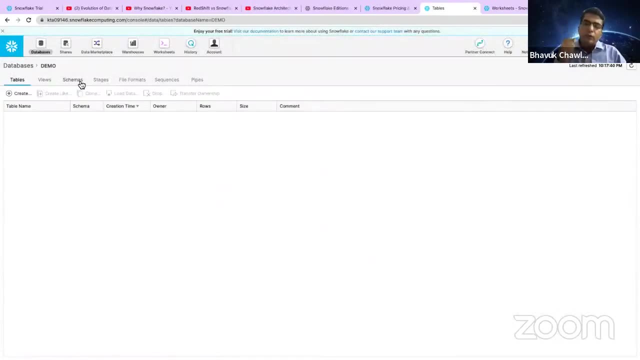 Then the cloud provider specific things will come, but we will not be going into that, since you are just getting started, So it will hardly matter. Yeah, So you can just choose any cloud provider. You've just choose a region which is closest to you, right? 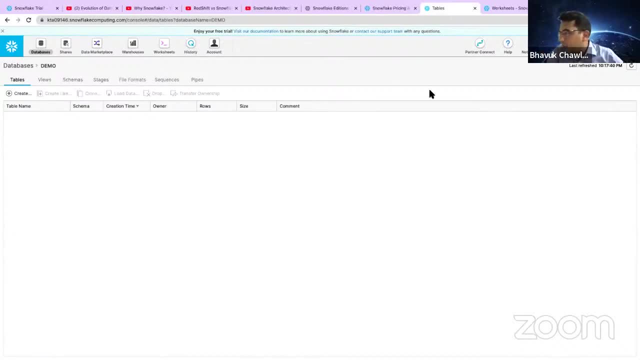 So that will be easier. Uh, so I, uh, I choose AWS right now. uh, but it's fine, You can choose any cloud provider to work with Snowflake, because it's all under the hood. You will not even see unless or until you integrate. start integrating, uh, with the, uh, the, the, the, S, S, Q, S, or like you are building such event based notification. 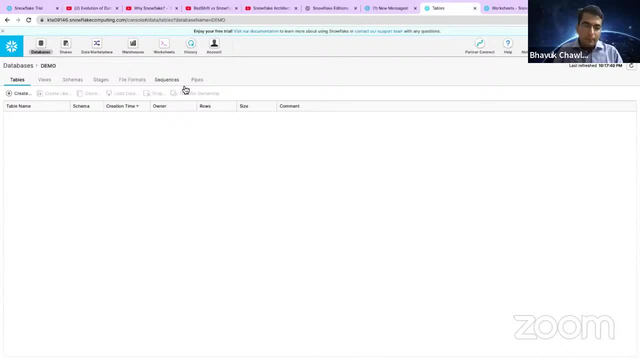 And then you are ingesting your time to Snowflake. You are not building those pipelines right now, but if you are building those things then you can choose the cloud provider where you you think that data will be arriving from some other ETL job, let's say, spark or some other um application is writing data to some external state, some S3 bucket, and then you can choose that specific cloud provider. 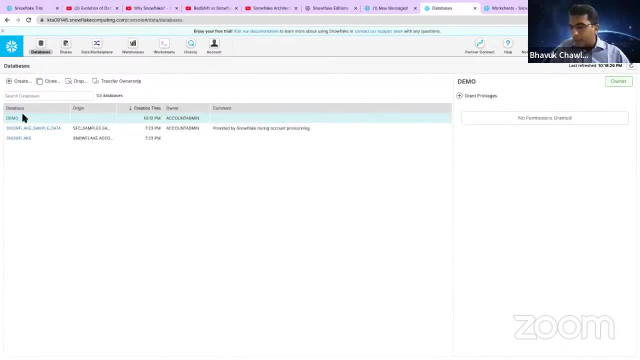 But it's fine for this demo. So we are talking about them like this database demo and I hope everyone got it Like, uh, this, this is one way. Um, so we can go to the worksheet where we can write queries. 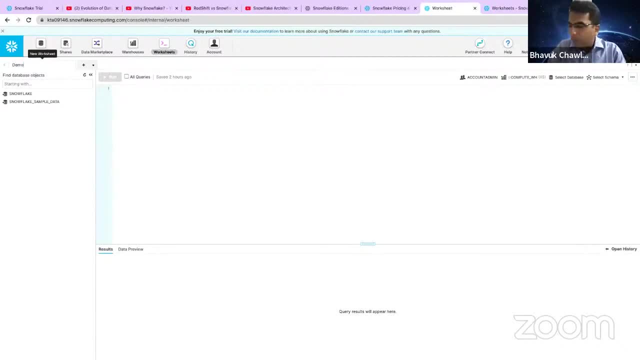 So can you see there is a name which is called new worksheet. So I'm just giving demo or the meter. Okay, So I'm just giving a name: Demo for meter. Um yeah, so this is like: uh, yes, 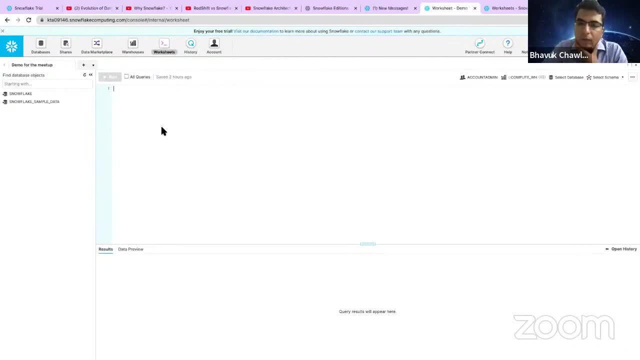 So for deep dive, you can um, you can read the documentation, you can watch the videos And also there are some blogs which we have published, like change data capture blog, So you can follow our LinkedIn page there. We published a lot of interesting things on a snowflake. 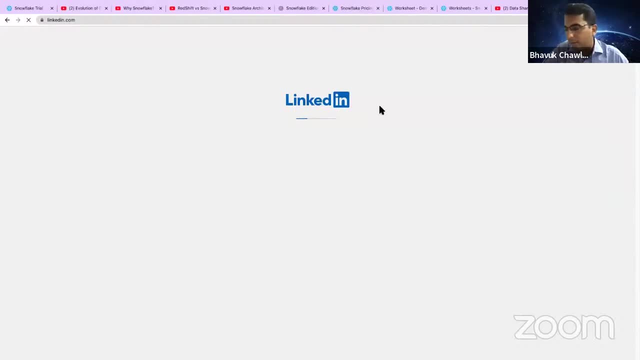 Like: uh, there are a lot of articles and blogs that we have published. So, in case you are interested, you can just go to the LinkedIn- Uh there, Uh, LinkedIn- page, where we share a lot of information. So let it load. 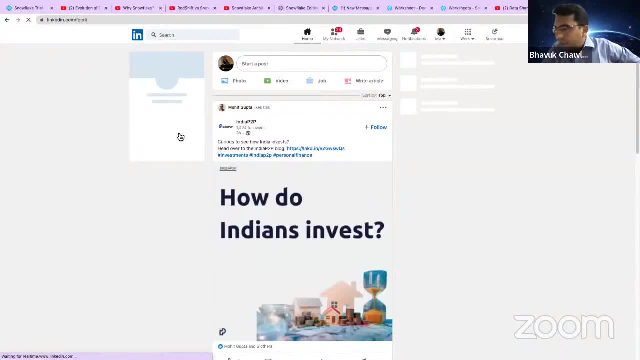 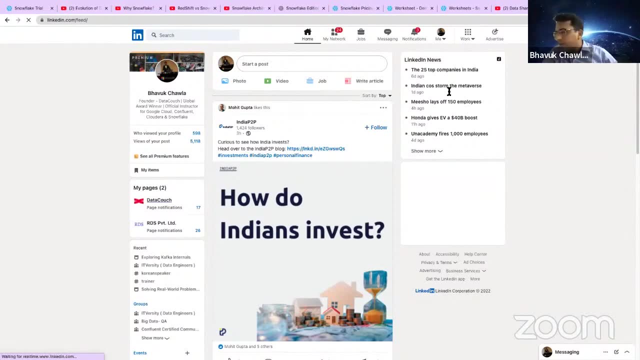 It is taking some time. So after that, you can just go to data couch main page- this one- and where you will find um, we share blogs also related to something. Okay, So, coming back to this, you can follow those blogs. 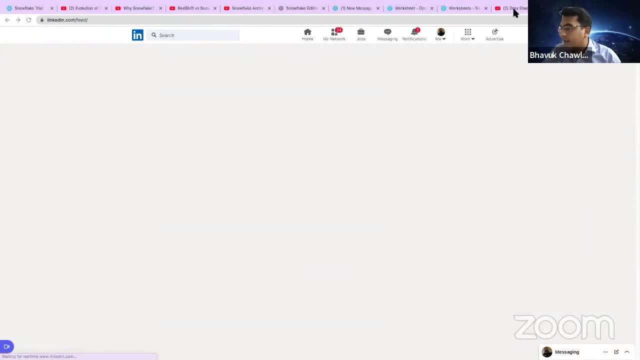 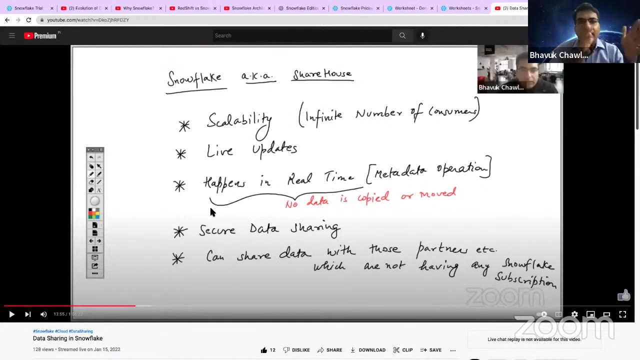 You can implement change data capture. some interesting use cases on snowflake. And then I have a video on snowflake, which is a snowflake share house. Uh, this is one hour video. This is like a dedicated topic. Uh, you know, share sharing data in snowflake- how it works. 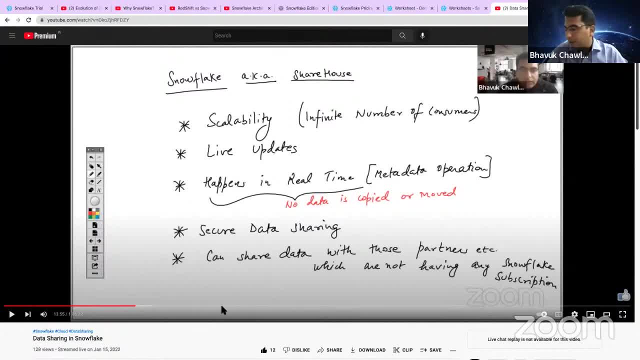 So here I have done a lot of hands-on also and here I have explained uh what is secure data sharing and how does it work. So I would encourage you to um uh go through these videos also on our YouTube channel related to snowflake. 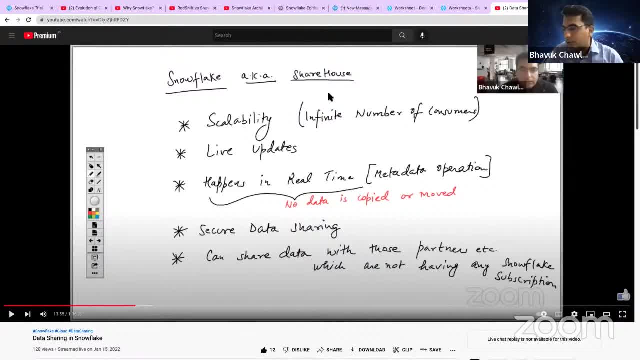 Um, this is one share sharing, data sharing, and snowflake is also called share house. We'll find how, how to work with that. Okay, Coming back to this, uh, uh, coming back to the worksheet. So we were here. 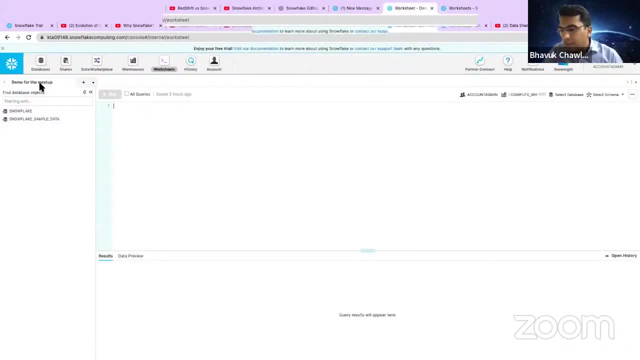 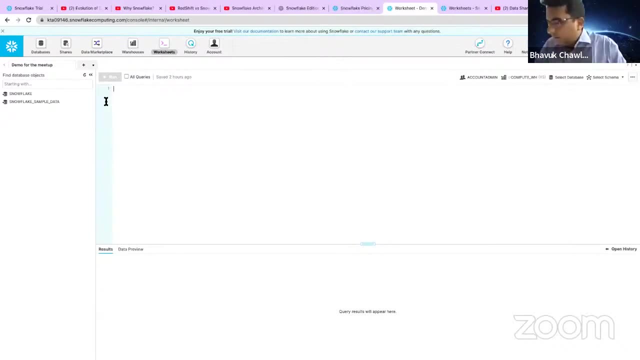 In the worksheet we can write queries. Yeah, So I just renamed this worksheet. You can have another worksheet, Um, so when you type anything here, so then uh, it will basically uh be able to retrieve results from the snowflake database. 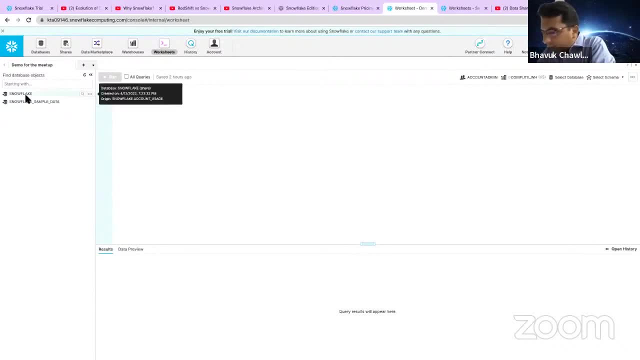 So can you see, um, I don't, I don't have the demo database here, because the demo database was created through account admin. Yeah, So I can, I can specify. let's say, um, I have, uh, um, let's say, I want to fire a query. 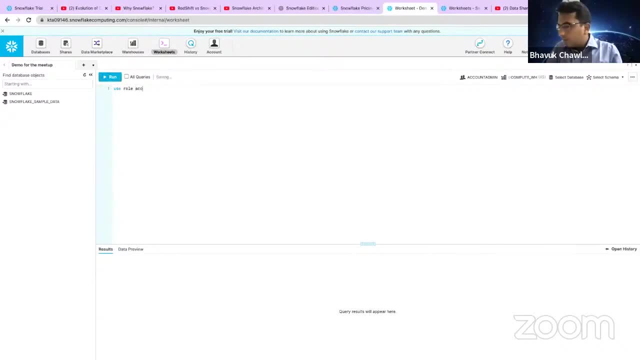 So let's say we have Use role: Yeah, So I can specify this. I can say that I want to use a role- account admin. Yeah, And I can refresh this. Yeah, And here I see demo is here. Um, but if I change my role, then I will not be able to see demo. 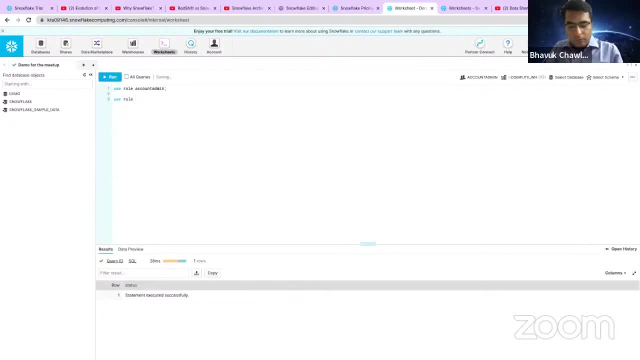 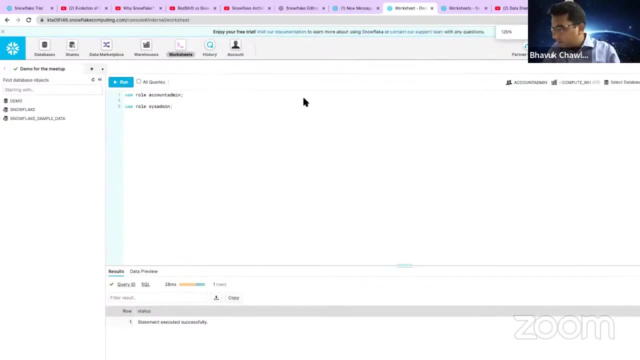 So if I say use role and I want to, let's say, admin, I'm changing my role. Maybe the font is very small. I can make it bigger so that you can see better. So I hope this is now legible. So maybe 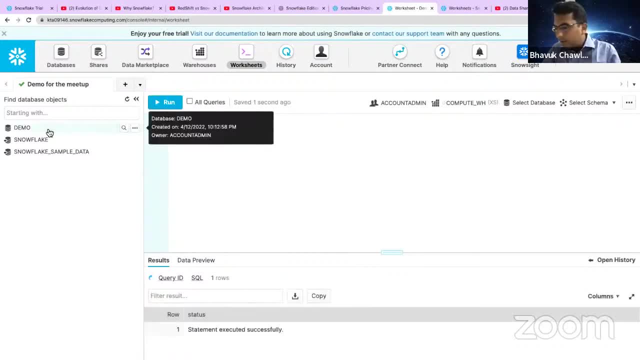 So when I change my role to sysadmin then I will not be able to see. I will refresh, So I changed my role. I don't see demo because the demo database was created through account admin. So it is very important. Some objects will not be visible to you because your role is different. 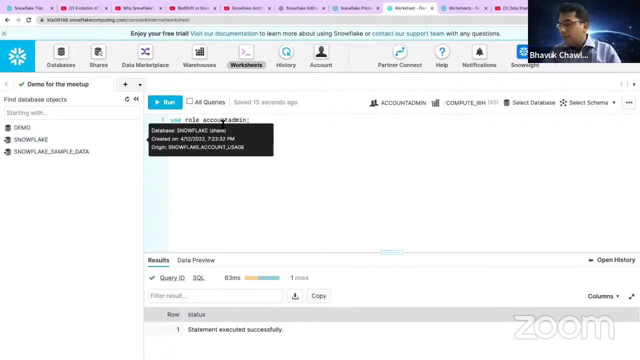 So you should use the right role so that the objects are visible. but creating objects through account admin is not a good idea. Yeah, But I'm just showing you how the default roles are and how the object owners can see the roles, unless or until you grant. 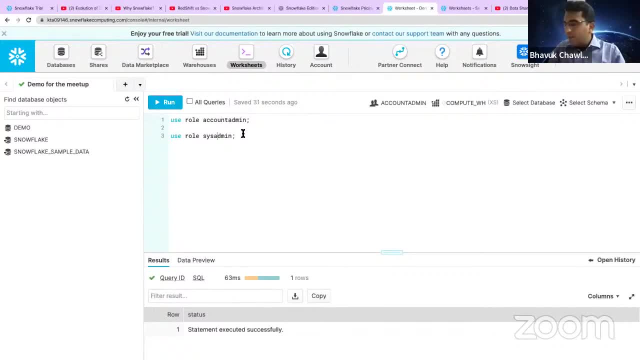 Permissions to that particular object. So let's say, I'm going back to sysadmin and, um, uh, this is like I'm going back to account admin. I want to compare a few things here before we go into the sysadmin. 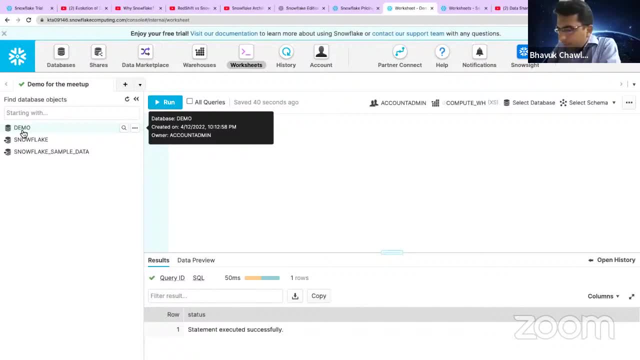 So let's say I'm here, You will see, there is demo database and then we have snowflakes, snowflake sample data. So what exactly it is. So can you see? the icon for this database is different from this database. this database. 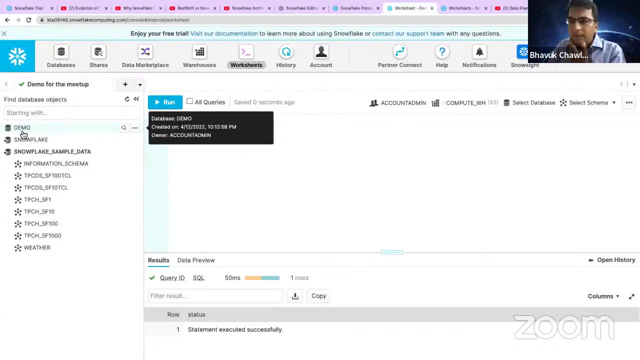 I created myself demo database. I created myself in this step in this meeting, Uh, but these two are uh sharing, like the data sharing. This is these are shares, right? So these are, these are shares. And uh, these these are shared by someone else. 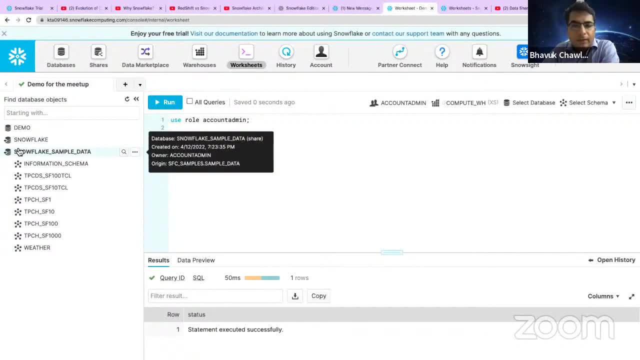 So this is shared by snowflake. It is part of the account setup. When I set up my account, like when I get my trial account, I got, I get these uh databases, these shares, And can you see, if I do mouse over this tool tip shows me that this is a share in bracket. 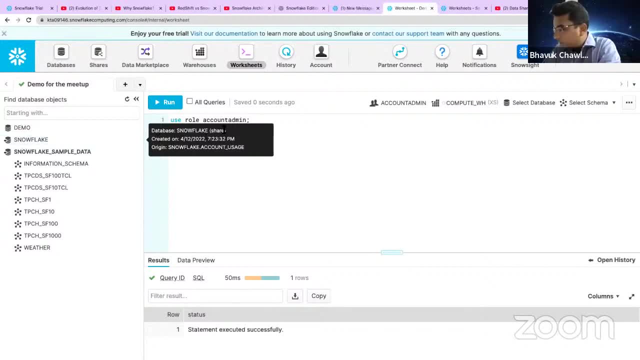 If you notice there is a bracket, if I go to that bracket, then the stool to people. Okay, Okay, No, No, it's there. You can see, this is a share. So when I do mouse over and you see a tool tip and there is a share written, that means that it is clearly communicating you that this is a shared database. 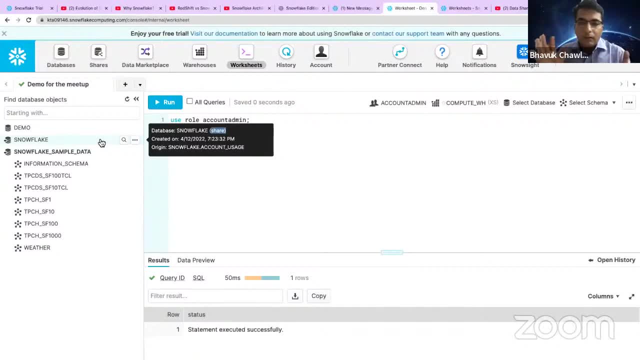 This database is not owned by you. You are not paying the cost of storage. It is like from snowflake. right now It's part of the account set up, So you will be paying for the queries that you are running. So right now you are. when you fire the query, then you will be paying for the query runtime cost. 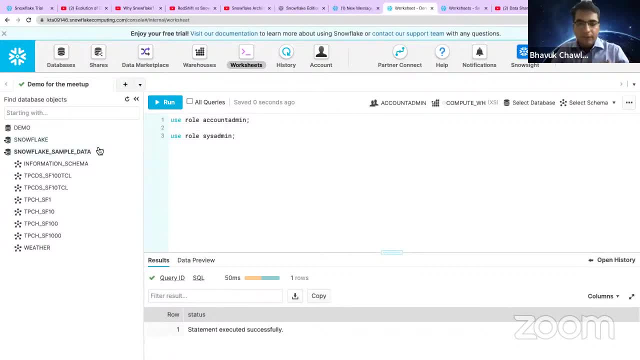 You are not paying for the storage that you are having. So this is that. That's the difference between a shared data as a or like when you are owning your own database. So this is your. you are paying for the storage and you are paying for the queries that you are running here, but here you are paying only for the queries that you are running, because data is being shared by someone else. 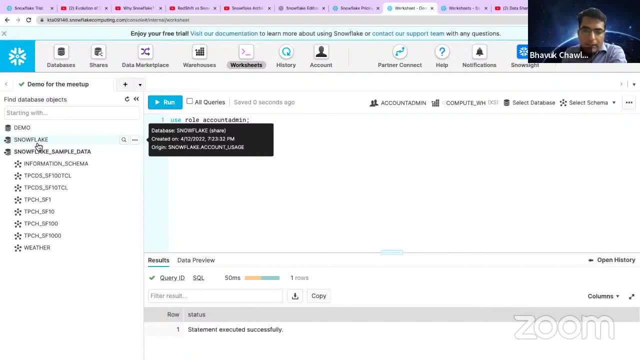 Yeah, Okay, So you talked about roles, account admin, and there is a question. I'm reading that question. So so, ideally, data warehouse solution requires involvement of more than one person. Absolutely, There are many roles in a data warehouse, so there will be database administrator. 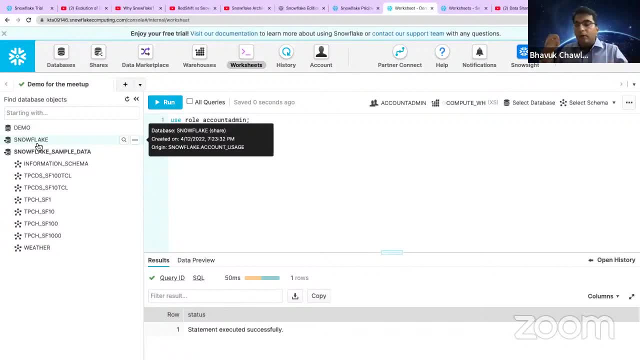 There will be, like, people from Data warehousing team or maybe a reporting team, There are people from business intelligence or maybe there are people from a data science team. So there will be different roles in different different teams. Like, you can have a hierarchical structure and you can create your own um, like role based access control, and you can- you can have your own custom roles. 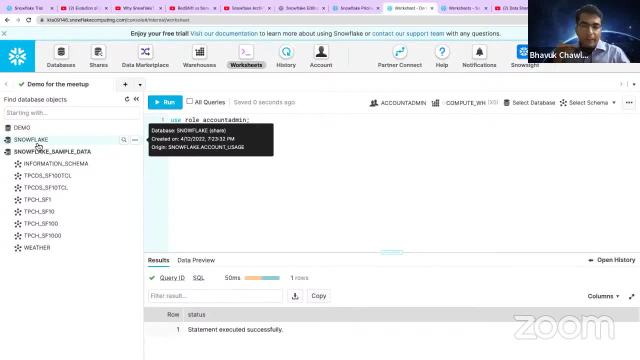 Yeah, So single person will not be doing everything in snowflake. There will be um like, depending on your responsibilities. some people are only auditors. They have only view, only access. They cannot modify Anything right. So some people have ability to drop tables, right. 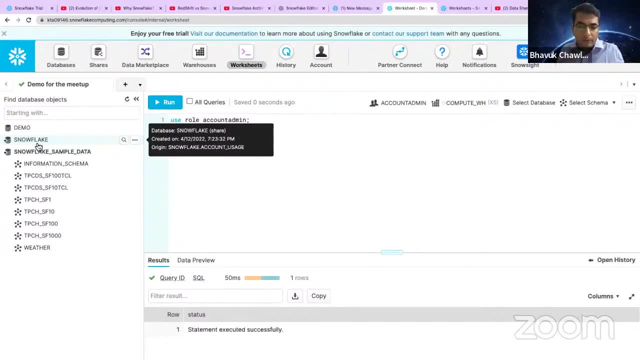 So some people don't have- like a lot of people they don't have- ability to drop tables right. So depending on role, it will vary, gently. So how secure is snowflake? So that's a good question. Uh, so I would encourage you to. uh, there is a white paper on snowflake security. 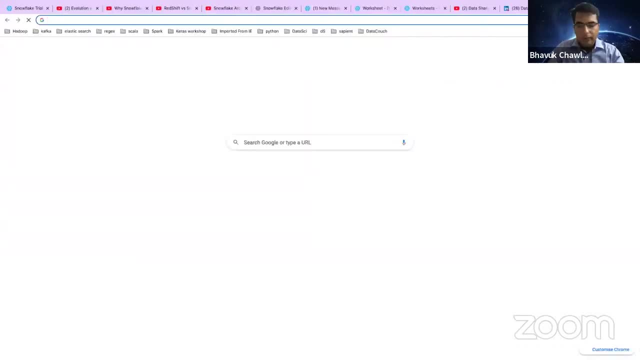 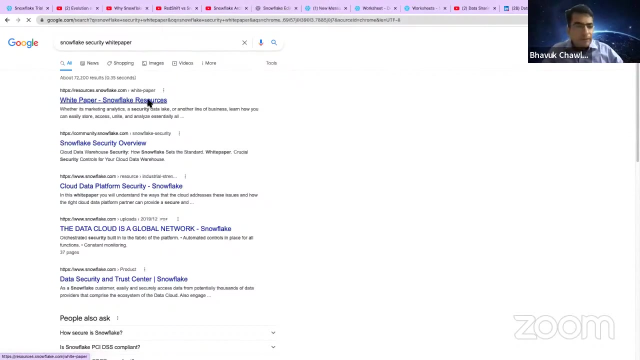 I would encourage you to go through that white paper- snowflake security white paper- just Google- You'll find very interesting um like some interesting aspects are given How keys are managed. So if you go to this white paper- and there are so many white papers not I'm answering this question in a more generic manner so that you get answers to a hundred other portions, not just about snowflake security. 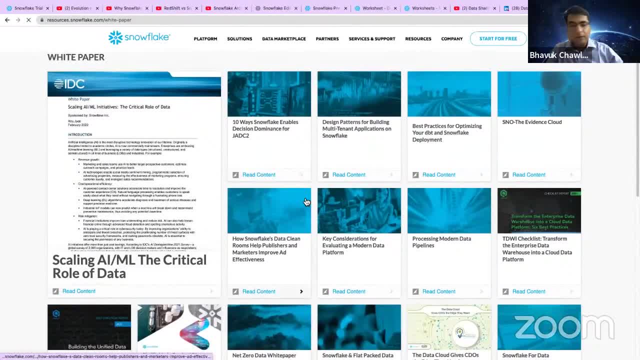 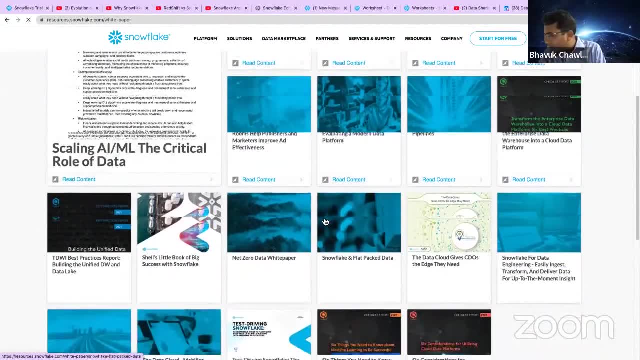 So if you go here, you will find there are interesting white papers. one white paper, very, which is very interesting is, uh, semi-structured data. You must read that. And then, uh, there is a white paper on snowflake security and there is a white paper on data cloud. 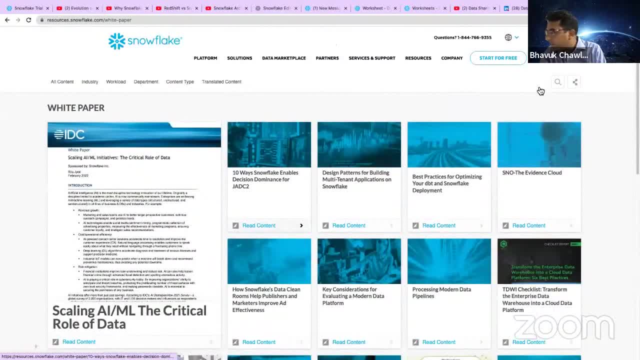 So you'll find there are different, different white papers. So just search for this white paper, You'll find: Uh, there is a white paper on security and there is a summary, very nice summary given about security. So I would encourage you to read that white paper. 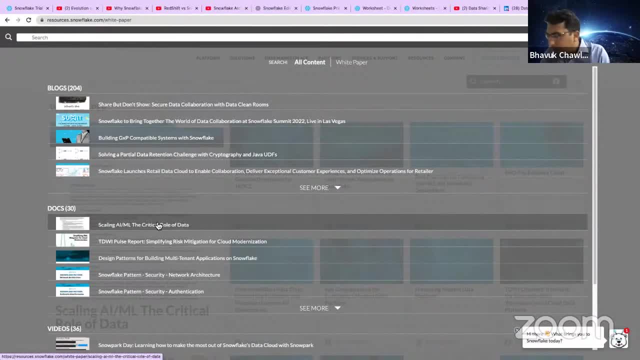 And second thing is like, once you read that white paper, there is like a white paper on security. Uh, you can search here. if you are not able to find it, just ping me on LinkedIn. I will send you the link. So, uh, apart from that, from security perspective, you can see if you go to the um, various additions. 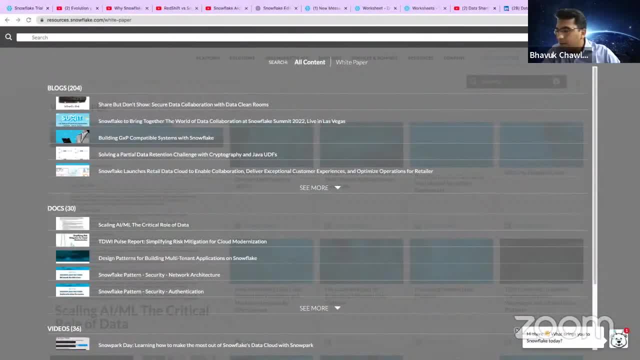 So I will show you the additions of snowflake. I want to show you the additions of snowflake there. Um, let's say I opened those additions. Yes, This is the additions of snowflake. Okay, So let me go inside this. additions of snowflake. 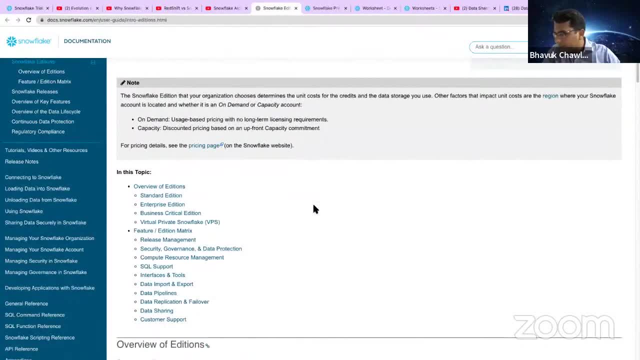 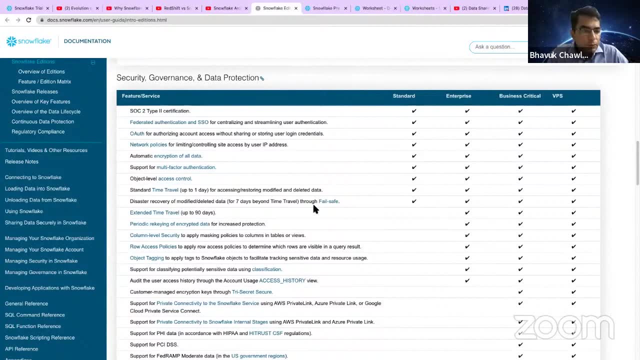 Okay, So when you go, once you go inside the additions of snowflake, you will see there is a comparison and there is a comparison with regards to various security and governance data protection features. So, Joshua, so in case you are interested to know about security, I would encourage you to please go through. 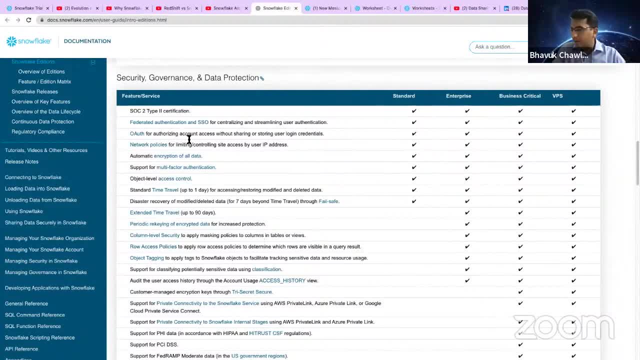 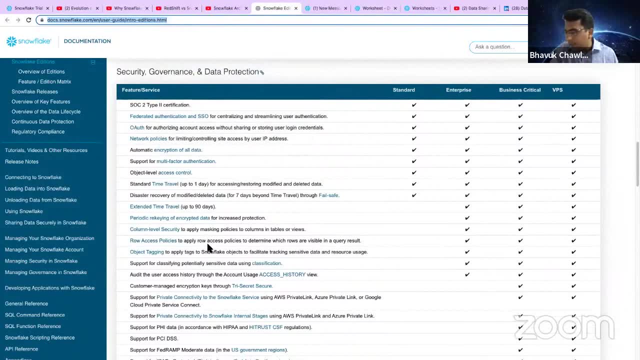 The white paper and also refer to this particular um, particular uh documentation. So I'm just sending this link over the chat where you can see um, the PCI, support for PCI, support for PHI. Yeah, So a lot of banks and a lot of companies are using you can see, in case you are interested to know, let's say whatever domain you're working, let's say you're working in banking domain. 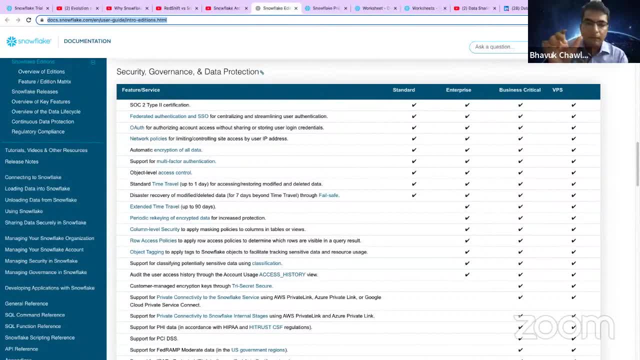 You go to snowflake website, go to case studies: filter based on the domain that you are interested in and then you will see which all banks have implemented snowflake- All right. Which all telecom customers have implemented snowflake already. Yeah, So you will find a lot of interesting details on the case studies page- success stories. 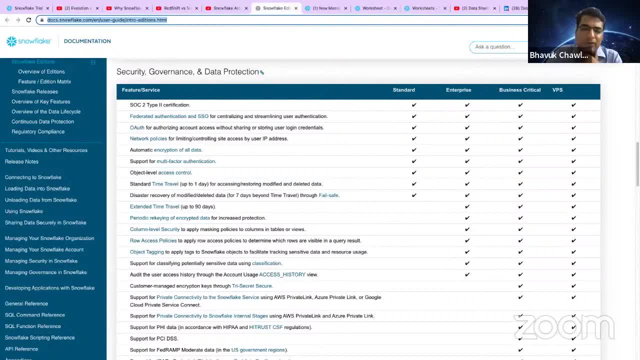 Is it correct to say snowflake is a cloud version of system? Like no, no, no, actually Oracle also has a cloud offering. So you know, a lot of traditional data warehouses like second generation, third generation data warehouses, tried to bring their cloud offering, but snowflake is a technology which is built from scratch. that is, cloud native technology and the patented nature. 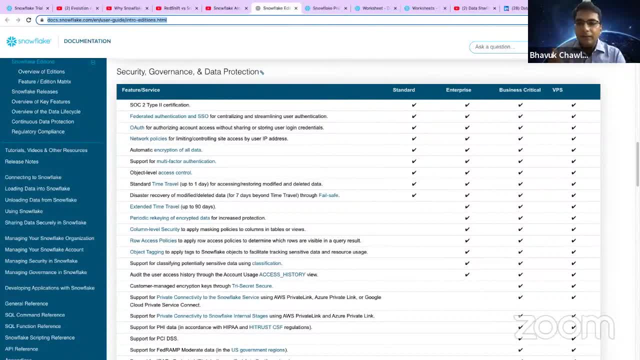 Like you know the way it stores the data: it's in FDN files. FDN stands for like it's. it's a FDN is basically French name of snowflake, Like if you search snowflake in French, then you will get FDN, something like that. 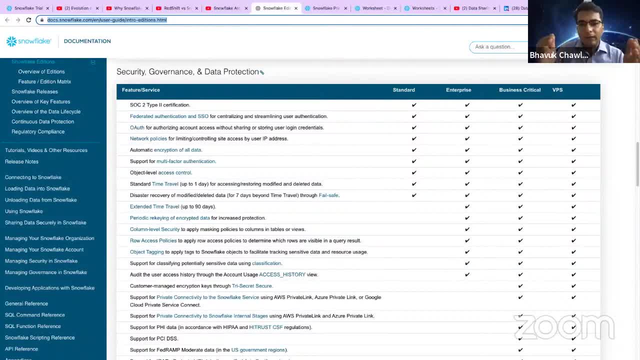 I'm not expert of French, but I'm just thinking aloud. like snowflake is basically like FDN format. This is a data like format or this is a file format that we are having. It's a columnar format and it's a patented technology of snowflake. 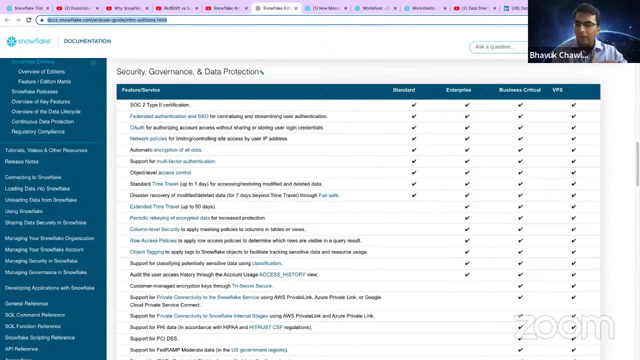 So it's something. It's just very much different from cloud offerings of other data warehouses that we are having. So it's built from scratch and it's not something it is adding the features later on. It is built from scratch and it is incorporating all the best practices that one data warehouse should have. 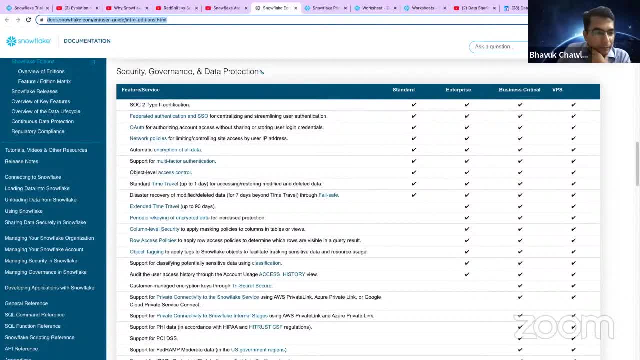 Modern data warehouse should have. Yeah, Yeah, Very good, Thank you. So I'm coming back here. So we have so many things to cover. Is it okay, Like Nathan, if we extend this session? Yeah, I mean, you want to keep going. if you have time, feel free. 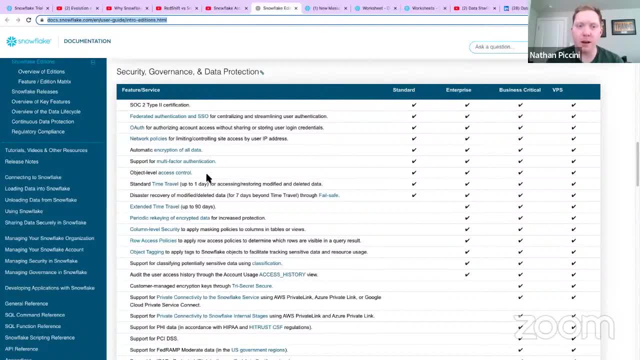 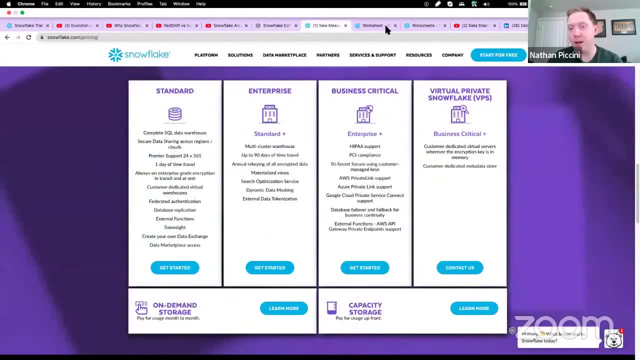 Just want to let everyone know we've opened up the certificate form, So if if that's something you're looking to receive and you need to drop off, please fill that out. But, Pavuk, if you want to continue, please feel free to. 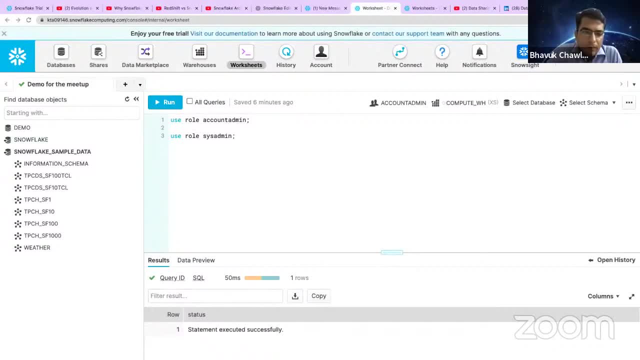 Sure, Sure. Thank you so much. So, if you are looking at this, I would focus primarily on demo right now. Yeah, So that you get a lot of value out of your participation here. So we see that we are able to. 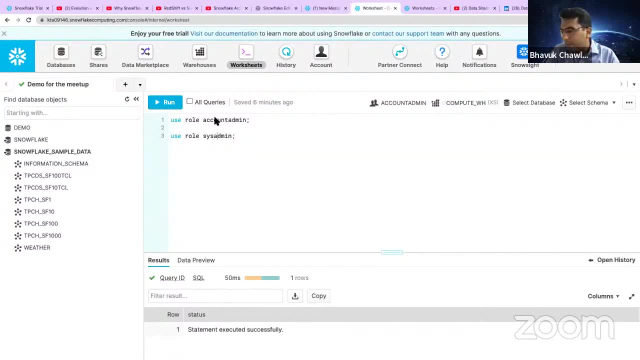 We are able to switch the role to account admin, sysadmin, and then you can see I'm using account admin and I see a different set of objects now within that. you can say I want to use the database, Yeah. So I can say I want to use Snowflake. 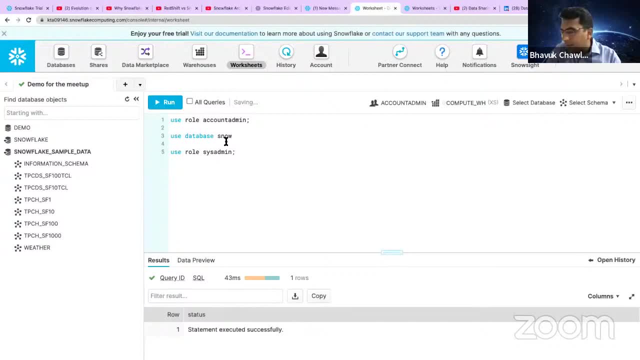 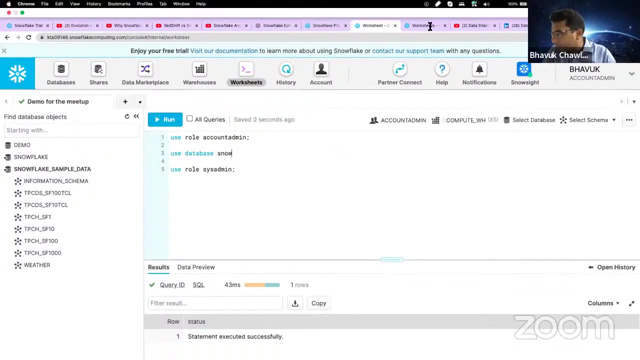 So can you see there is no type, like there is no search suggestion, or you can say typing: There are no hints coming here. but then when I switched to the new interface, when you log into Snowflake you will see this is a new interface and you can create a worksheet here. 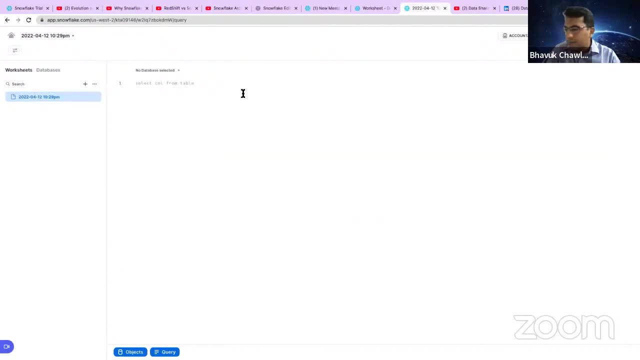 So within that, when you are working with this new interface, then you can say use database and then you can say Snowflake sample data. I want to use that. Yeah, Can you see? now hints are coming when you are typing. So this is a new, this is a beauty of new interface. 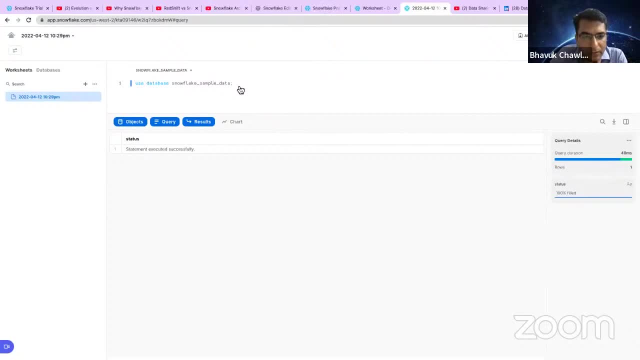 Yeah, So there is a question on um. is it correct to say that, uh, Snowflake work is fine and something? provide data modeling. Okay, There is a question on data modeling, So provide data modeling to. okay, very good. 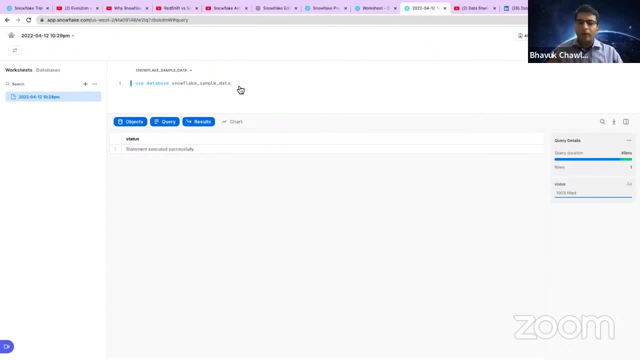 So Snowflake is a platform which gives you ability to model In your own way, So it is not giving any best practices to do data modeling in a certain manner. You can do data modeling in your own way, the way you do it in other data warehouses. you can do it on Snowflake. 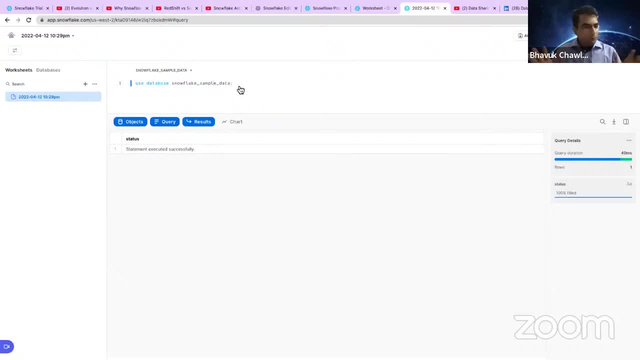 So if you search on Snowflake documentation anywhere, you will not find anything related to data modeling, because it's a platform which is a modern platform, which is giving you high performance and, like uh, reducing your cost and overall, the cloud benefits, the elasticity. 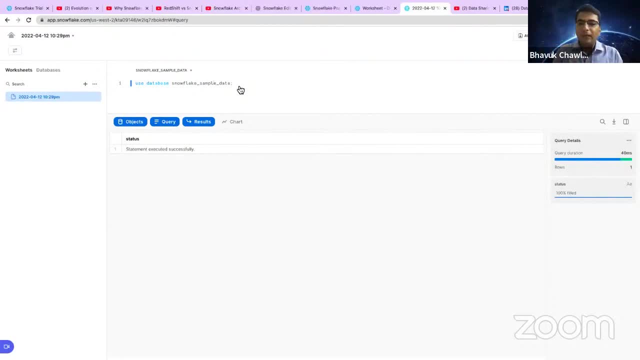 scalability and many other things. So it is not giving any recommendations. So it is not giving any recommendations related to data modeling. So you can do that. And there is another question: Can you perform ETL in it? Yes, we can do ETL in it, but primarily it is a data warehouse. but it does provide ability to perform transformations. 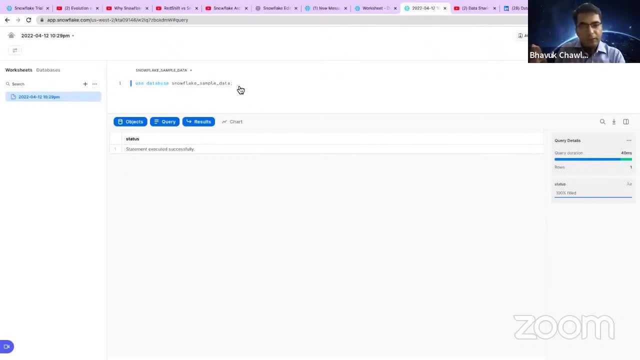 So you can perform transformations in Snowflake through stored procedures, through user defined functions. You can perform transformations in Snowflake through um. maybe you can write your Spark queries. through Spark connector You can connect with Snowflake. You can do transformations through streams and tasks- also right tasks you can schedule, and through streams 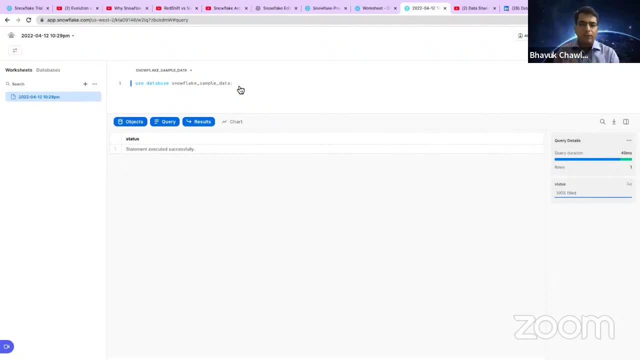 You can perform that. Okay, So you can perform transformations. There are many ways through which transformations can be done and you can extract data from raw table to a process table. You can do that. Like ETL, can be performed, but some companies they prefer to have a dedicated ETL tools like, specifically, you have talent or Informatica. 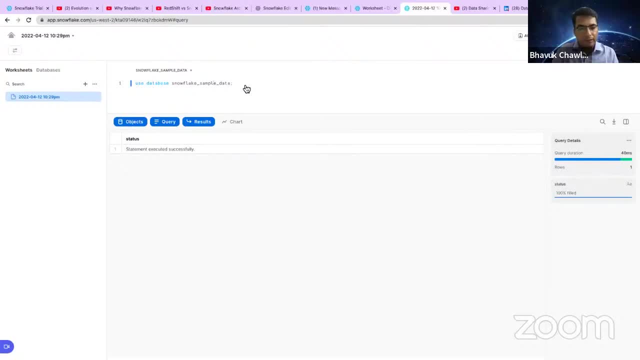 You can integrate those tools also with your data warehousing solution like Snowflake. that is also possible. So, coming back here, so you can see when I'm running the query, I'm able to switch the database and I can use the particular schema. 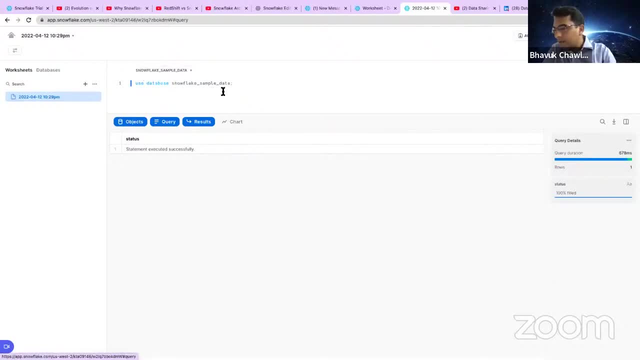 I'm having and this is my home, I can go back. So the beauty here is, when I run my queries, I can see that when I run this query, this is used database And then I say: use this. then this is like use schema. 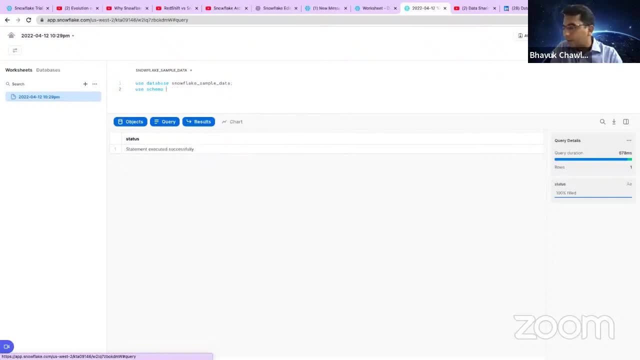 Yeah. And then I'm saying let's say I want which schemas we are having. So I can even see this is one schema, This is another schema. So these are different schemas that I'm having. So let's say I have this schema. 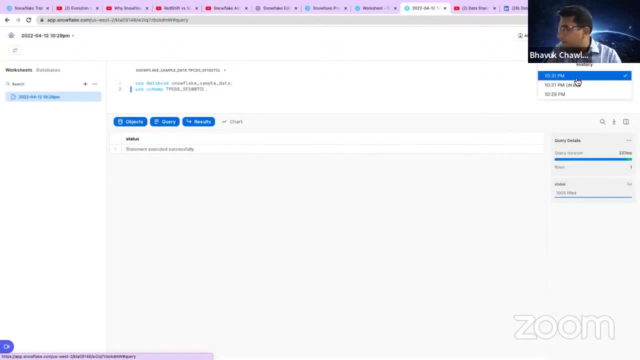 So I'm choosing this. Okay, So let's say, I have this schema when I'm executing. so can you see we have three versions. Yeah, So whenever I execute any query, then there is a new version which is created. 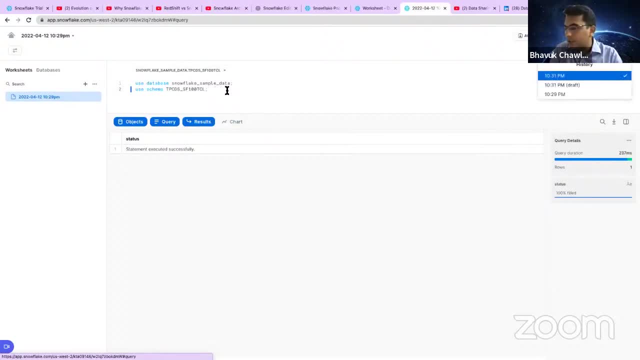 And I want to go back to the previous version of the code. I can easily do that by switching the version. So let's say I type more and then I'll show you the functionality of versioning. So this is fine, Like you got it. 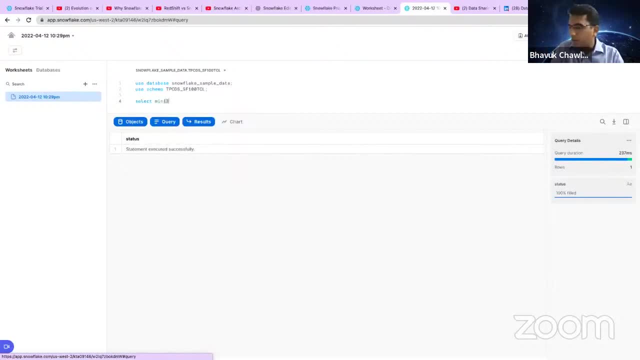 Like we are specifying the schema. and let's say I want to select minimum of a particular field, Let's say minimum value of shifted. I have select star from. let's say I pick up one table, So maybe I need to see which table I am having. 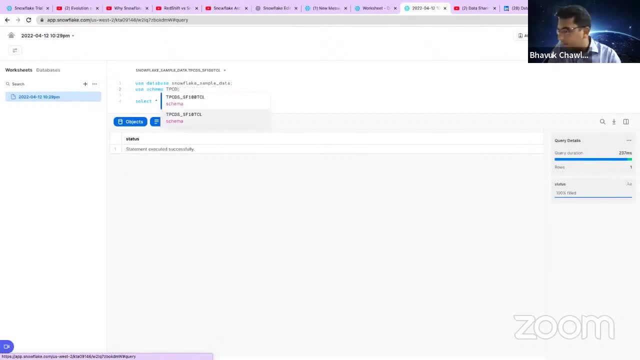 So this is SPDs, PPC, This is, let's say, TPC, CH, and then this is like SF, SF, 10.. So let's say I'm picking up this and I say: use this schema. And then after that I want to pick up a table. 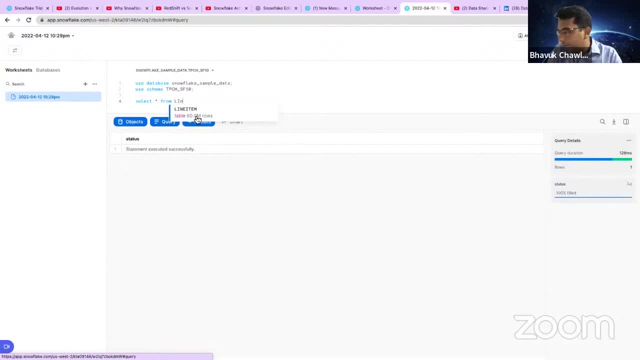 So this table can be like. let's say, I'm picking a table line item, This is having 60 million rows And I want to pick up- Let's say I never do star in a data warehouse. This is not a good pattern. 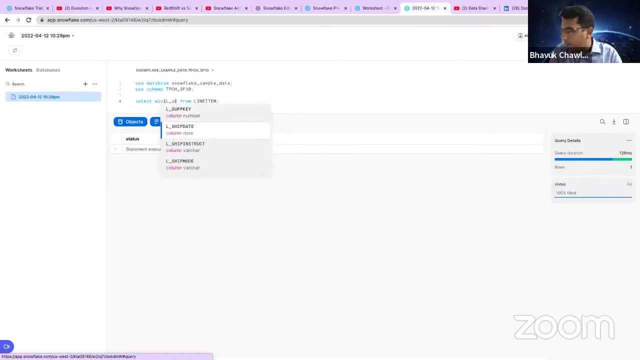 So I am specific to a particular field, So I want to find out minimum ship date. So this is a meta database query. When I run this query I am able to find out the minimum ship date and the runtime. It took like less than like around a hundred millisecond. 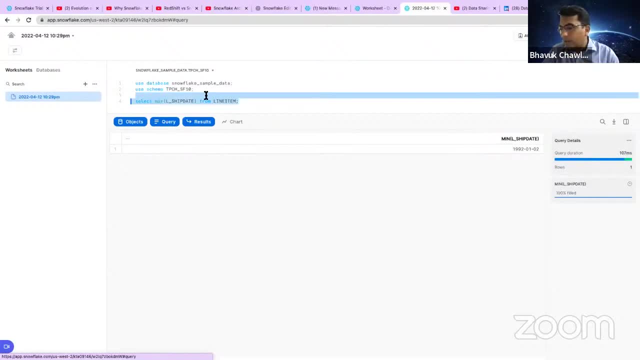 It took a hundred millisecond to retrieve the minimum date, And you can also find out other attributes, Um like, for example, you want to find out the max or min, or this metadata database query. So these are very, very So you will find I'm executing this query and there are so many versions created. you know, when you are working with Google doc, then you will see a lot of versions are getting created and you can go back in time. 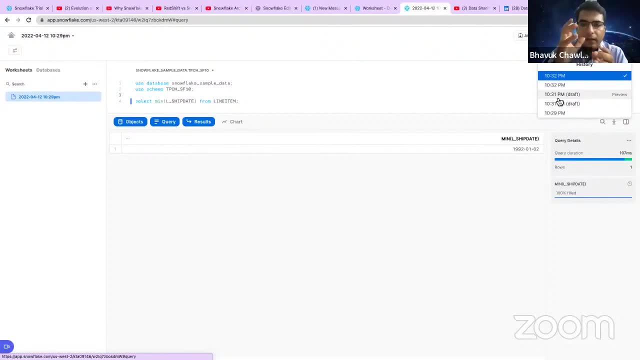 Same thing. So what is the difference? This is like crux of this webinar. What is the difference between snowflake and other data warehouses, traditional data warehouses, You know, one option is you send an email and share a word document. So that is like one way of data sharing. 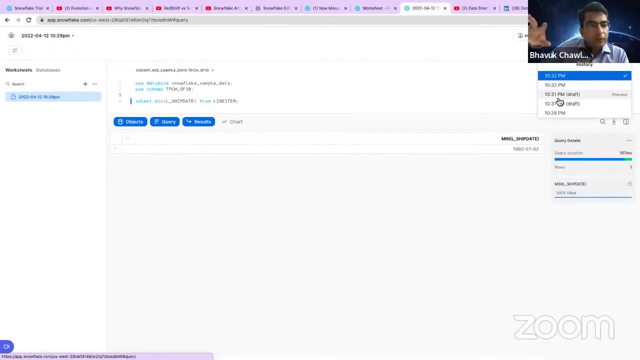 But when you are working in Google doc, then It's like storage on cloud and you can have infinite storage on Google doc. It's not limited. when you are sending an email and you're sending a word document, then it is limited by size of the attachment. 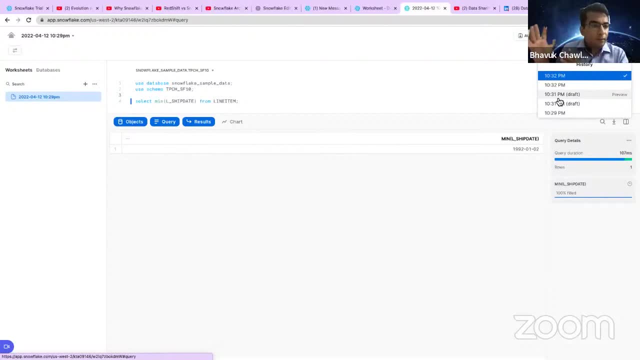 Right. But when you are working on Google drive, Google doc, then it's infinite storage. Second benefit is when you're working in Google doc you have versioning. So same thing you can say: we can go back. Let's say I want to go back to the initial version. 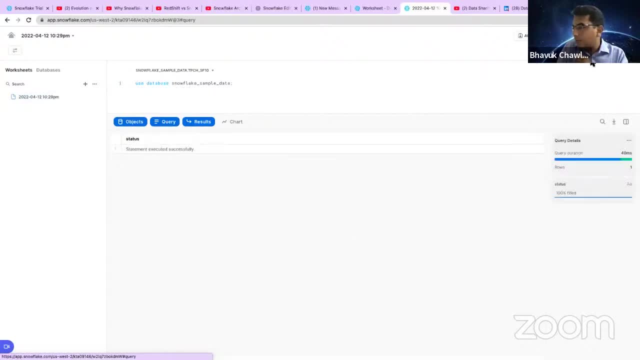 So can you see, now this is the initial version and I can switch back. Same thing, I can switch to the latest version. Yeah, So same thing: You can do time travel, You are able to do time travel and you are the owner of the data. 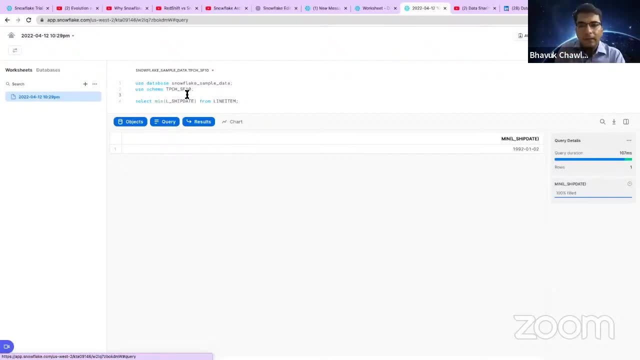 Like in Google doc, you are the owner of the data, but when you are sending an email, the owner is the one who is receiving that email, Right? So that is through uh like email you are sending the data to. you are losing the ownership. 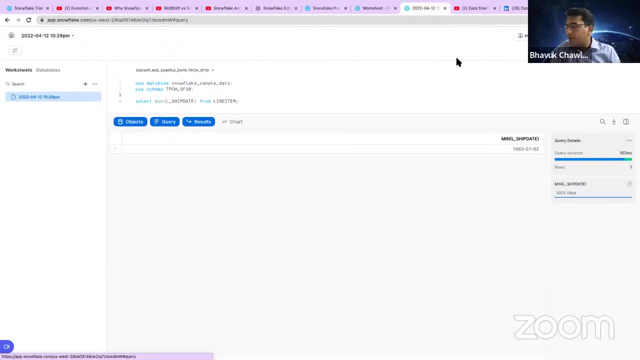 Yeah, So that's the same concept that I have covered here in my session related to the sharing, data sharing. So you can see, in this we have like hints coming where it will suggest the name of The table name, of the schema name of the database, and then you have metadata based queries. 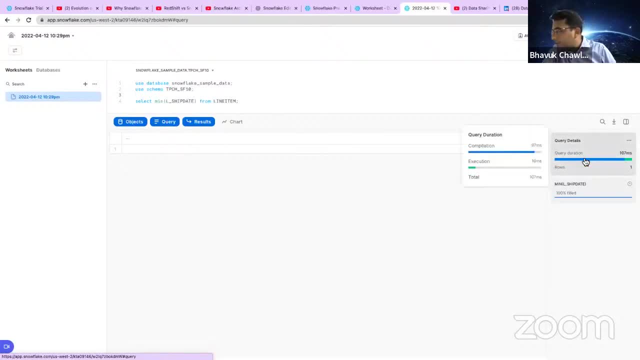 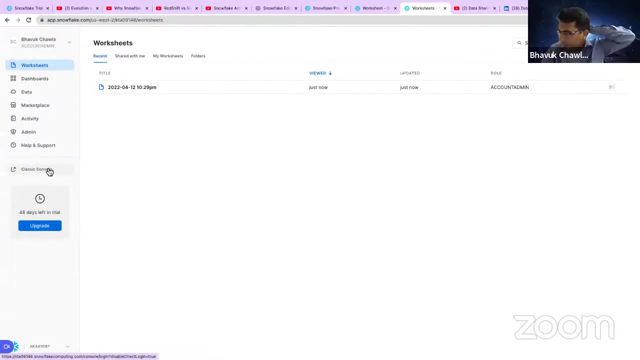 You can look at the query duration and you can see how much time it took to execute it. So even you can look at the query plan and other things. but I want to communicate. here is like a snowflake. Uh, this is new interface, but you you can switch back to classical console also and you can see what limitations we were having and the new interface is overcoming those limitations. 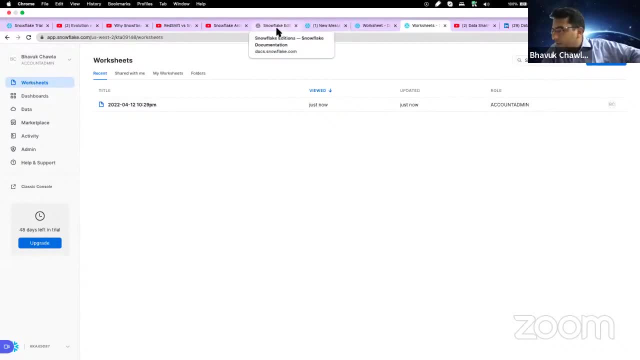 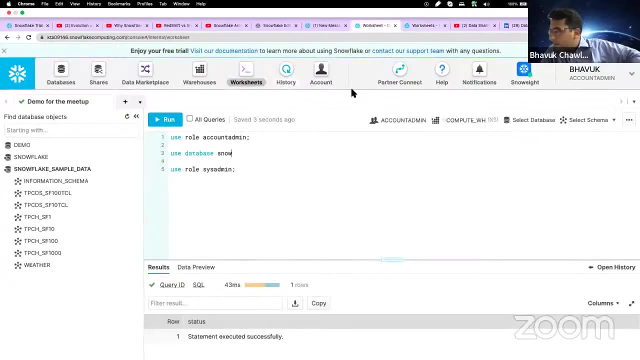 So let's say you want to work with data in snowflake, Yeah, And you are looking for telecom data, You are looking for medical data, You are looking for data specifically to your domain. So that is also possible. You can just go to um the data marketplace and you can bring data from here. 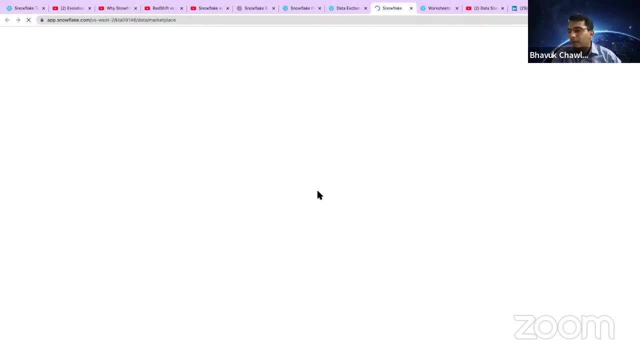 You can say, explore data marketplace, You just need to sign in and then you can uh, have a share. So you can have a share from that particular domain, Like you can have domain specific search. So I have explained all these things in a video, which is data sharing. 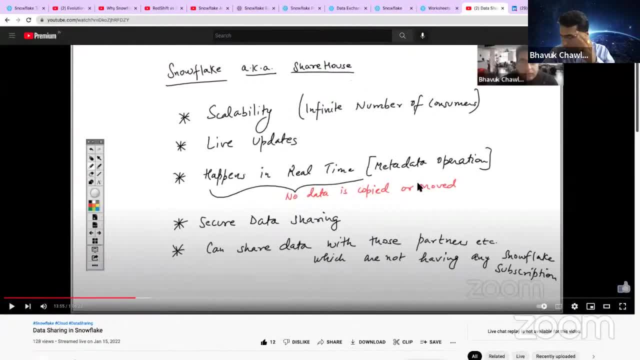 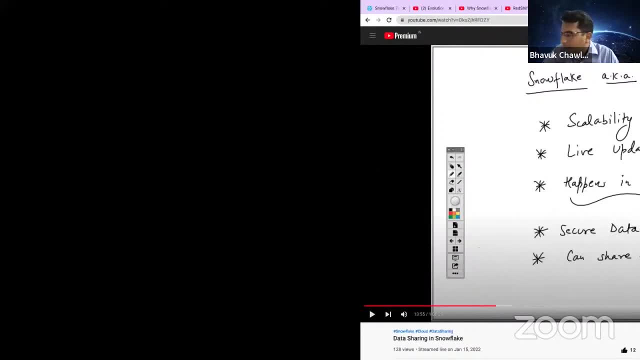 So I would encourage you to watch that Um video, where you will find interesting details. Yeah Around data sharing, Yeah. So, coming back to this, so we were. we started with snowflake basics, We started with snowflake architecture. 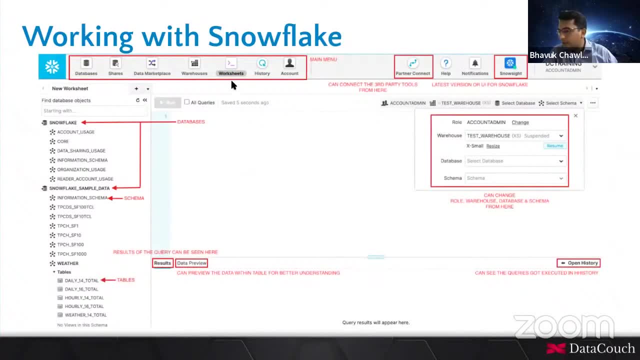 Um, and then how do we work with snowflakes? So there are like a lot of tabs in snowflake database tab. We have seen shares, We have seen data marketplace- I just talked about that- And then warehouses is basically for compute. 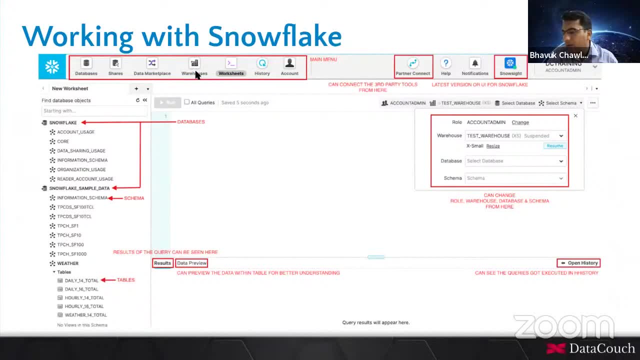 So I think um this webinar, we could not cover where Houses. this is like a very detailed topic. We I need to explain a lot of things. Maybe we can have a subsequent webinar where we can start from here only. 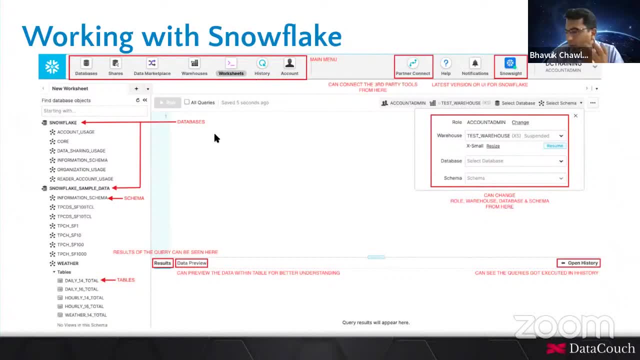 What are warehouses and, um, how do we work with warehouses? How do we fire queries? in more detail, So, since time is limited, so that's why I'm just um thinking like, uh, uh, maybe let's take up some questions from the chat. 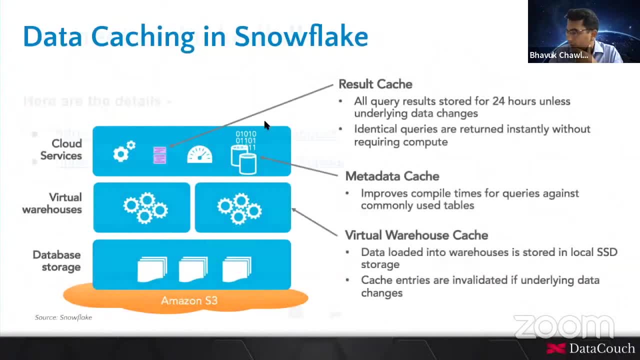 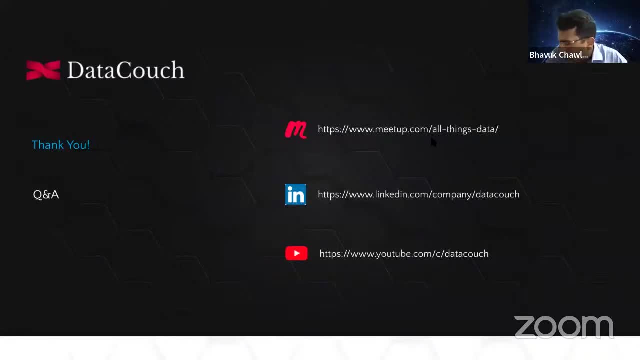 And also I would encourage you to please connect with me on uh LinkedIn. So this is my LinkedIn URL and um, there are links through which you can Join our meetup uh channel also, And then we have company page where you can find you can follow this company. 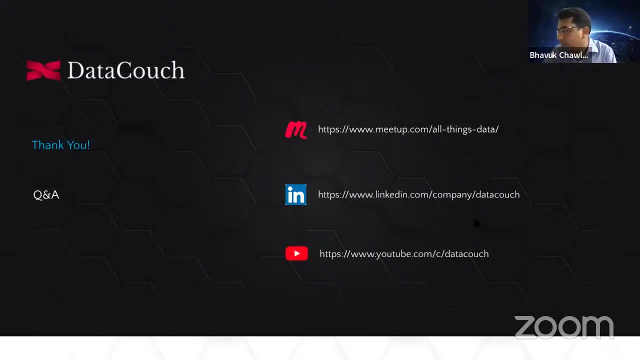 page where you will see a lot of interesting blogs and articles around snowflake and many other areas, And then we have a YouTube channel. So let me pick up a few questions. that okay, Nathan? I, if I can pick a few questions. yeah, let's just answer a few questions and then we'll. 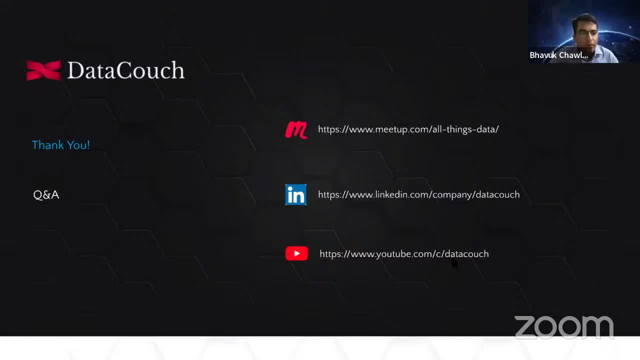 let everybody be on their way. Sure, sure, I'm going to talk about it, Thank you. Thank you, Nathan. Um, so now there is a question. Is it correct to say, okay, this is fine. So let me scroll down. 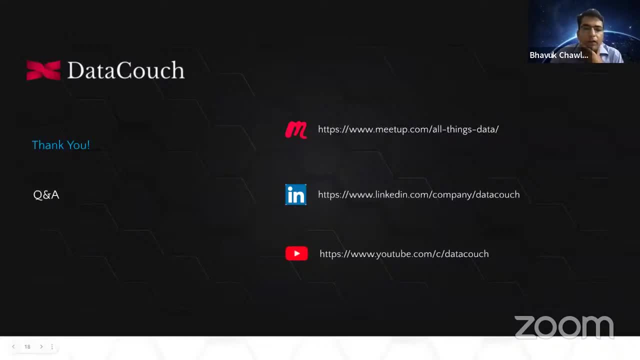 There are more questions: What is the difference between BigQuery and snowflake and how a snowflake is better? So you know, costing model is different and you need to see many, many things Like when we compare BigQuery versus snowflake. um, there are like the, the 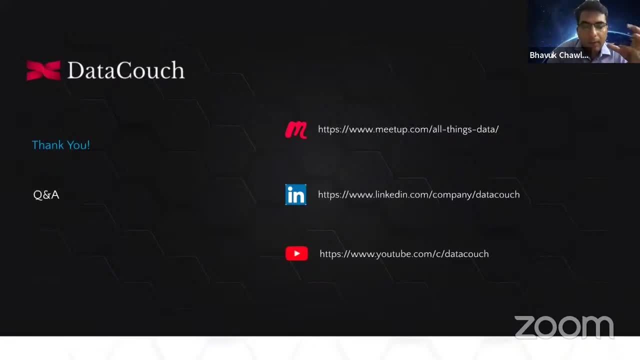 way it charges the BigQuery charges based on the amount of data that you process, Right, So you pay for that. but in snowflake you are charged for the um, the query runtime. So So the compa comparing which one is like? there are many things like: whenever you choose a data warehouse, you have to have um, a kind of metrics that you have to create. 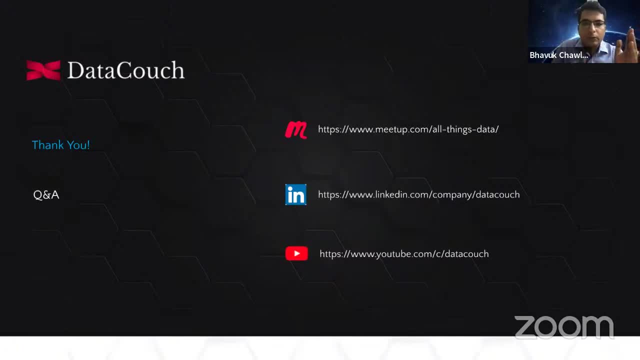 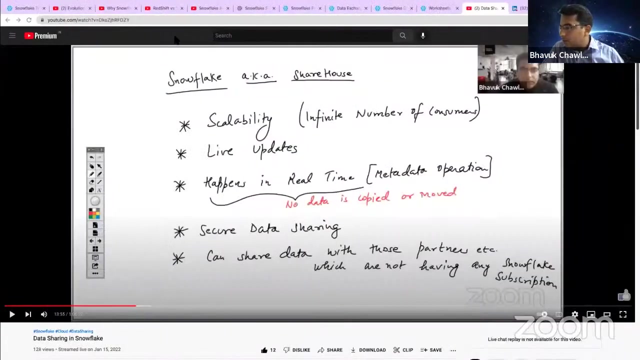 You have to write down the factors based on which you are choosing a particular data warehouse. So it's not like very straightforward to say that this data warehouse is good or this data warehouse is good, So you have to write down the security requirements. So when I come, when I talk about security, so you need to go to which edition of snowflake. 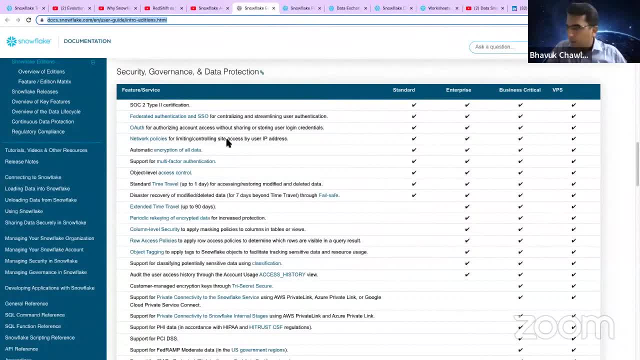 You need to Be very specific. which edition of snowflake we are talking about, which security features you are talking about, right? Um, so one thing is costing, Another thing is security, Another thing is performance. So you have to have all the functional, non-functional requirement. 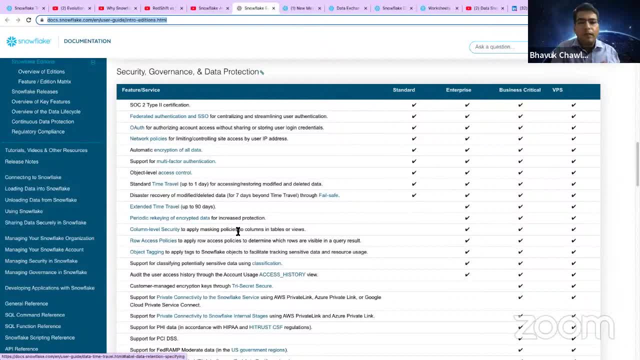 Do you have a lot of semi-structured data, Like what is the native support? Like what is your primary cloud provider? What is your cloud strategy? You have to write down all these requirements and then you can compare. but BigQuery is offering what snowflake is offering. 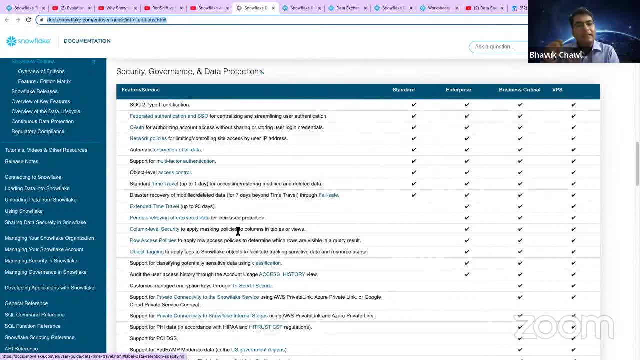 And if you are comparing signups or any other Data warehouse, you have to write down all this thing and then you can say, okay, this one works well for my use case, for my requirements based on functional and non-functional things and compliance, governance, and everything will come into picture overall how it integrates with your partner ecosystem tools that you are having in your org right. 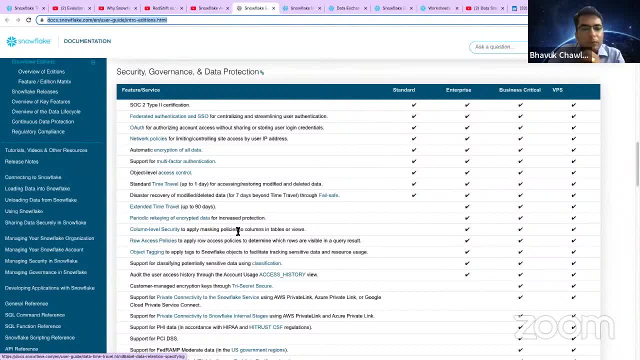 So multiple factors will come into picture. Yeah, So case sensitive thing. Um, if you create a database- let's say I'm creating a database with lowercase or uppercase- it will always, let's say, you can quickly see the demo. Also, if I just 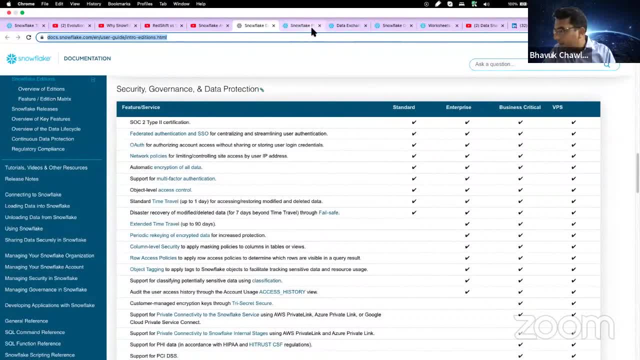 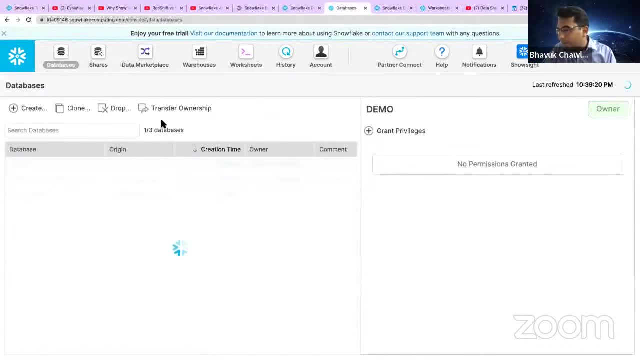 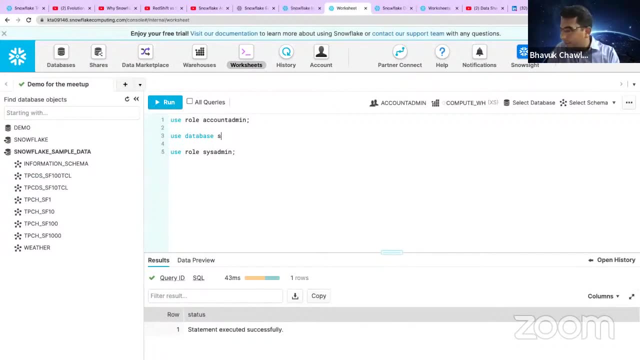 Uh, go to snowflake again. And uh, if you go to the snowflake platform, uh, sorry, I'm here. So if you just be so it will not matter, like if you should do that. So if you are in worksheet and you are saying, let's say, if you write, let's say, database I'm using demo is lowercase or you write uppercase. 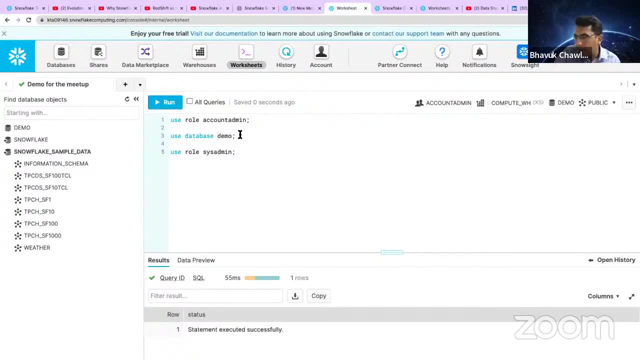 No problem, It will be able to select. It is not like having any problem with this. Yeah, So uppercase or lowercase, it's fine. Um, specifically, This is identifiers that we are talking about. uh, what happens to my data when registration ends and I stop paying? 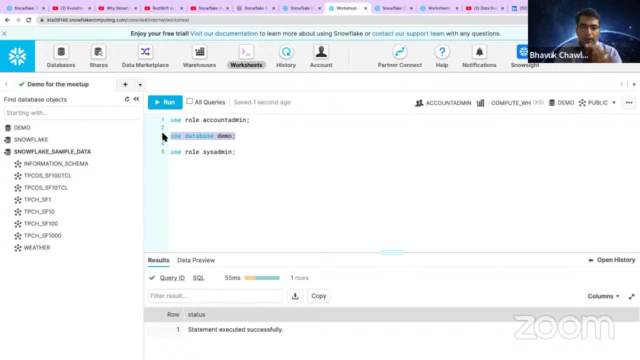 Okay, No problem. So there is a state in which account goes into inactive state. So that's a good question. Um, so, uh, when you log into snowflake, then there is a check which is made like: uh, if your account is inactive state or inactive state. 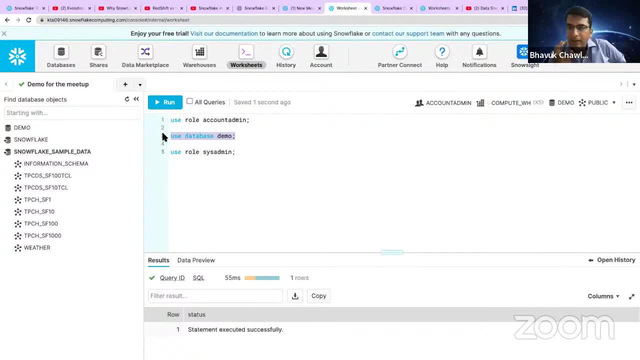 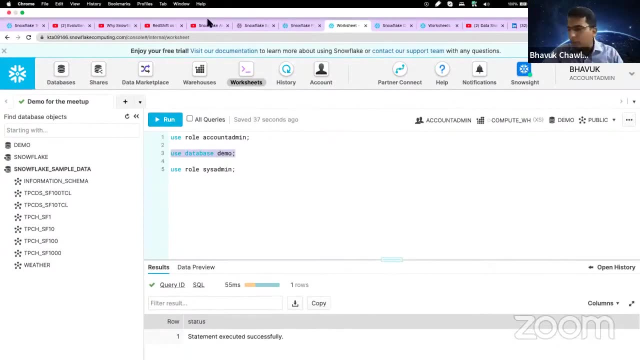 So, if you're not paying, and then, um, there are many things like which model you have chosen, like uh are you paying for? let's say you have uh super, So that's a good question. Um, so, uh, I think it's very, very first thing, before I answer this question, it is very important to understand the pricing model. 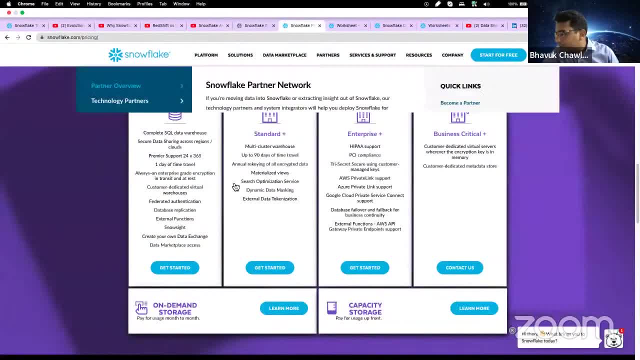 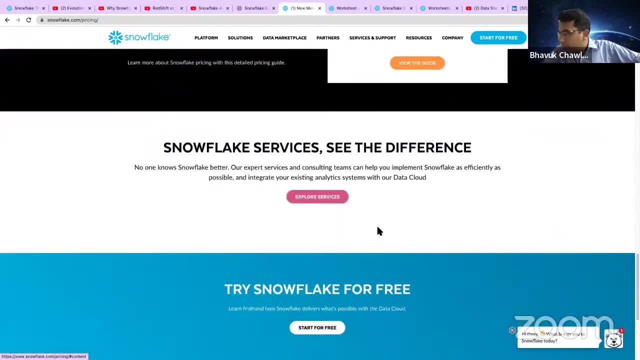 So how the pricing works in snowflake. So this is a pricing guide that we are having on snowflake. So are you going for um, something which is like on demand storage, or you are going for capacity storage? how the pricing works. 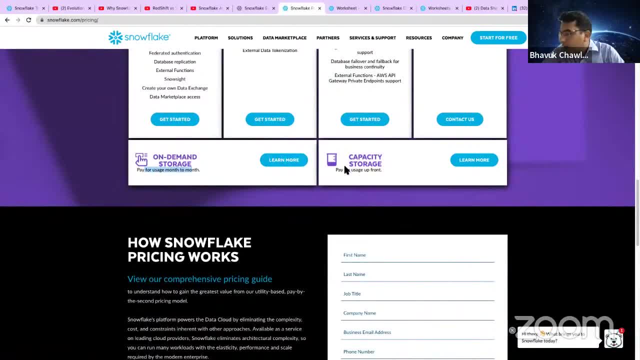 Right, And you can also see, uh like: uh, do you, do you want to pay for usage month to month or do you want to pay usage upfront? So which pricing model you are choosing? Right, you can, you can have so like. your account may be in an active state, that is, another state of. 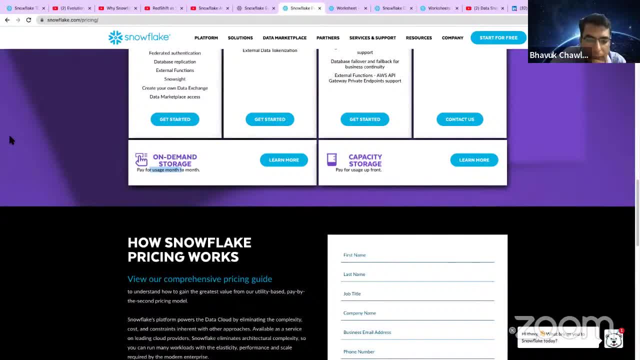 account and when you log into snowflake, then it is all. these checks are made. can you alter, modify, insert, delete the table? yes, it is possible. would it be time travel to show data before? yes, so time travel, you can do that in snowflake. yeah, so you can insert, but if you perform single, single row. 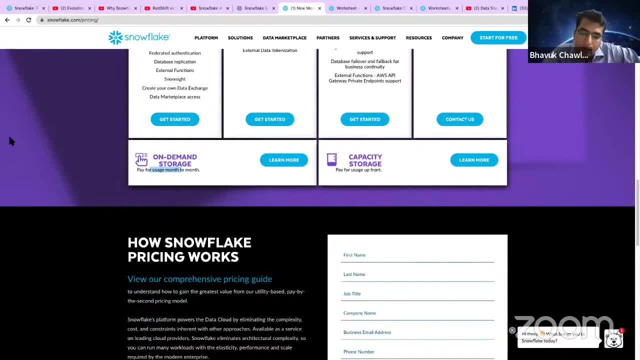 operations in snowflake, then it will be very, very slow because it is an olap. it's not designed for that specifically. it's a columnar storage. yeah, so the purpose is different here. okay, any other question? can you give outline on migration of legacy? so, yes, so here, if you go to community, 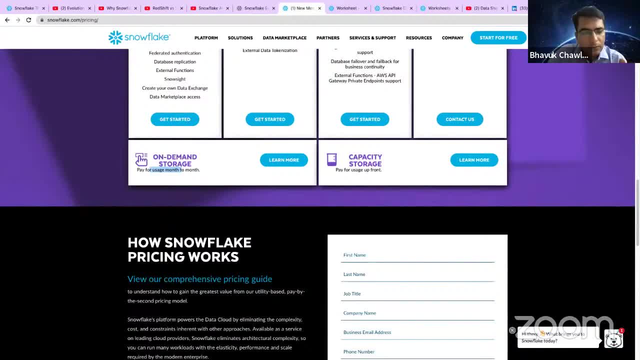 you will find like: can you tell me like which specific data warehouse you are targeting to migrate into snowflake? jenny, if you can share, you can send me questions over linkedin. i can answer that and then i can share more details about specific data warehouse that you are planning to migrate. yeah so, thank you so much for attending the session. 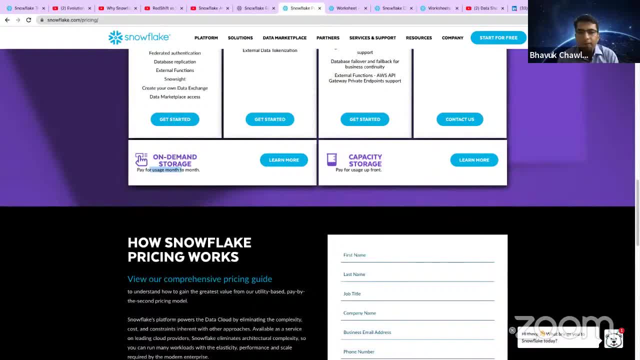 uh, it was my pleasure and honor to have you all nathan over to you. yeah, thank you, pavuk, i think. i mean, with the number of questions we saw, i think everybody really enjoyed, enjoyed your session. so thank you for for being here with us and everyone, thank you for sticking around. i know we went a bit.